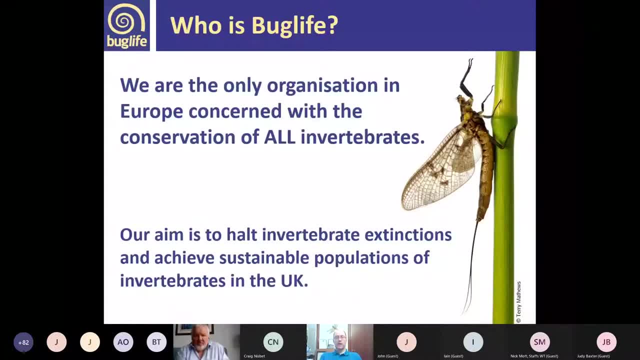 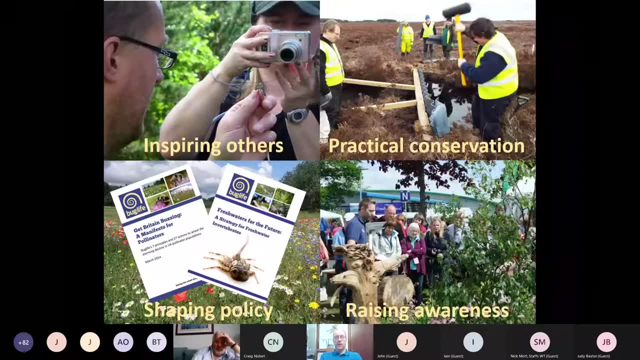 to millipedes, spiders, to starfish- you name it. we cover it Anything without a backbone. And we do this in four main ways. We inspire others. we go out there, we show people invertebrates. we get them up close to invertebrates and show them what makes them tick. We shape policy. 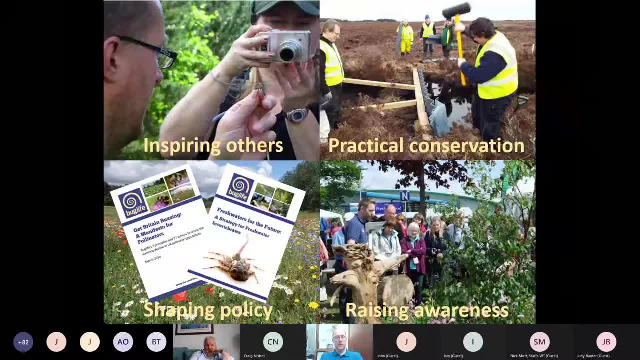 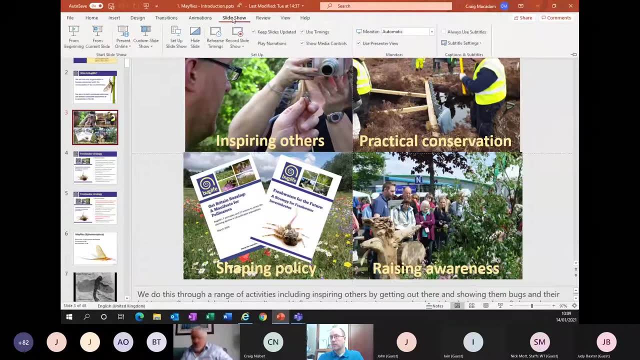 we influence decision makers to make the right choices for invertebrates, to benefit them and their habitats. We undertake practical conservation efforts. So then like this: sorry, I've seen the timing on here, Hold on, I'm just going to start that without timing again. 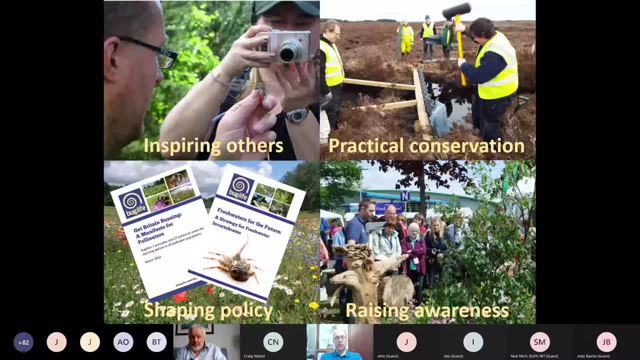 Yeah, so we undertake practical conservation efforts, which, in this case, in the top left, top right, there is a bog restoration project that we've been running in Falkirk and North Lanarkshire- And we raise awareness. we go out there and we talk to people and we tell them all about invertebrates and the issues affecting them. 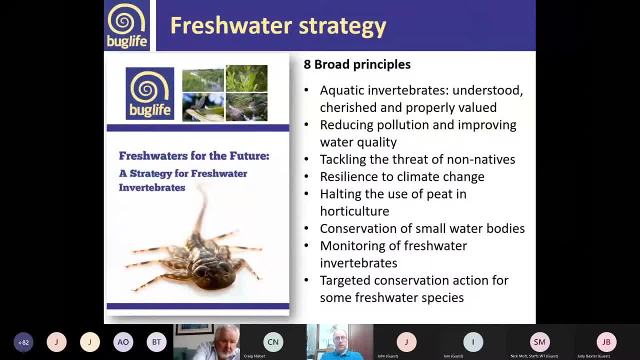 So this particular workshop feeds into our freshwater strategy- We published this last year or the year before- which has eight main broad principles, and the two that this one feeds into is understanding, cherishing and properly valuing aquatic invertebrates and monitoring our freshwater invertebrates. 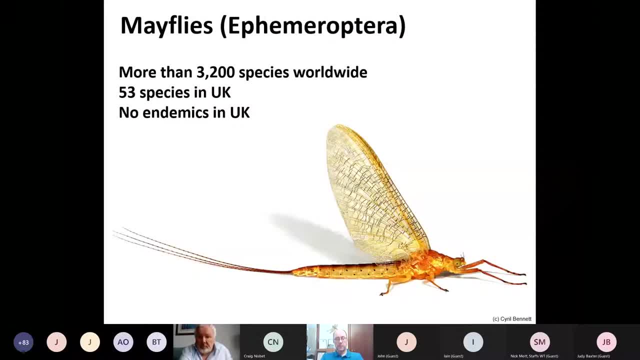 Today I'm going to talk to you about mayflies. I'm going to do this presentation in three parts: one in the forest and the other in reco vam sun. I'm going to do this in a typical setting and I'm going to show you how I do it. So back in the beginning, where I was, this is a nice accident site with water. Use a device, a persuadet putty only, and Powell and other different types of water once a year go into the water. you have to do things that Lando's going to make mentioned before. there's a three-part department. 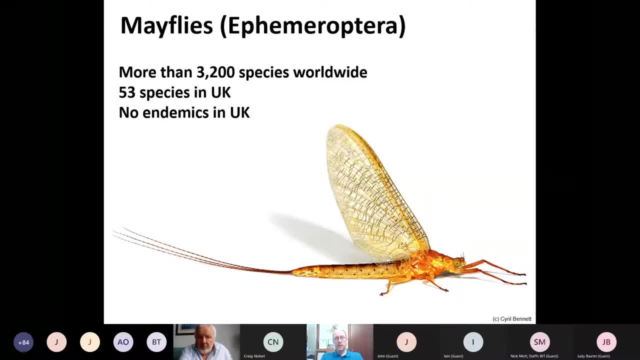 three parts and at the end of each part I'm going to allow a little bit of time for us to go through some of the questions in the chat. So the first part is going to be about just a general introduction to mayflies, Then I'm going to talk about the identification of mayfly larvae and then the last. 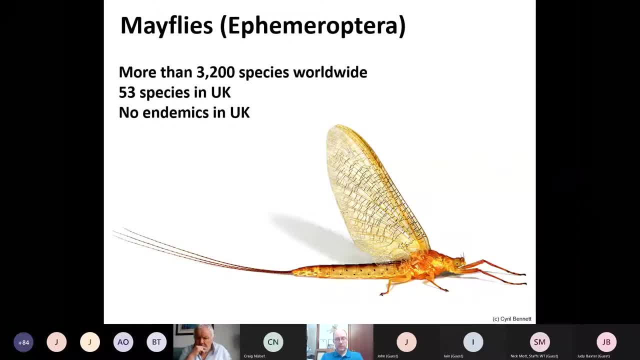 part is going to be about recording river flies, so recording mayflies, stoneflies and caddisflies. So mayflies are a fairly small order of insects. There's around about 3,200 species worldwide. there's a few new ones described every year and in the UK we've got 53 species and for those of 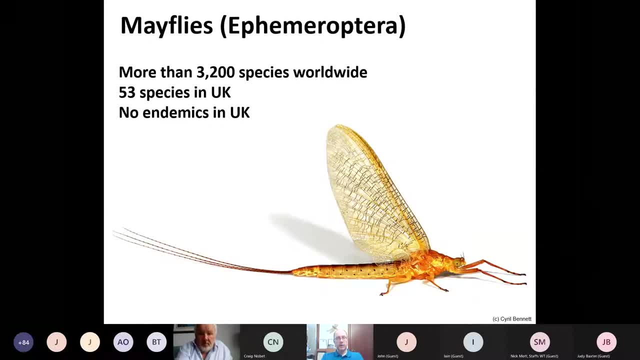 you that know your mayflies will know that for many, many years there was only 51 species. but in the last two years we've actually discovered two new species and I'll come on to that later on. There are no endemic mayflies in the UK. In other groups we have some endemic species. 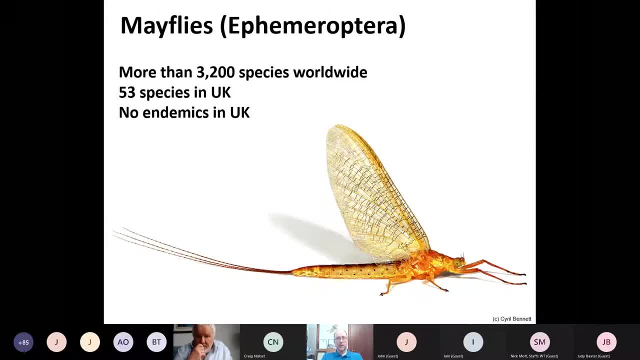 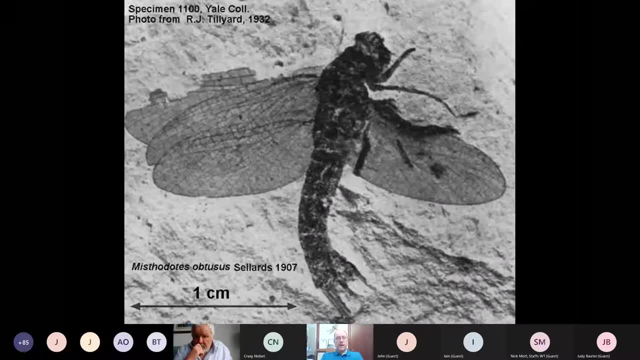 some species that are only found in the UK, but in the mayflies they're all European species that have found their way here. Mayflies have a really ancient history. They're one of the oldest winged insects that we know. This is Msthodotes obtusus, which is a fossil from around about 280 to 290 million years ago. 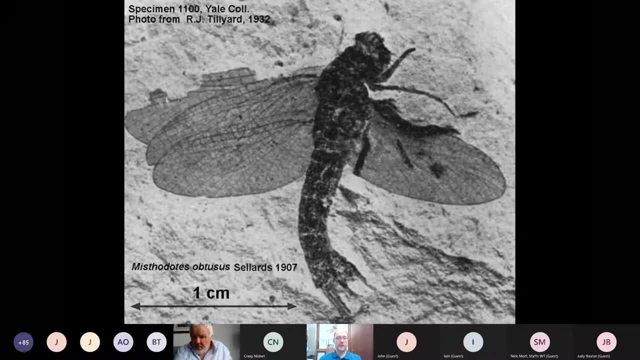 which was found in fossil beds in Kansas and you can see. if you look at that, you can see it looks very similar to a dragonfly. actually, It's got long, large wings. both sets of wings are large, and the difference is that it's got these tails at the end here, and so this is 290 million. 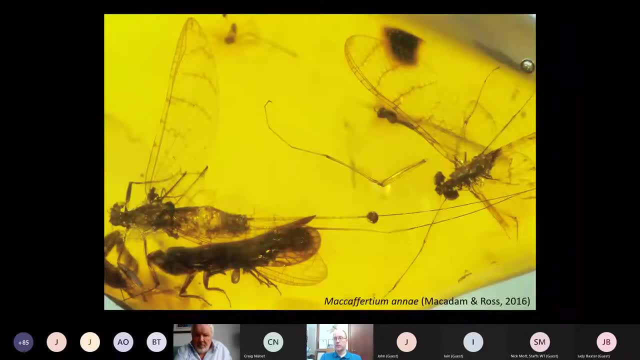 years ago and if we come a little bit closer to present time, this is a piece of amber from Mexico from about 15 to 20 million years ago and this is a species of mayfly here which you can see. it looks a lot more like a modern mayfly. It's got the large forewings. 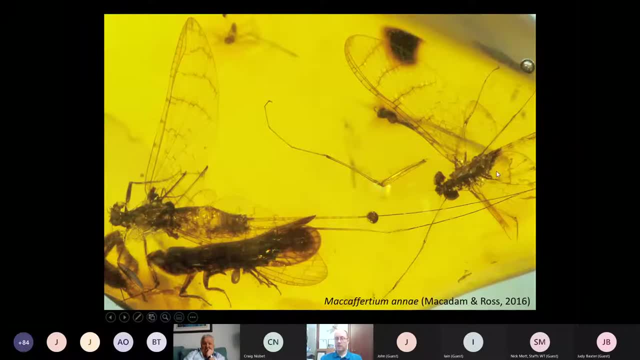 and smaller hind wings here. This is actually a piece with a female here and a male here, and this is a full-grid bug that's in the foreground there and amber's amazing substance, because these insects have landed on a piece of resin on a tree that's solidified within a minute and they're preserved perfectly. 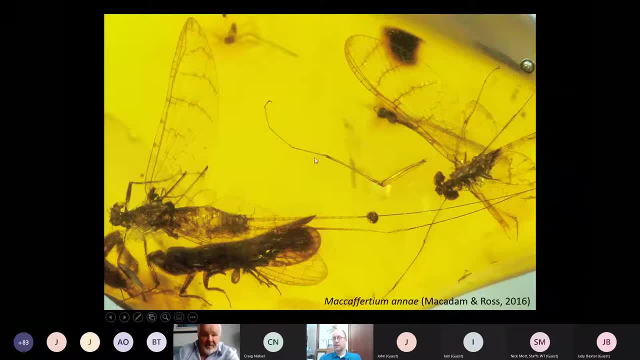 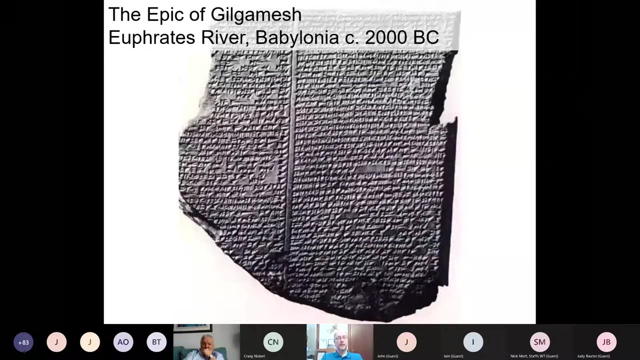 You can see all the features you can see on this, this detached leg here, just all the features that you need to to identify or to describe this species. The written history of mayflies is long as well. It goes back to around about 2000 BC and this which is thought to. 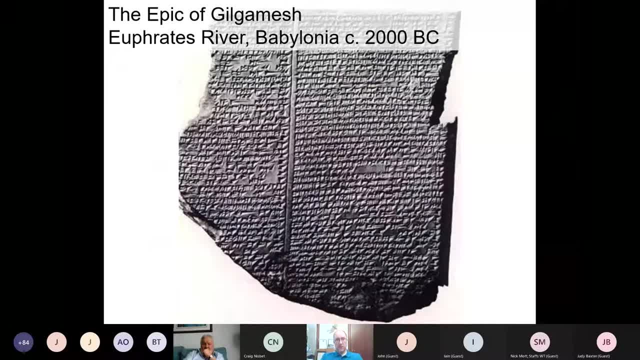 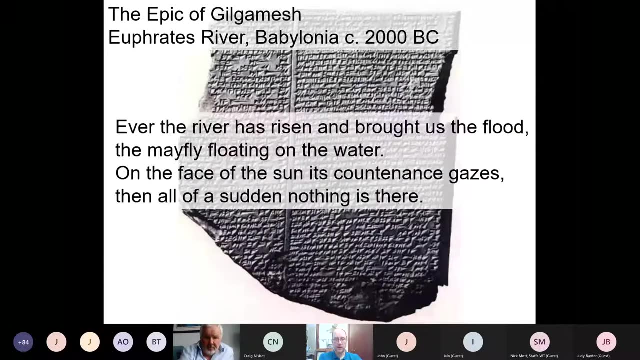 be the first written text, the Epic of Gilgamesh, which describes a great ruler in ancient Babylonia and he thinks he's immortal, and he thinks that he'll live forever, and they liken him to a mayfly and that, and with this quote here, which is ever, the river has risen and brought us the flood, the. 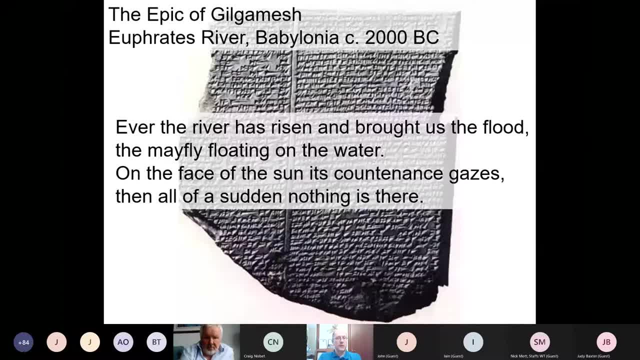 mayfly, floating on the water, on the face of the sun. it's counting its gazes, then, all of a sudden, nothing is there. So it's talking about the, the brevity of life. it's talking about the brevity of the mayfly's life and the fact that it lives for a day and then it's gone. Craig, Yeah, Craig, sorry, I'm just interrupting all the time. 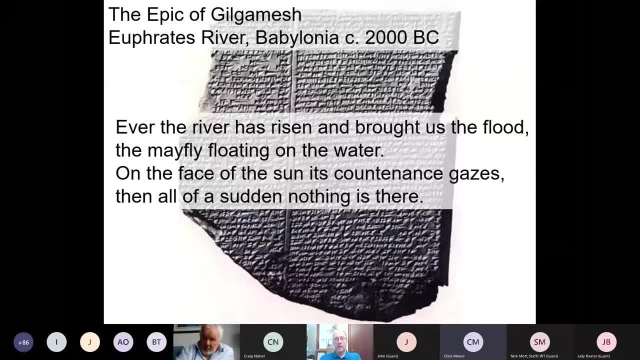 behalf of quite a number of the audience. there's some comments and hands raised that the the presentation you're going through isn't on the screen. Oh, okay, It is actually being shared. I think the what what I was just typing is I'm recommending that people. 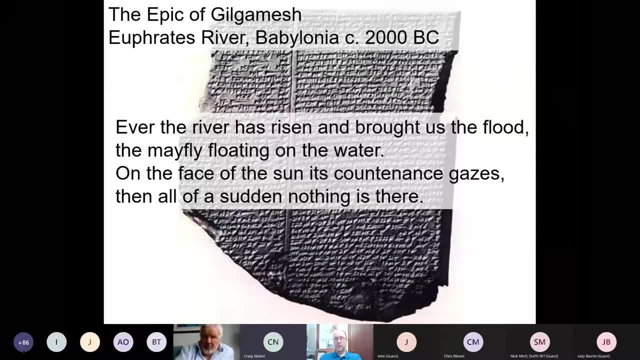 log off and then rejoin the meeting. Shall we start again then? I mean, we've not, we're only a couple of minutes into this, so shall we start again? try and get this to everybody see it. Well, I, I know that many people, many people can see it. it seems to be a a divide between 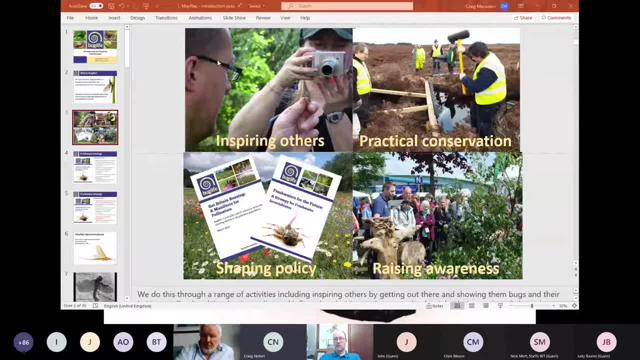 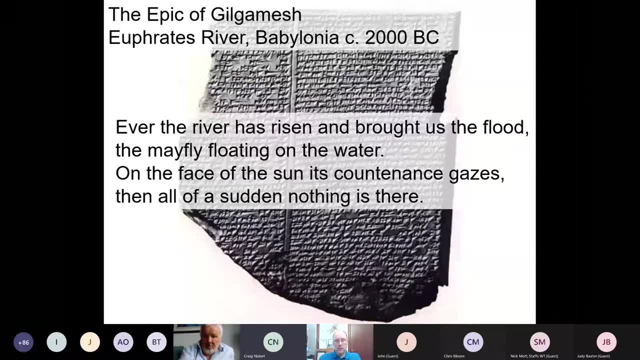 the I. I don't know how many people can't, and there's certainly a few, but I'm getting. well, I mean we're getting it. we're getting messages coming through saying I can see it, I can see it, and so I will stop sharing. I would, I would recommend that anybody that hasn't been able to see the 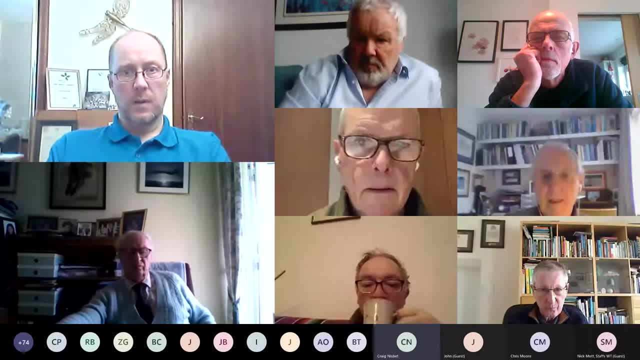 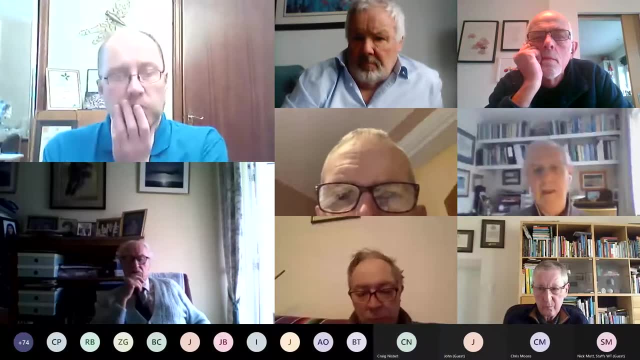 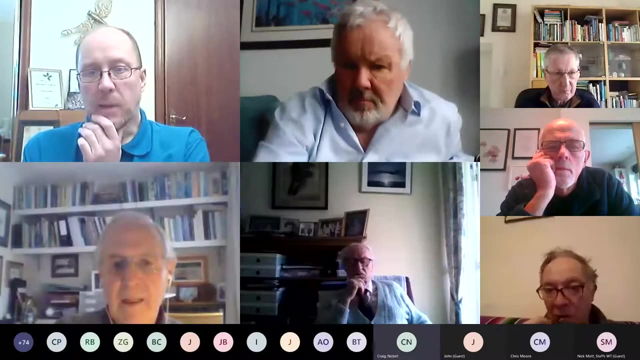 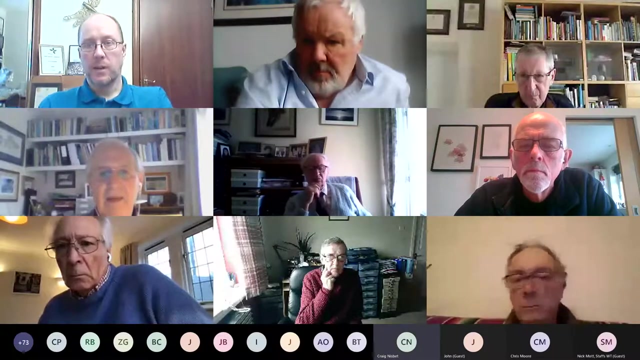 screen that Craig was sharing there, logs out, logs out of the meeting and tries to rejoin because the screen was being shared. so it was. it was visible for many of us. I can't see the comments when I'm presenting, so okay, so leaving and joining has worked for people. Yeah, Sandra said leaving and rejoining has worked. 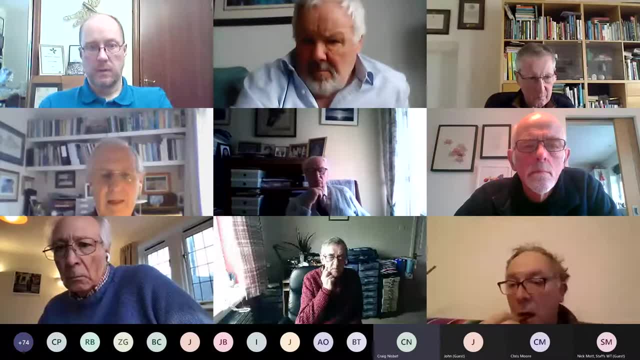 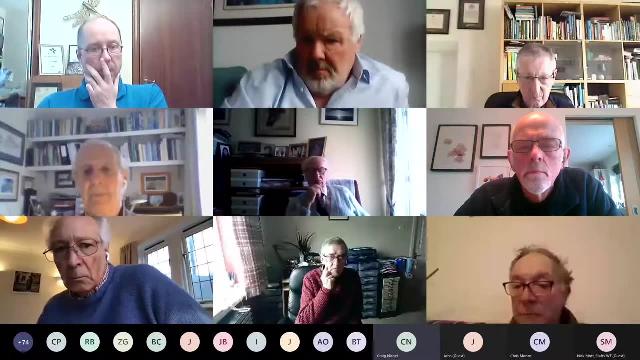 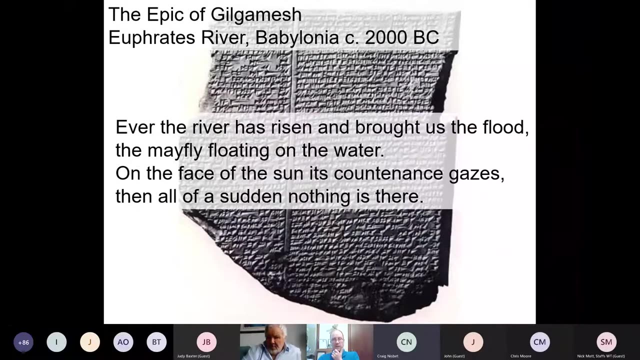 for her. so if anybody does have the problem that they can't see the screen, then I would recommend just leaving the meeting and then rejoining. Hopefully that will solve your issue. Okay, so can people see it. Sorry for the interruption, Craig. No, that's fine. can people see it now? Yes, that's, that's being shared. I need to find my notes now. 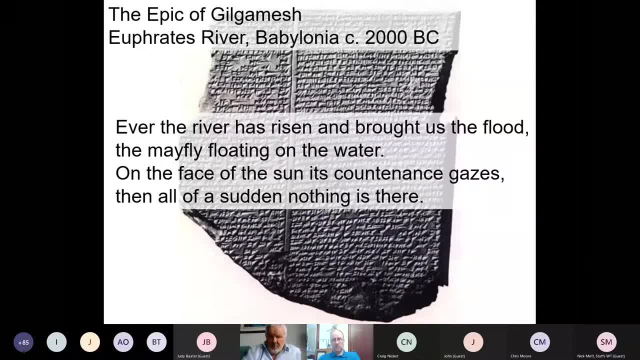 there we go, okay, and I've got, oh okay, I've got, oh okay, um, right, so, uh, yes, so the epic of Gilgamesh is the first, uh thought to be the first, text with a reference to mayfly in it. If we fast forward, uh what? nearly four thousand years and we actually 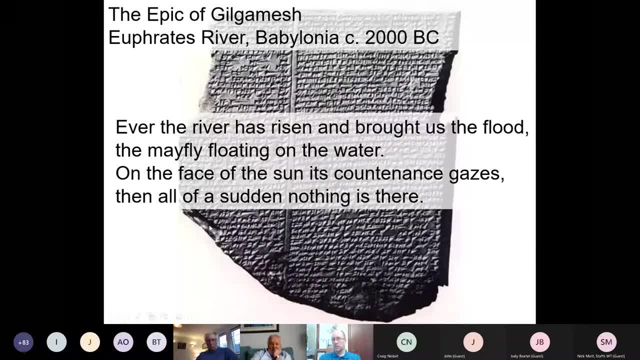 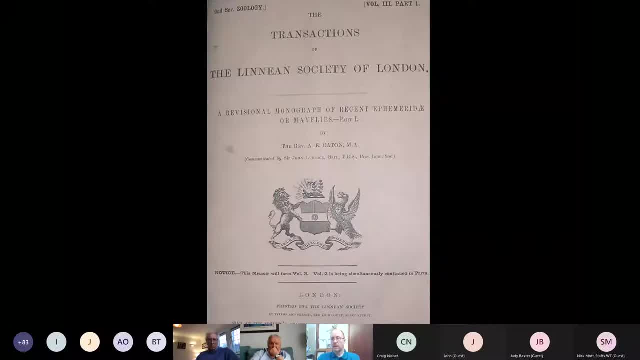 find the first scientific text with- uh, I'm not moving around. yeah, we find the first scientific text that names all uh ephemeroptera as mayflies. This is, this is the um, uh, a monograph that was written by, uh a minister from Cornwall and from Somerset, sorry, uh the. 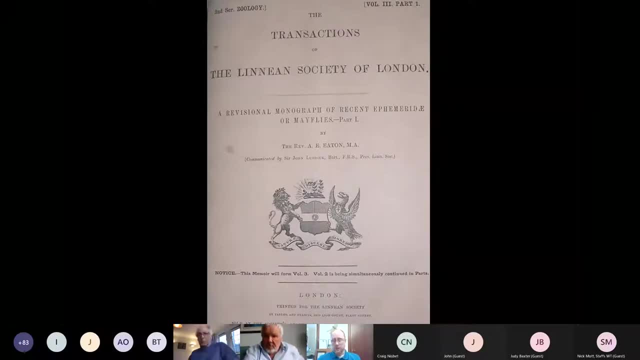 Reverend Eaton. He is sort of the grandfather of mayfly research. he at the time, in 1883, he described every known species of mayfly and he called them mayflies, and up to then they'd been called ephemeroptera, uh, ephemerons, ephemeridae, um. but he was the first person to coin the the phrase. 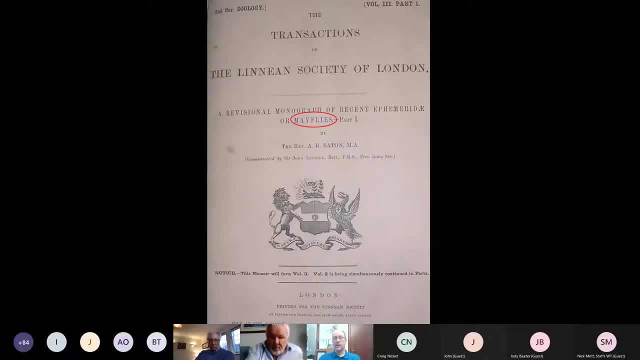 mayflies for them and uh, the this this book is still used. I've got a copy here and I use it fairly regularly to check descriptions of of species. it is a monumental piece of work. um, the, the descriptions of mayflies. this, this is a a scientific description, but before, before Eaton. 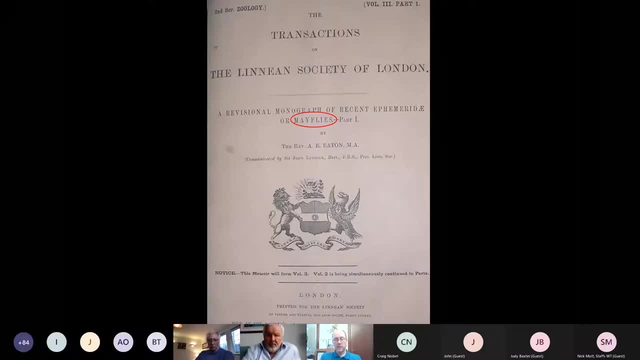 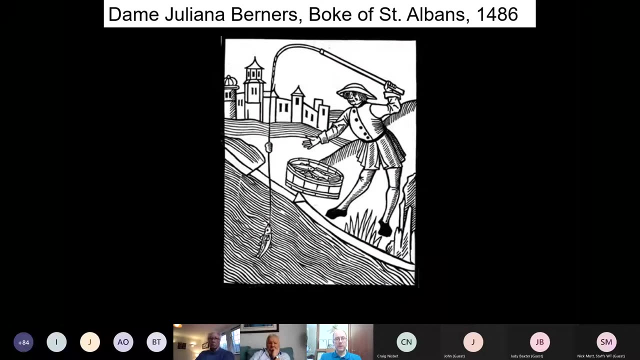 um, there were, there were descriptions of mayflies, and they were mostly from people who were um interested in angling, and one particular book which has some very detailed descriptions is this one. here is the book of St Alwyn's, which was uh created by a clergy person, Dame Juliana Berners. 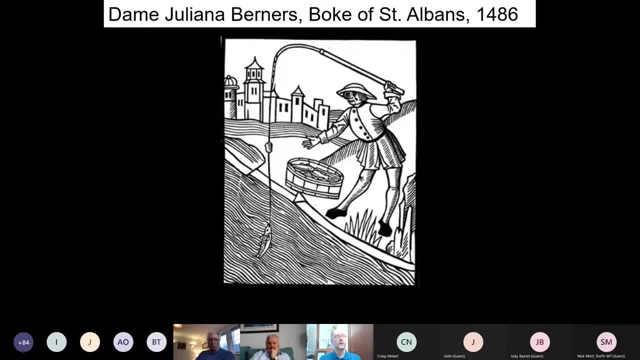 who was the abbotess of? uh well, which abbot uh abbey she was with? but um, sorry um, and this was in 1486, and she made quite detailed descriptions of how you fish um, so she had a treatise of fishing with an angle um, so the first one of the first uh uh mentions of angling um, and she described the 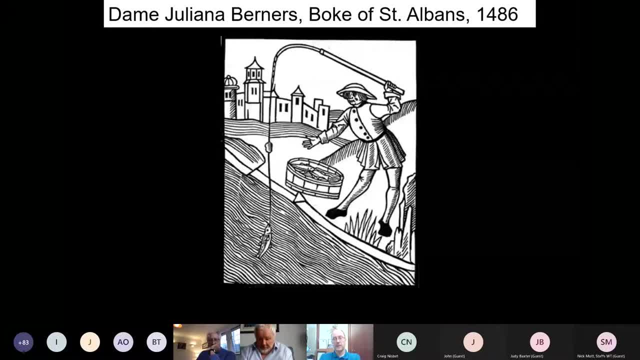 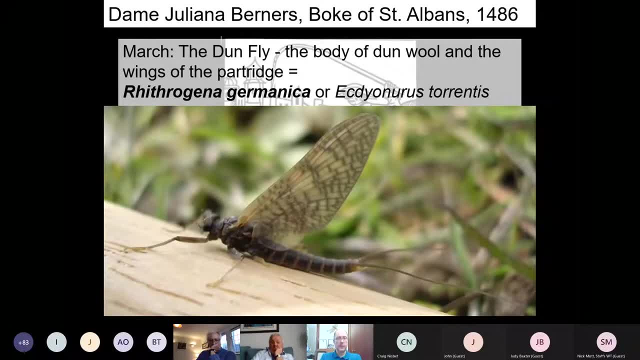 tackle. she described the methods, but she also described the flies that you should use and she she gave patterns for, for mimicking them. so this one here, the the dun fly, was the body of dun wool and the wings of the partridge, and that's believed to be either Rithuagina, germanica. 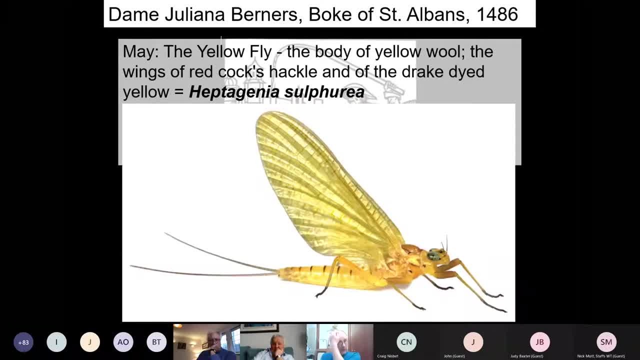 or Ecteoneris tarentis. she described the yellow fly for may um the body of yellow wool, the wings of red cock hackle and the and of the drake dyed yellow, and you can see here this is Heptagenia sulphurea, which we now call the yellow may dun um it. 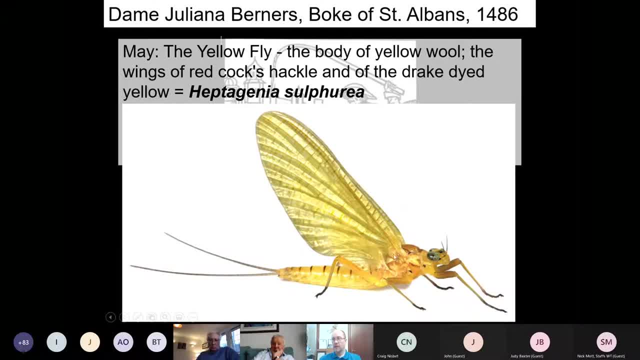 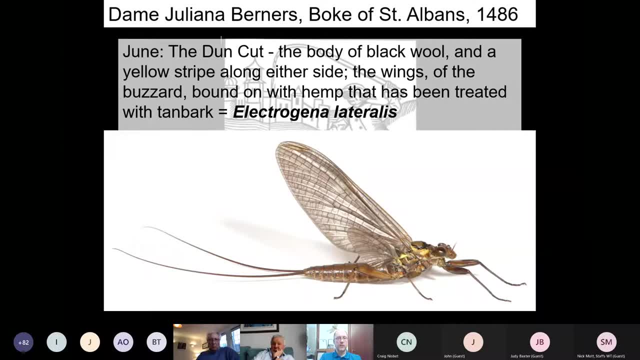 emerges in May and it's got this uh reddish colouring round about the base of these uh yellow wings and yellow body. and then she called the, the, the. in June the dun cut the body of black wool, a yellow stripe along either side, the wings of the buzzard bound on with hemp. that's been. 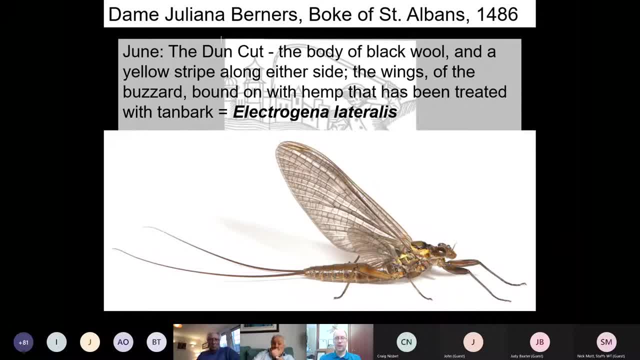 created- and this is a really good description of uh electrogenolateralis with this, this uh yellow stripe down the side, underneath the wings here, and we still call it the dusky yellow streak now. okay, so that that's um kind of the history of of mayflies as a thing. let's have a look at the life. 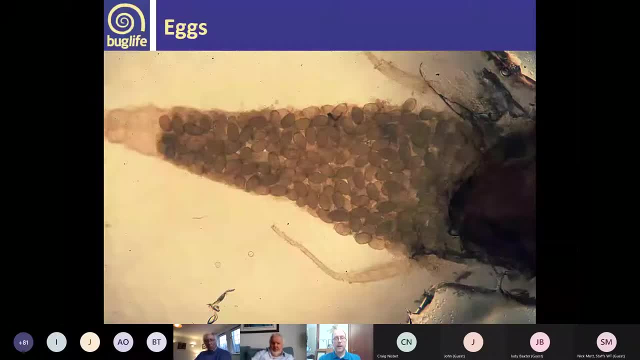 history now, um, they start off as an egg, um, and the, the female insect is, is simply an egg carrier. it it eggs to the river for laying, And you can see this image here of a small canis adult with the abdomen actually packed full of eggs. And mayflies can lay anything between 2,000. 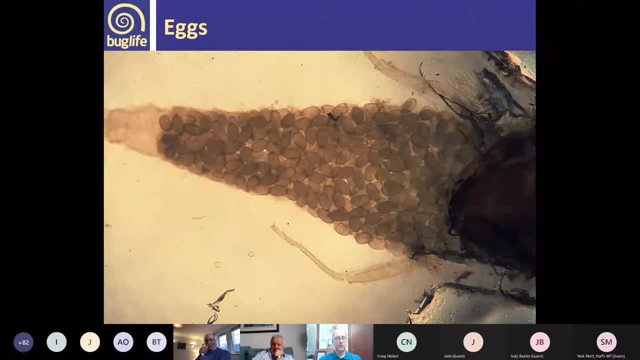 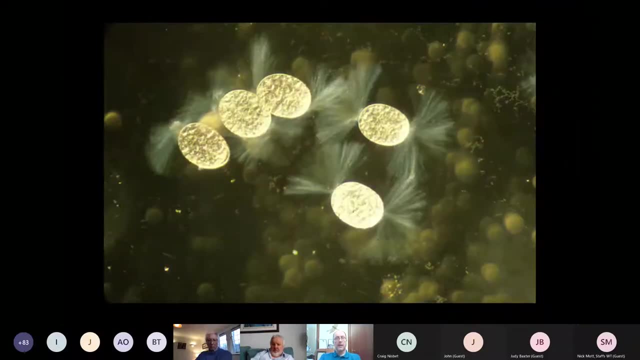 to 8,000 eggs the species in the UK. So they're basically just egg factories, if you like. for females, The eggs- when they hit the water they need to prevent them from washing away, So they have a form of sticky attachment structures. In many species this is just the sticky surface. 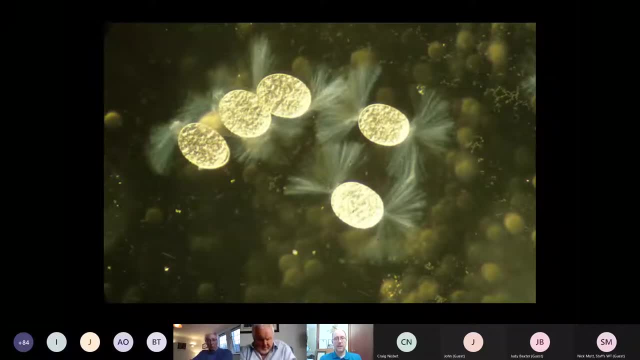 of the eggs themselves, But in others, as these ones here, they're very distinctive and they can even be used to identify the species to the species level. These fine hairs on the side of the eggs spring out on contact with water and enable the stick the egg to. 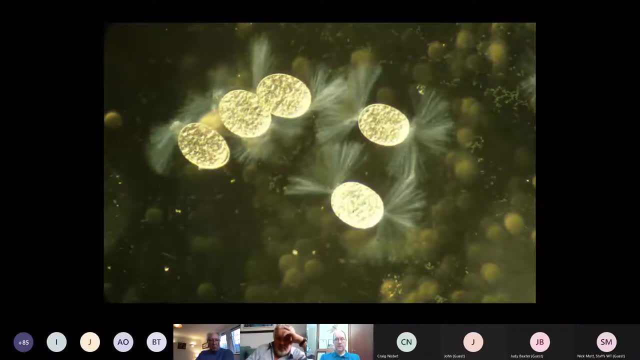 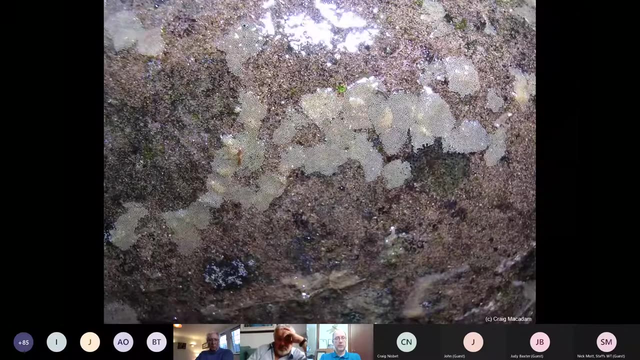 stick to plants and gravel and the bed, et cetera. Some species go a step further and they actually crawl under the water to lay their eggs directly onto stones to prevent them from washing away. And this is a Betis rodani egg patch here. 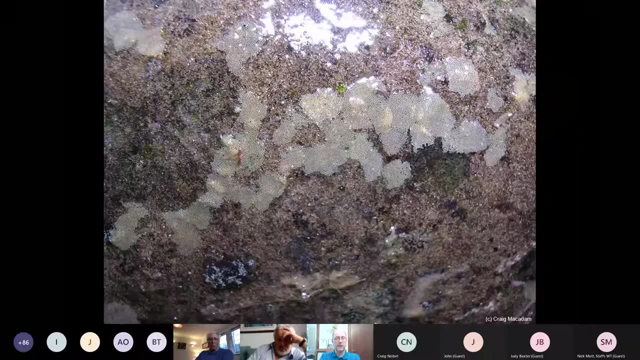 You can see, all these little tiny patches are actually patches of eggs that a female has laid on an exposed stone. She's landed on an exposed stone in the river, crawled under the water surface and then laid the eggs directly, And you can see that each patch 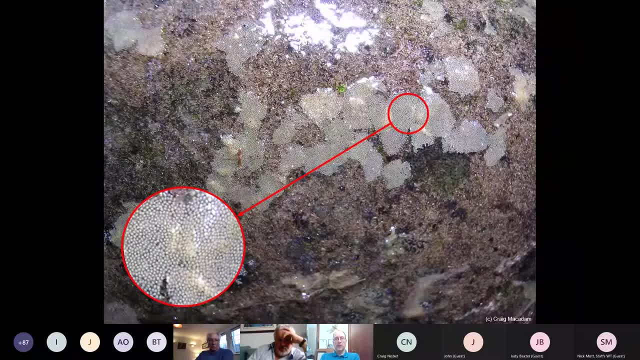 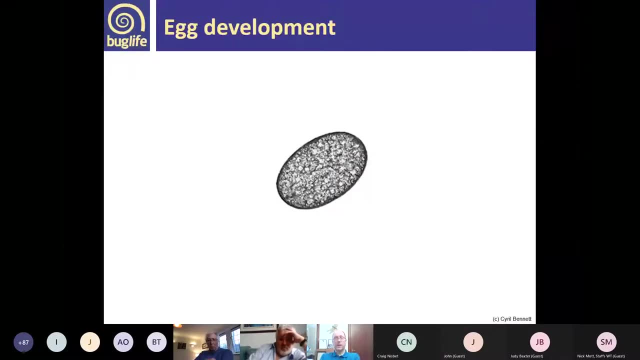 has hundreds upon hundreds of eggs in them. The egg develops through time and is linked with temperature. It starts off as a fairly featureless object. You can then through time. you can see it change inside. You can see the larvae developing. you just about see. 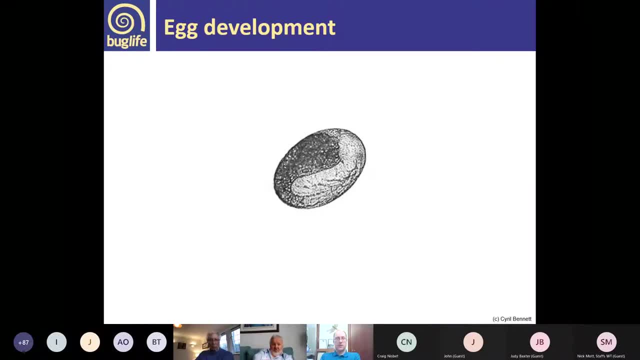 the shape moving there. You can start to see the body segments in the bottom of this image. here You see the eye spots now And then you see it'll hatch out, And when it hatches out it looks a little like a silverfish. The things to note are that in this case there are no gills down. 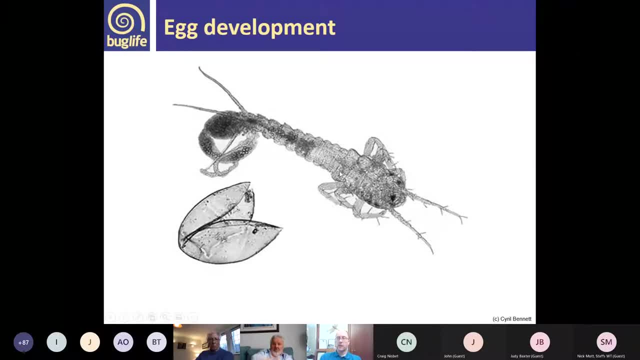 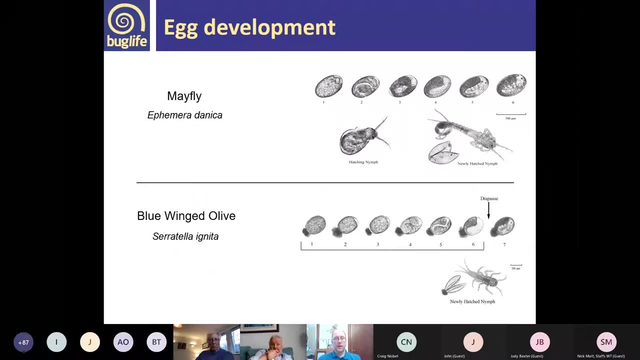 the side of the body when in this first instar larvae, Different species go through different egg development stages. So in that one that I've just shown you, which was ephemera danica, the egg is laid and the egg starts developing straight away, and it develops all the way through and hatches. 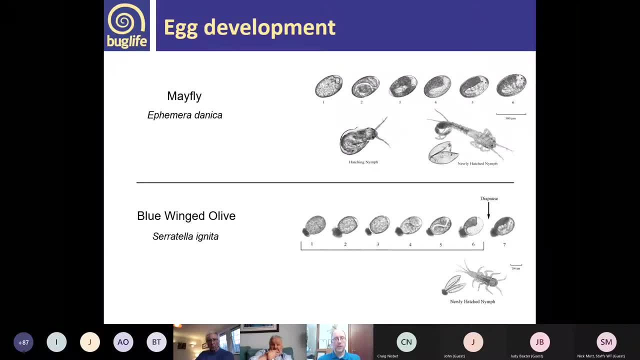 without stopping The one on the bottom. here is the blue winged olive, serratella ignita. And this does the same thing: It develops all the way through, and then it stops, and it stops just before the winter in this case. So it'll lay its eggs in between July and 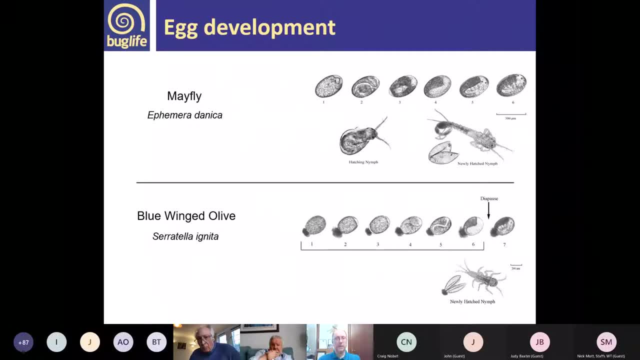 September, It'll develop fairly quickly And then it goes into this thing called diapause, And this is- this is a effectively a suspended animation stage where it stops all development. It stops. It stops any development at all And it waits, And in this case it waits over. 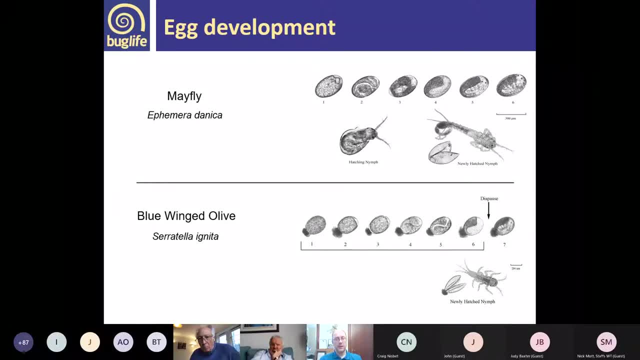 the winter and then its development is then triggered again when the water temperature rises in the spring. And so this is, this is just basically a method for it to avoid any, any harm during the winter. You can see on the image here. you can see. 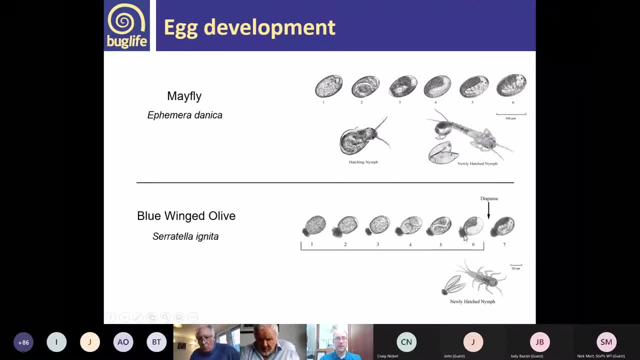 the attachment feature on this one. So these eggs are stuck to the bed, developing away and then waiting for the warmer weather in the winter, in the summer, in the spring, sorry to to allow it to hatch. Interestingly, some, some populations of this species have 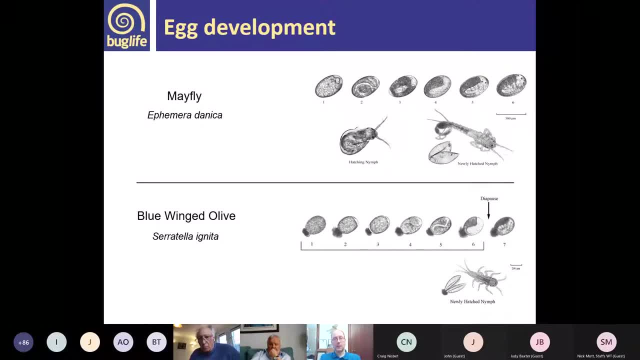 foregone the diapause and will develop all the way through, particularly in warmer temperatures. So And we're starting to see that in the chalk streams of the south of England, where we're getting populations of serotella ignita going right the way through without diapause And 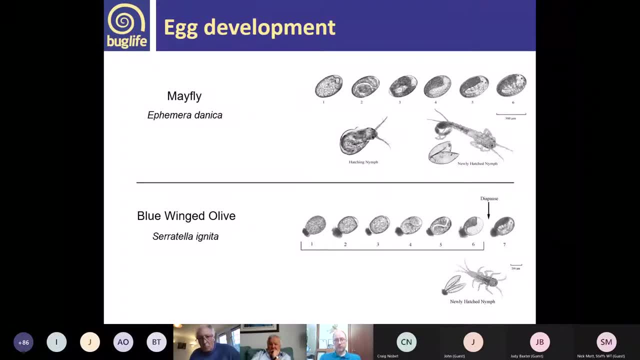 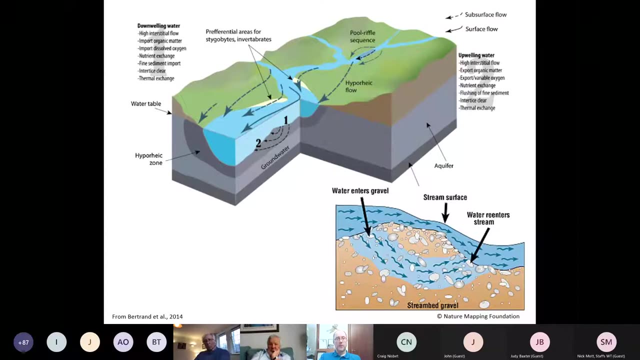 that is almost certainly a response to climate change. When they've hatched out, that little nymph that I showed you there is pretty vulnerable to being mashed about and or taken by other insects. So what they do is they? They go down into the gravels, And when we think of a river, we think of that meandering. 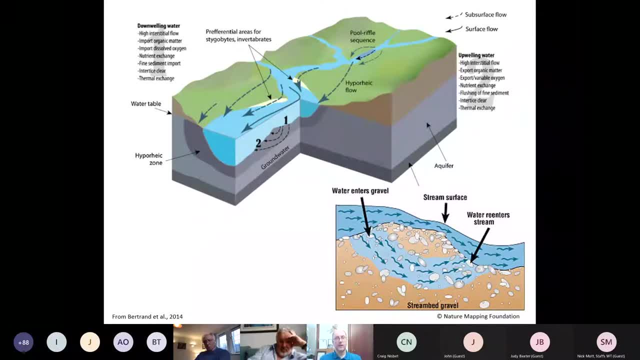 stream on the surface of the land, But actually the river is much bigger than that. It's got a large area called the Hyperia area, which is the. the water is where water is underneath the river, in the surrounding land and in the surrounding gravels, And on this image here. 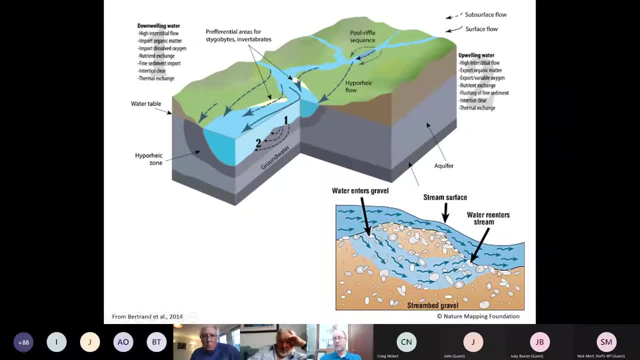 you can see how the water enters gravel and and will appear elsewhere, And it's in this sort of flow. here You'll find a lot of those small first instar larvae. We did some sampling where we put in tubes and sucked out the water from this area about a metre down, And you know you. 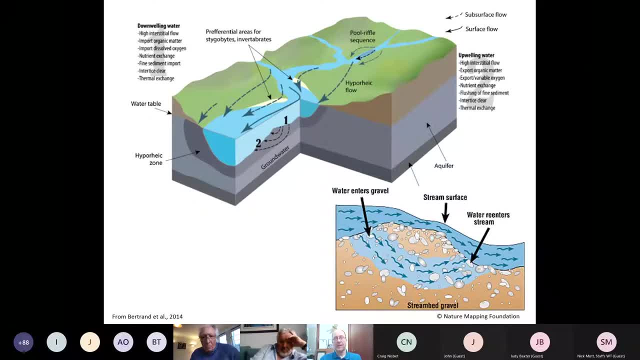 think you've got nothing. And then we start looking under the microscope. You've got all the tiny, tiny mayfly and stonefly larvae, And if you put them in a tube you think there's nothing in there, but you shake it and you get this sort of like snow globe effect with 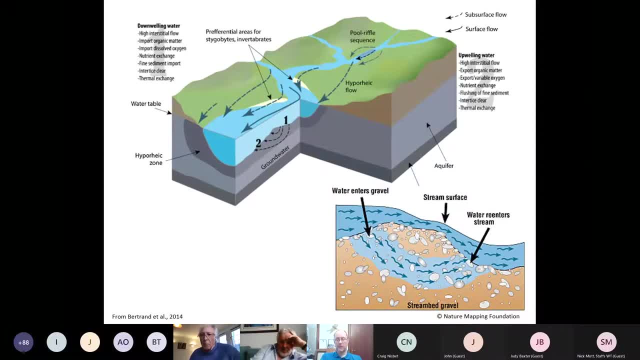 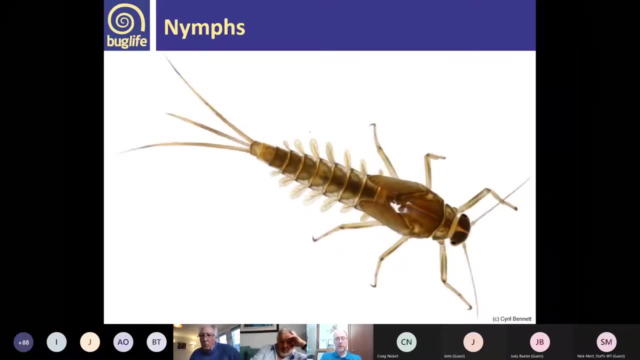 all these tiny, hundreds upon hundreds of these tiny larvae. Yeah, Now this, this, this slide is titled Nymphs. I've not changed this And so, just before we go any further, nymphs and larvae are kind of the same thing And the accepted term now. 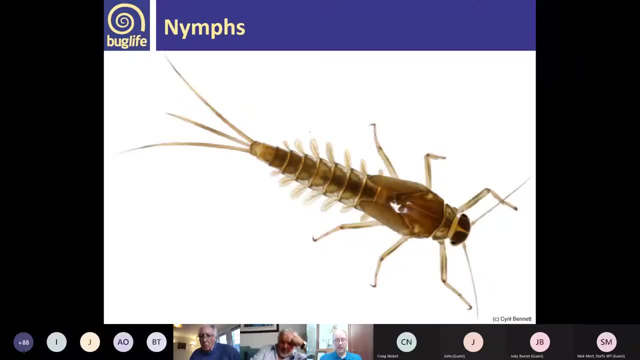 is larvae for all aquatic insect, juvenile aquatic insects, But I still lapse into saying nymphs every so often. Nymphs used to be the the term that was used for things that didn't go through full metamorphosis, So things like mayflies and stoneflies, whereas caddisflies, which do go through metamorphosis. 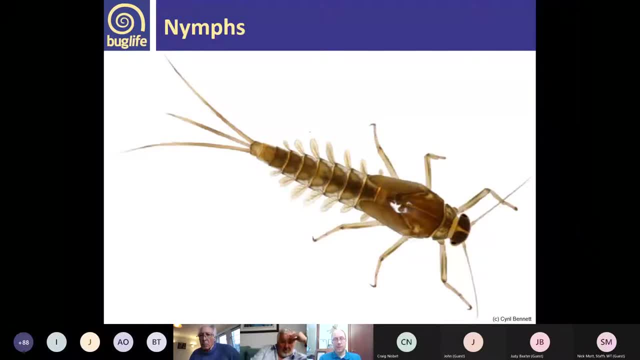 full metamorphosis, were larvae, And now we just call them all larvae- although I've not changed this slide- And the larvae come in various shapes and sizes, but they all have a. there's probably two main body plans, if you like. There's the streamlined cylindrical. 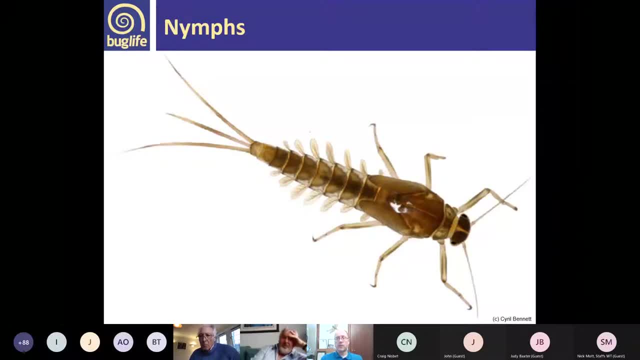 shape like this here, with the three tails Here and external gills down the side. You see the antennae are quite long, Yeah, and the the three pairs of legs, as you would on all insects. You actually see here the developing wing pads as well, So this is a fairly mature. 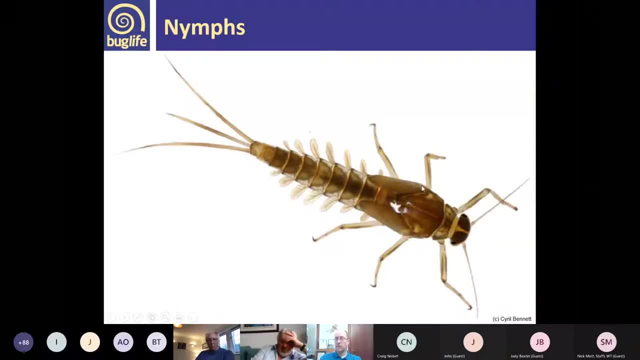 larvae The wing pads are. This is this is holding the wings in here And as the wings are bent, this is the wing pad. I can see that there's the wing pad here. This is the they mature, these grow and they darken. So, once these went, if these were to go black, 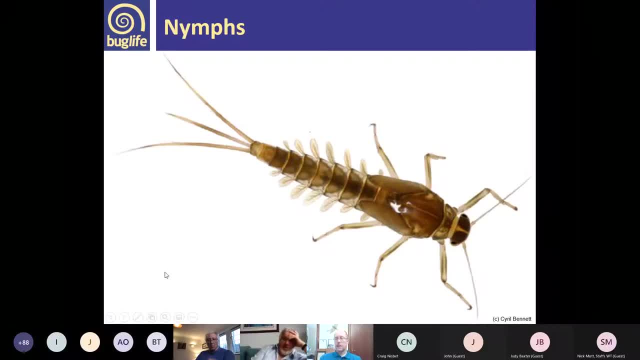 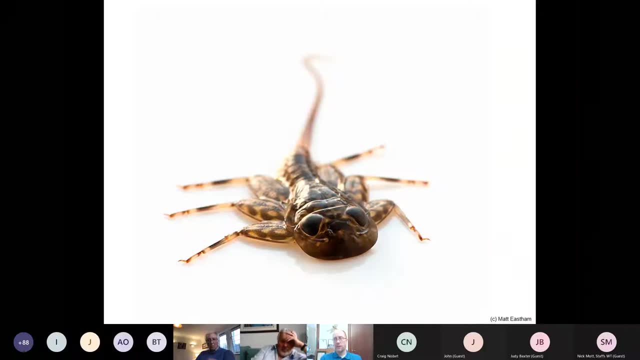 you would think that this was going to emerge in the next couple of days. The other main body form that we have in the UK is the flattened nymph, the sort of like very streamlined. These are the heptagenidae. They live in really fast flowing water and are superbly streamlined. 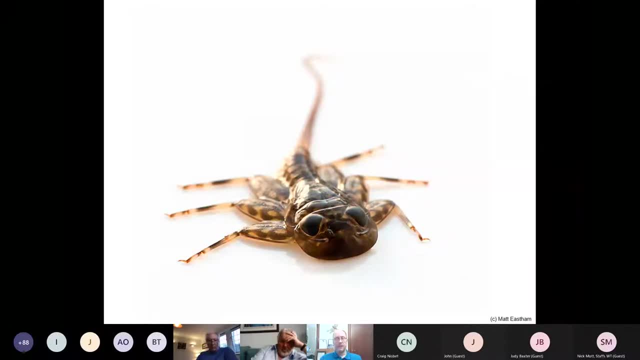 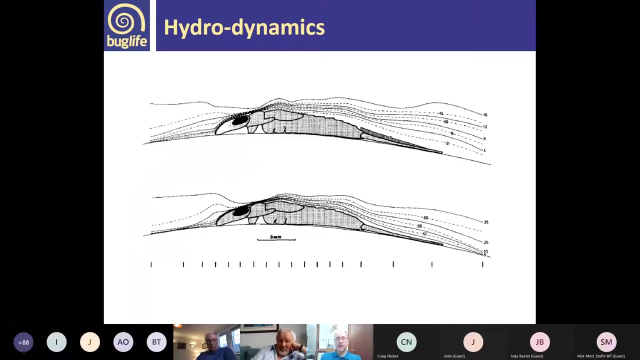 They've done various work on these species to look at just how effective they are at reducing drag and keeping themselves on the water, And this is some of the information out of the papers, And they have used this sort of the design of these nymphs. if you like to design Formula, 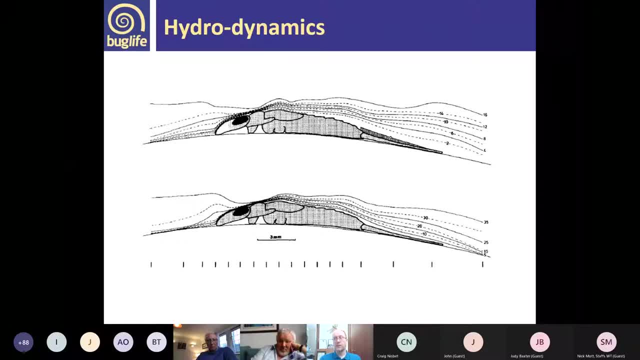 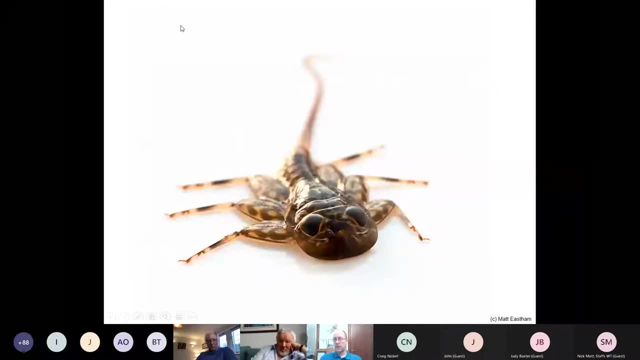 One cars. They've looked at how effective these are at keeping themselves on the ground, on the bed. If I go back to this one, you can see some of these have quite a lot of adaptations. This one has actually got a big bulge on its pronotum, which is a flattened area at the side which 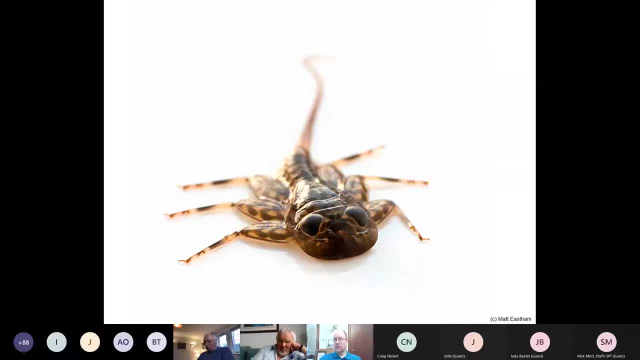 allows the water to push down on it. It's got this broad, flattened head which slopes back the way, So again it can put that into the current and the water will go straight over it. These big, powerful legs with the which are angled backwards so that the water again doesn't catch it. 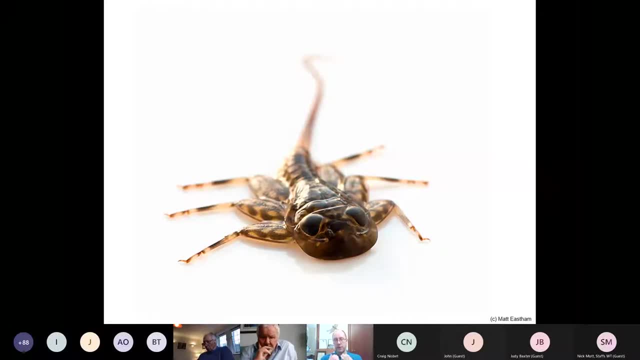 And then in the heptagenidae they've got, their gills are actually interlinked and overlapped down the side, So it creates a skirt which allows them to get even more downforce onto the bed. They're actually really difficult to get off of a tree or a stone, if you find one. 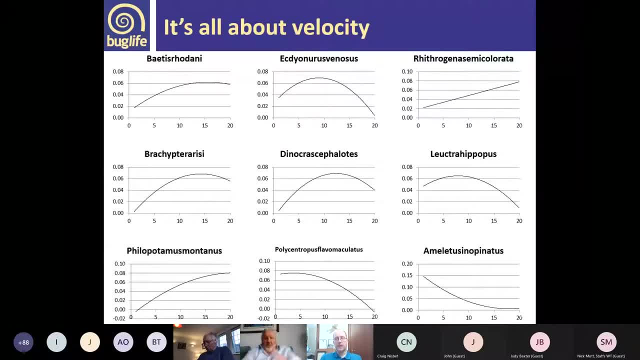 And that comes to the point that in all aquatic insects it's not about, you know, it's not about the flow, It's about the velocity, It's about how fast the flow is going. And these are just some graphs from some work that was done in Europe, looking at sheer stress at how much flow there. 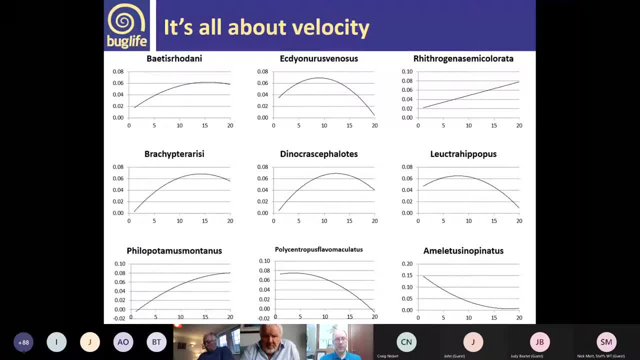 could be before an insect popped off a rock or whatever. And you see, there's quite a difference. The one I showed you there was Echogenerous venosus and you see that's a fairly medium in its requirements, whereas Rhythogena semicolorata, that one with the 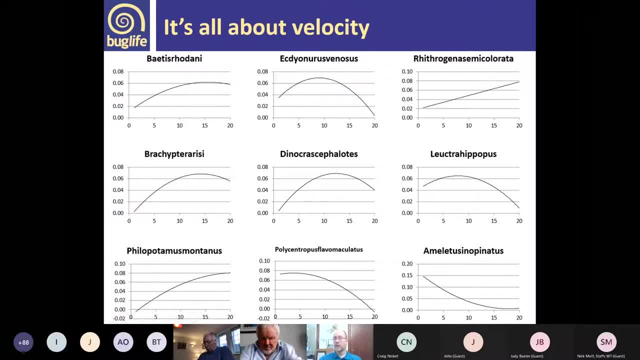 with the skirt of gills round it. it can just hold on and hold on, and hold on, right off the end of the scale. And then you can see other ones here, like Amelitis sinopinatus, which is clearly not doesn't like flow at all, It doesn't like fast flows at all And it prefers- and this one, 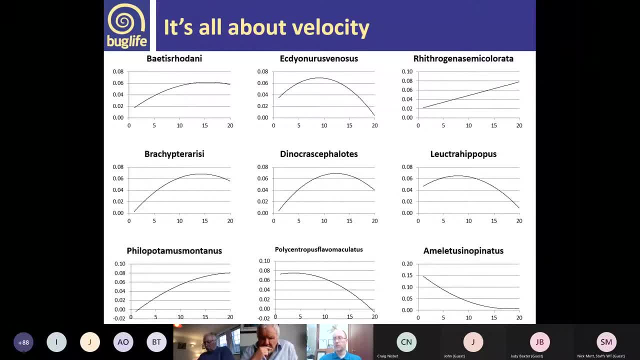 you find in, typically in pools, in rivers. So it's very much about what's happening in the river And that can dictate not just which lengths of river you find them, these species, in, but also the individual parts of that length you know. So it could be. 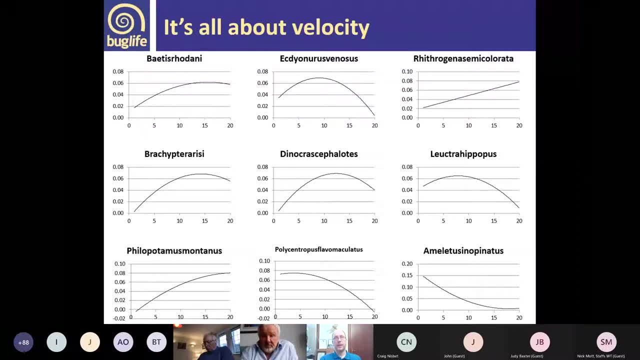 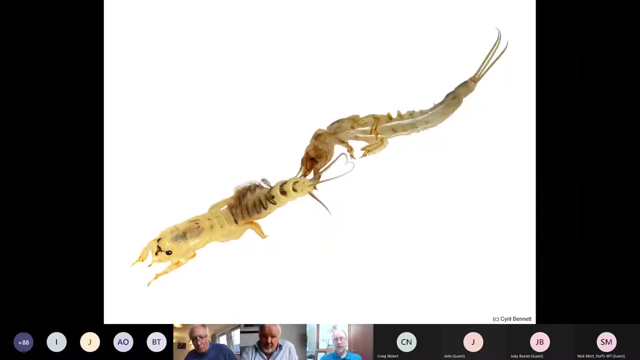 that you find some just behind the larger stones, where there's a little bit less flow, less velocity. Or you might find them in the very fast riffly bits, because they prefer that, As with all insects, the strength of the insect body is in the exoskeleton And for them to grow, to get rid of that exoskeleton And mayflies need to do this just the same as any others. But mayflies do it an awful lot of times. They can be up to 50 instars in some mayflies. So through that annual process, annual life cycle, they're shedding their skin, maybe 50 times. 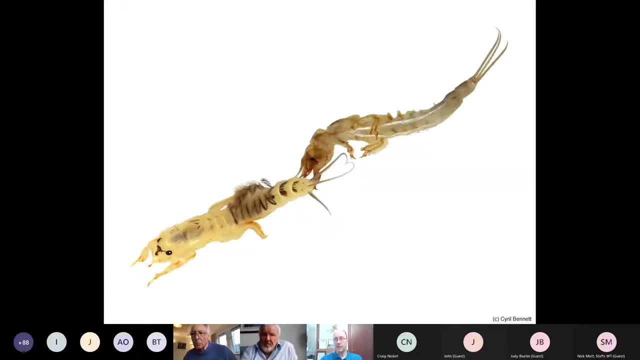 which is a lot, And when they shed their skin- this is an example of Ephemera danica shedding its skin, And you can see that the freshly emerged next instar is actually quite soft because that exoskeleton, that hard outer layer, hasn't hardened yet. And so it's fairly vulnerable at this time, And to put all that energy into developing the exoskeleton- and to do that maybe up to 50 times- there's a lot of effort goes into that. They don't feed either when they're molting, So once they've got to the stage where they need to molt, 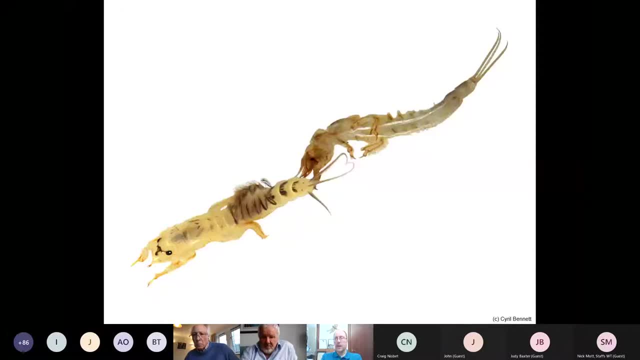 they'll stop feeding and they'll shed their skin. And you'll often find- if you're kick, sampling or collecting in any other way, you'll often find these shed skins, particularly around when there's been a hatch as well. I'm going to show you one species, one or two species now. 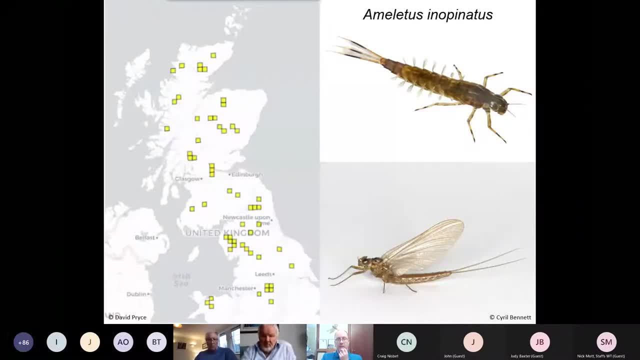 This is a species that is relatively uncommon in the UK. This is amelitis nopinatus. It's found in upland areas. It's called the upland summer mayfly And it's found in Wales, in Snowdonia, in the Pennines, the Peak District and throughout Scotland. It lives in particularly 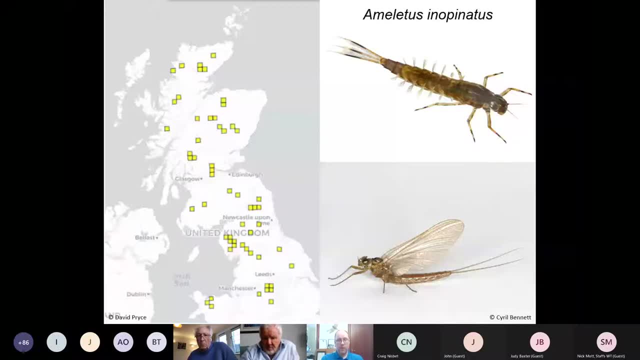 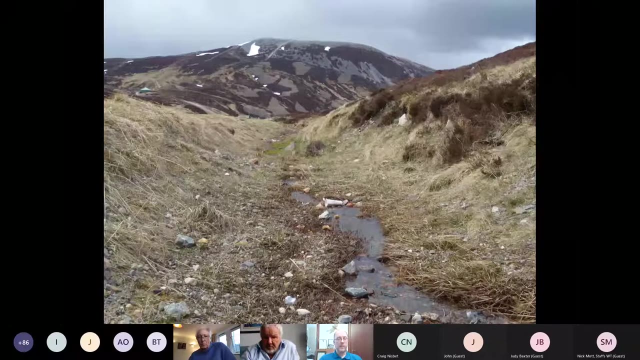 harsh environments. So it lives well up in the hills, often where there's a lot of cold weather. In this particular, I'm going to show you a site that we've sampled a lot. This is up at the top end of Glenshe. This is where it lives. It lives in this little stream. 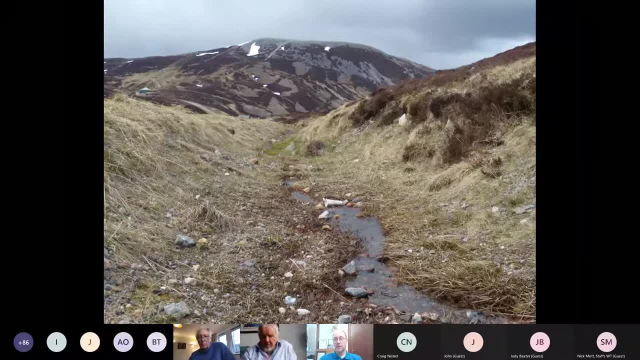 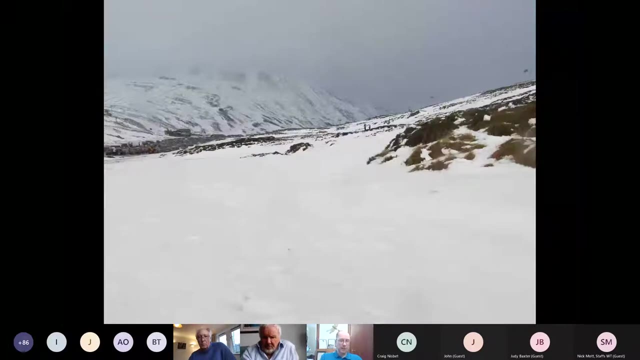 This is just as the streams drying in the summer, And so it started to pool and there's not much flow in it, And the mayfly at this stage is in its egg form and down in the gravels. In the winter there's not much flow either, because the thing freezes over and the flow actually stops as well. 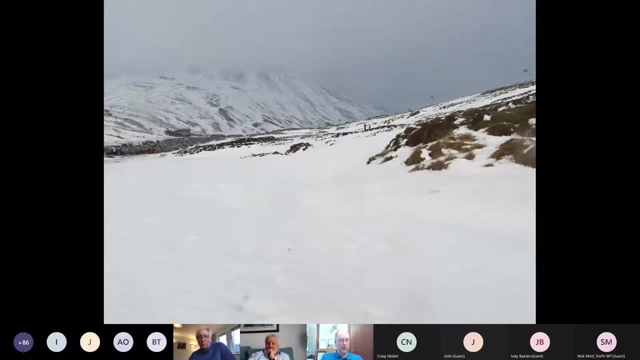 If you remember, back to the slide about velocity. amelitis nopinatus doesn't mind that. It doesn't mind living in a pool. In this case it's living under the ice, And the reason that this is one of my sampling sites is because I'm a fairly lazy entomologist And there's a large car park next to. 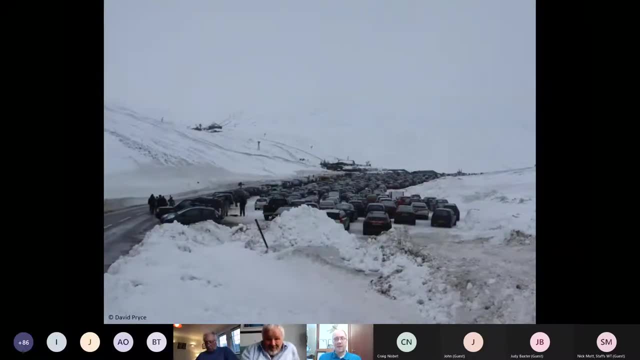 it for the ski centre And unfortunately my sampling point that I chose to begin with is underneath that white van because they've put the car park extended the car park over the stream And that causes a problem. There are some problems with pollution later in the spring when the ice is melting. 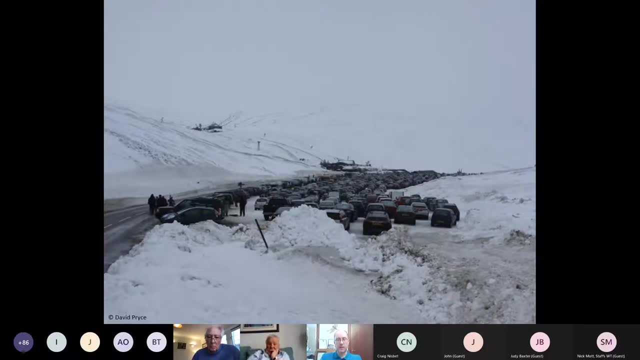 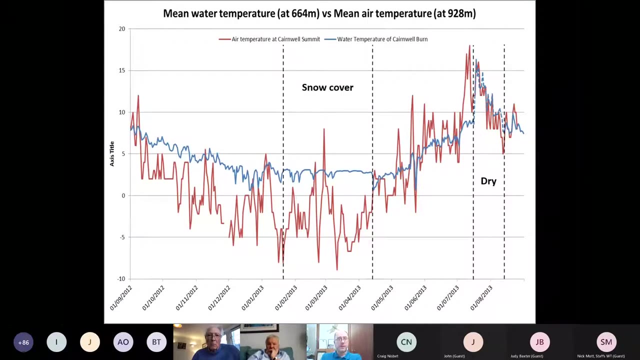 But, generally speaking, parts of this system up here are pristine. They've never changed. And temperature is the key thing for amelitis nopinatus, And what we've been looking at is how its growth is affected by temperature. And what's really interesting at this site here is this is a 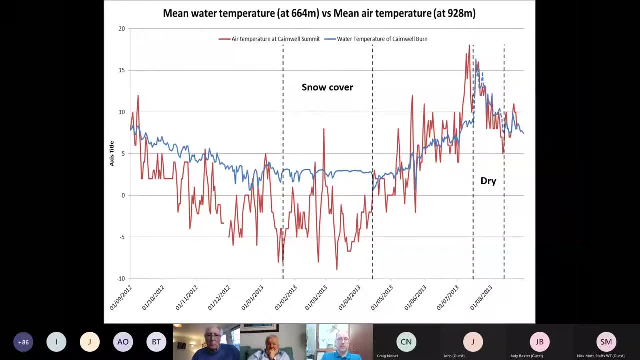 graph of air temperature versus water temperature round about that area. So the air temperature at the ski centre and water temperature in the stream. And when we get to the period of snow cover, the water temperature just levels off because it's insulated, The streams insulated and the water 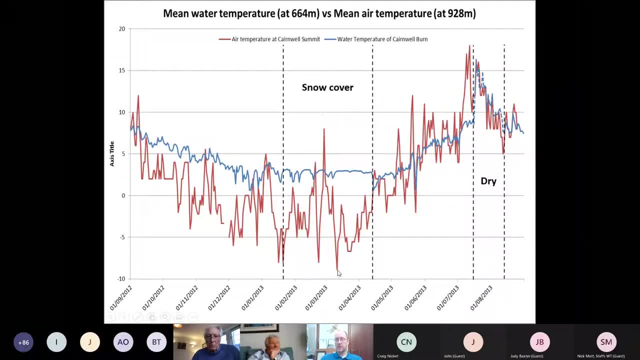 temperature is actually really constant over that period. Despite air temperature going down to minus- you know, minus nine or something there- and going up, the water temperature just stays the same. And you can see here as we go further on during the year, you've got this period here when the 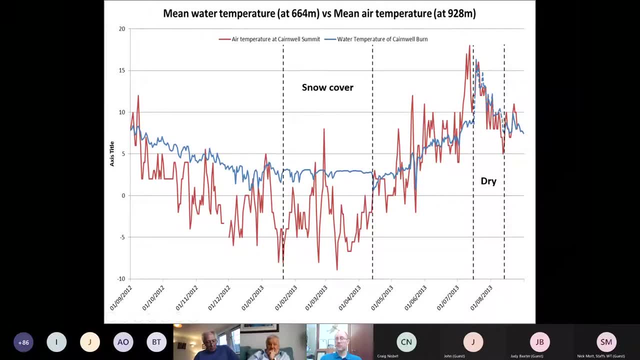 air temperature and the water temperature are the same, And that's when the river was, the stream had dried out And the logger had been exposed, So we're getting some of the water temperature here, and the water temperature is also very high, and the water temperature is very high in the place where we were when the stream was moving, And that's what we see here. 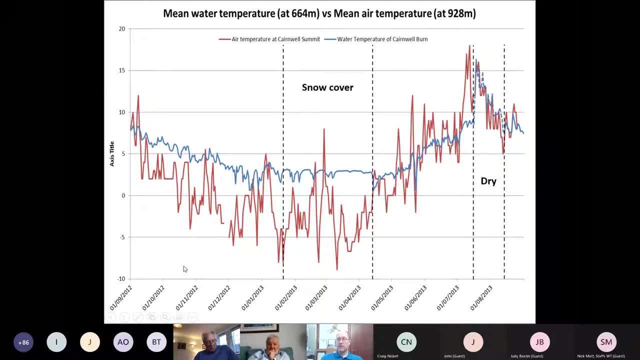 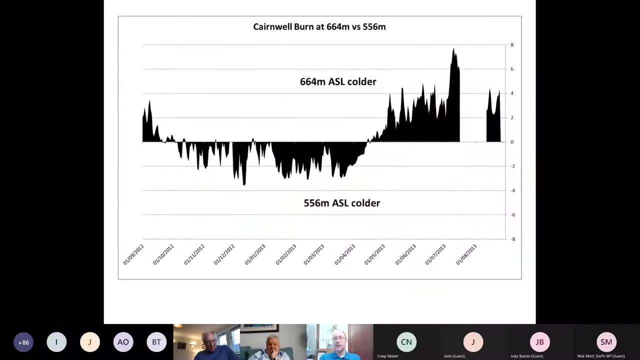 been exposed. So amylitis is present in this stream from around about the end of September, so around about here. so this is the growing period and it's got to get out before it dries up. The temperature: we looked at various points in the catchment and the temperature. 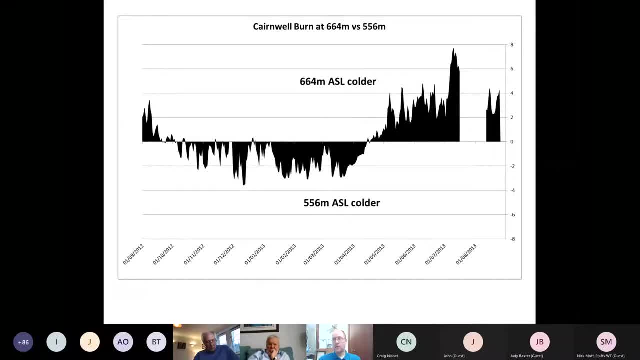 and what the difference was in the temperature. and what we found was that during the, the coldest parts of the year, the site at the highest altitude- the one that was covered with snow all the time- was actually the warmest site in terms of water temperature, and that meant. 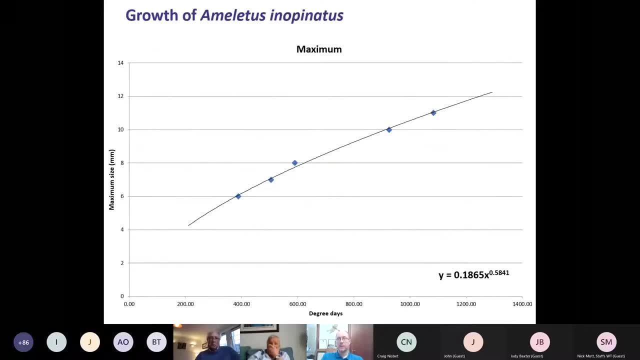 that amylitis inopinatus could actually develop relatively consistently right the way through and emerge at the same time as the rest of the population in that stream, which was a very good thing, Quite interesting. and what is particularly worrying, though, is when you start looking at. 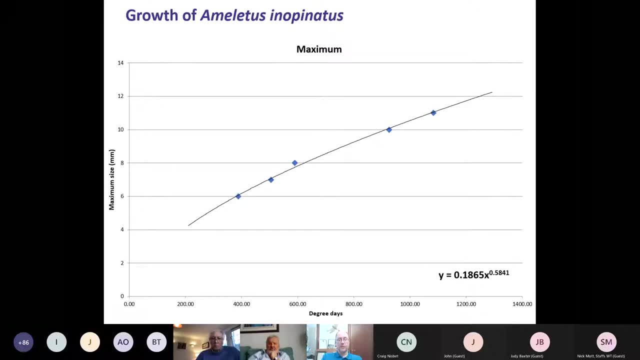 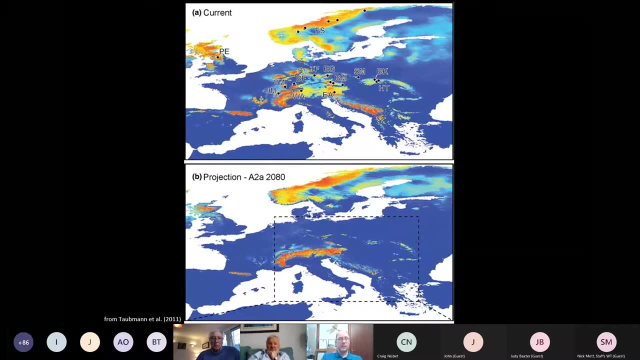 climate change and what may happen to temperatures in Europe over the next sort of 50 years or so, you start to see that there's going to be a big pressure on these species that are living at high altitude. This is a piece of work that was done by Taubman et al in 2011 and it looked at 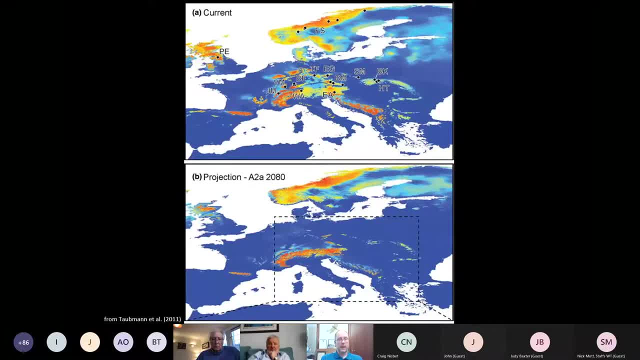 current temperature, current climate conditions and projected climate conditions and looked at what the distribution of amylitis inopinatus may be under those projections. and you can see this is the current at the top here and it shows there's strong populations in Scandinavia and 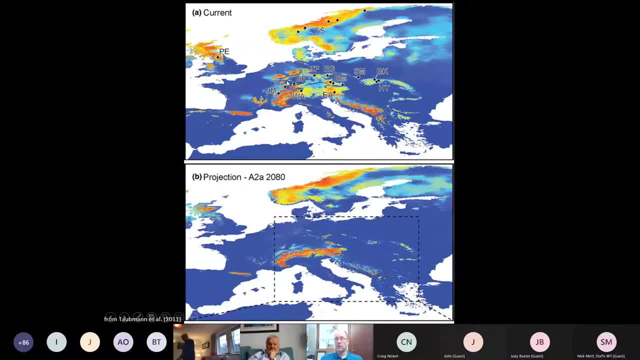 in Scotland and the areas that I mentioned and also in Central Europe. but by 2080 it's going to be a lot more than that. It's predicted that it'll be lost from much of Central Europe. We'll still have populations in Scandinavia and Scotland. It'll be lost from much of 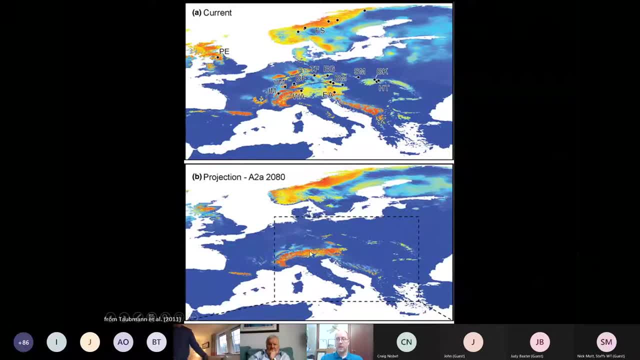 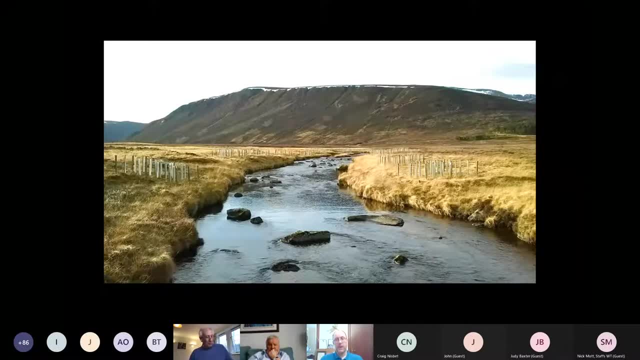 some trees along the river. As long as we get them high enough up the catchment, they can help to cool the water by shading it. This is a piece of work that was done actually for perimussels rather than amylitis in the River Mick up in the Scottish Highlands. 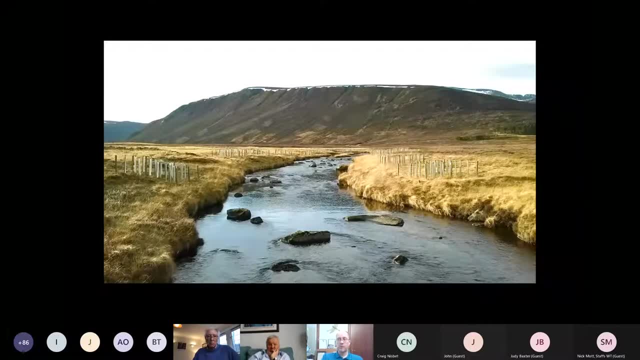 and these little patches of trees will grow and provide some shade for the river, But we need to have the right tree in the right place and make sure that winter sunshine still gets to the river in the places where it's needed, because that can be important for the development of other 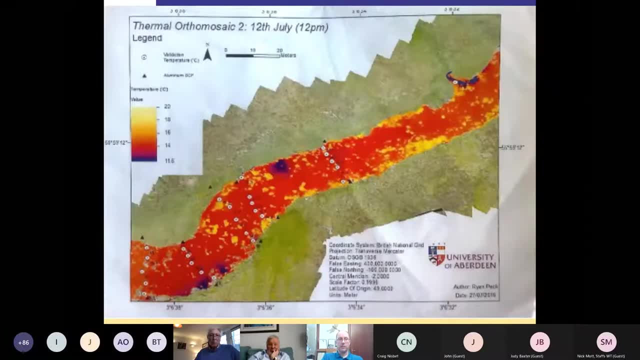 stoneflies and mayflies. We are working with University of Aberdeen to look at just exactly how we target those patches. We know which stretches need the trees, but where do we put them? This is actually an image from a drone with a thermal camera on it. It can show you. 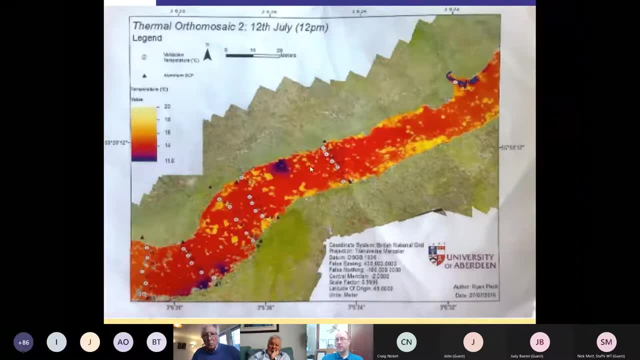 where the cold patches and warm patches of the river are. So we can see here this blue patch. here is probably a groundwater upwelling. There's a tributary coming in here that's providing some colder water, But along this bank here. 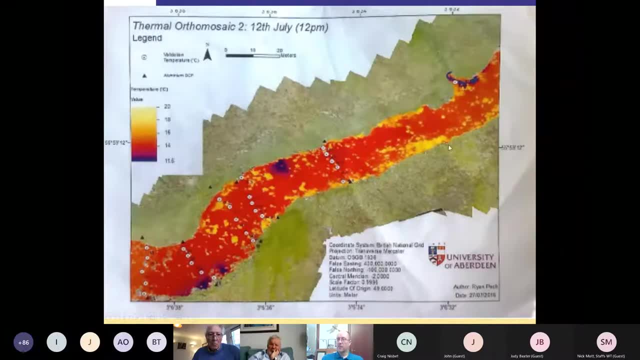 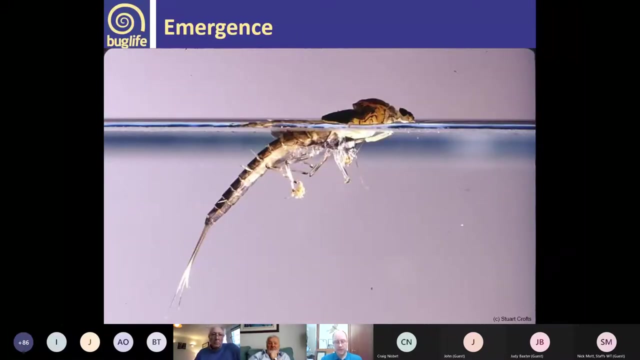 there's big yellow patches where, if we were able to put some trees right here in this area, we might be able to cool that patch there. So once they've gone through going back onto the life cycle, once they've gone through their nymph or larval stage, they need to get out the water. These are aquatic insects. They need to. 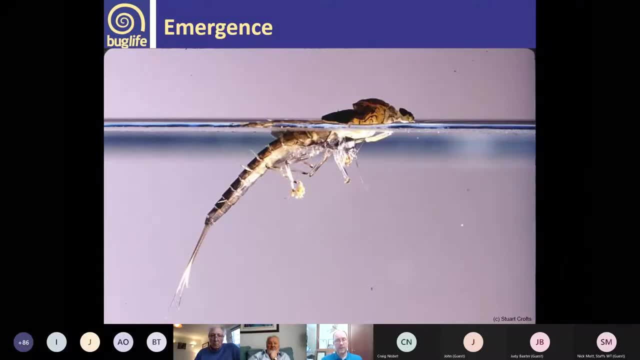 get out of the water to take to the air, to become adults. Most of them emerge at the surface of the water. So what will happen is that the larvae will go down to the bed of the river or pond or lake and it will do a couple of practice runs. It will swim up to the surface. hang there for a bit. 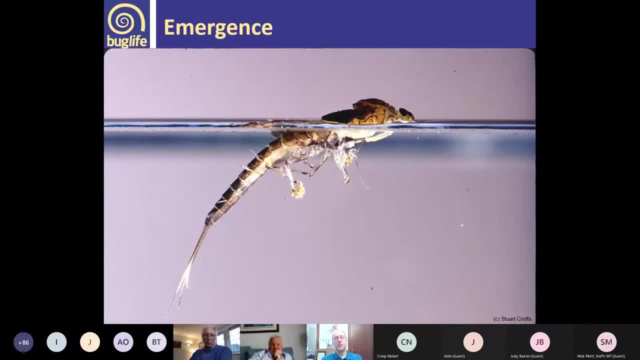 and then swim back down And it'll do that a couple of times And it's probably just checking out conditions at that stage. When it's ready to go, it will swim up to the surface And as it hits the surface the back of the thorax splits open and the adult inside is covered. 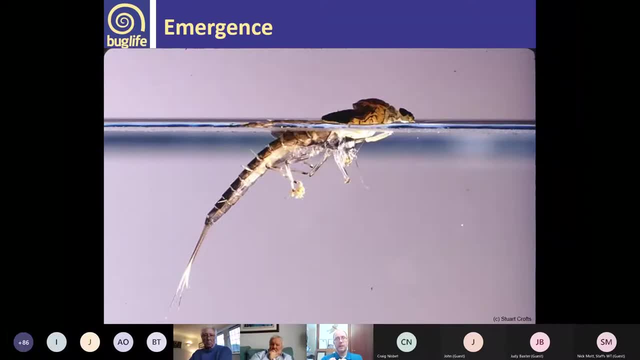 in tiny little hairs, And these hairs repel water and they open up a little window that allows the adult to crawl out. As you can see in this image here, this is a abatis larvae that has got up to the surface. It's cracked open its back of its thorax and it's now just pulling itself out onto. 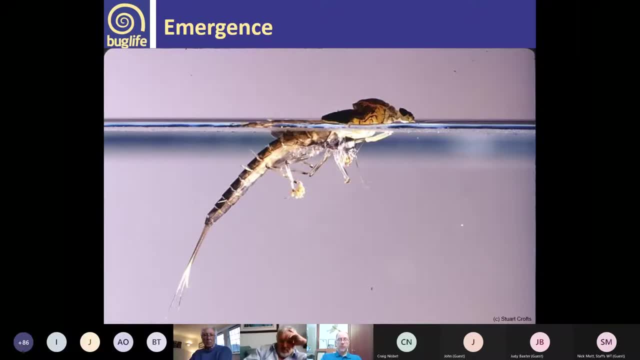 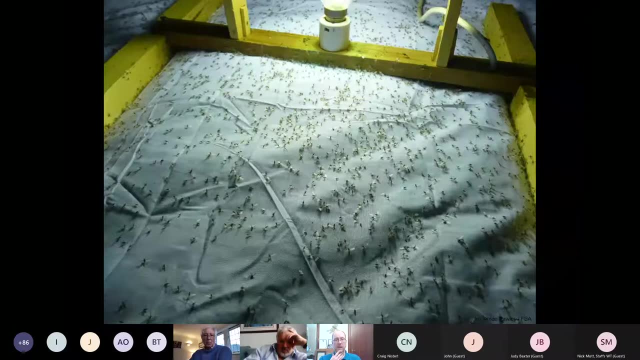 the surface of the water. And when they do this, they can do this in huge numbers. We trapped at Windermere in the Lake District one year And we were actually looking for caddisflies And we were conscious of this sort of sort of miscarriage, And we were actually looking for caddisflies And we 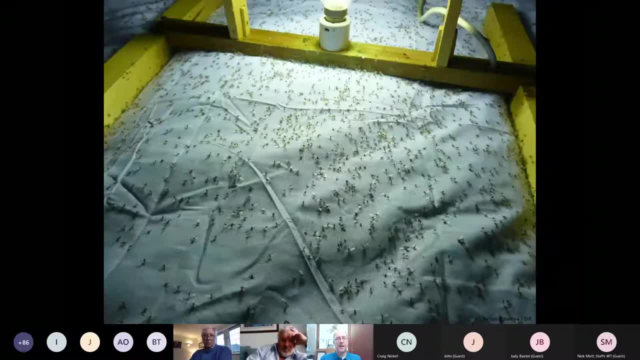 were conscious of this sort of miscarriage And we were actually looking for caddisflies. And we were actually conscious of this sort of miscarriage And we were actually looking for a mist or this smoke coming across Windermere, And then it hit the trap And it was. 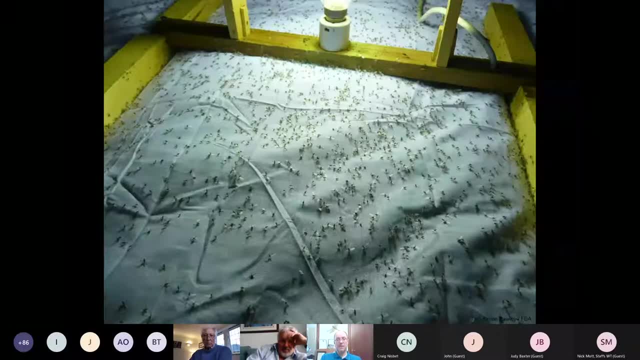 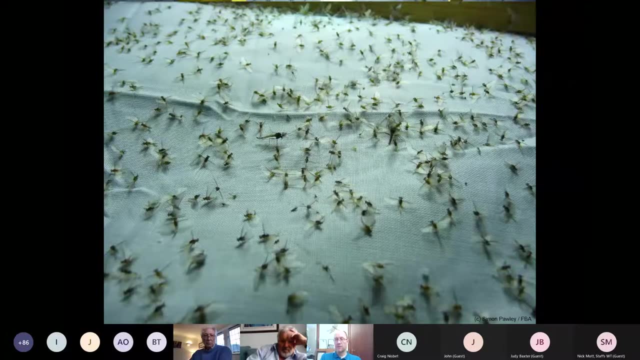 it was a swarm of caddis mayflies And you see, there were just hundreds of them And there were some midges in there as well, But the majority of them were these little caddis myflies And that was a. that was a big hatch and it's one you kind of could predict from there. 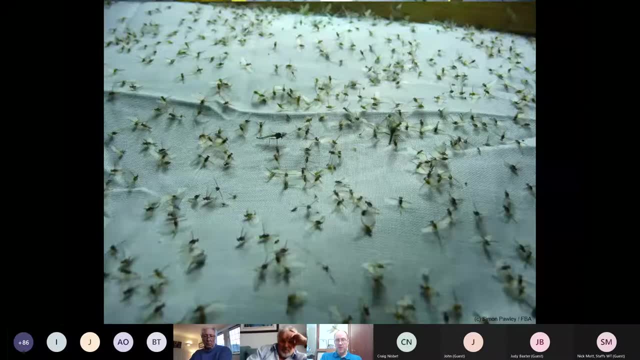 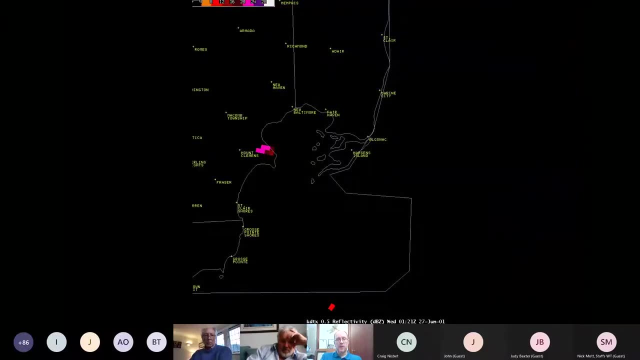 But there are some huge hatches in the world And so big that you can actually pick them up on weather radar. This is a little sequence from Lake St Clair over in the States And this is the start of a hatch, these little pink pixels there And these are 10 minute intervals. 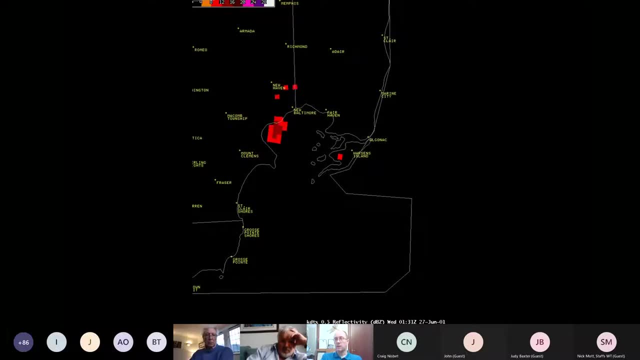 these animations. So we start to see the hatch build and build. That's after 30 minutes, 40 minutes, And then there, at that point, there you see those two intense points, the two pink points, that is the mating swarm. So that's where the males and the females 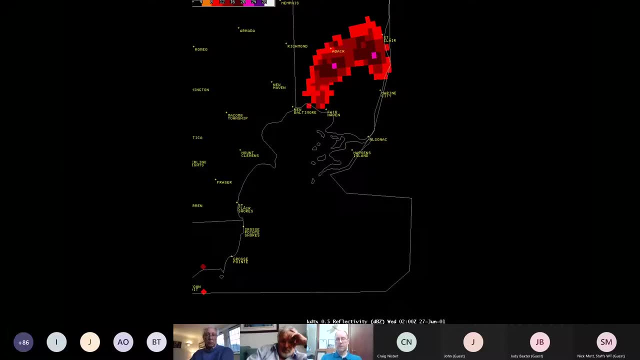 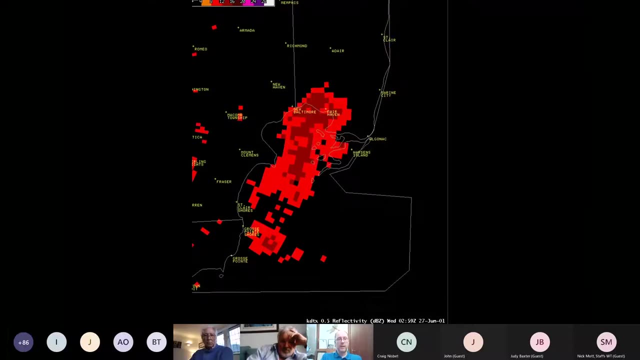 have come together And they're in these massive mating swarms, And then, an hour later, in the sequence of data, all the females are back on the lake laying their eggs. So you can actually track the life cycle of these insects using, you know, remotely. 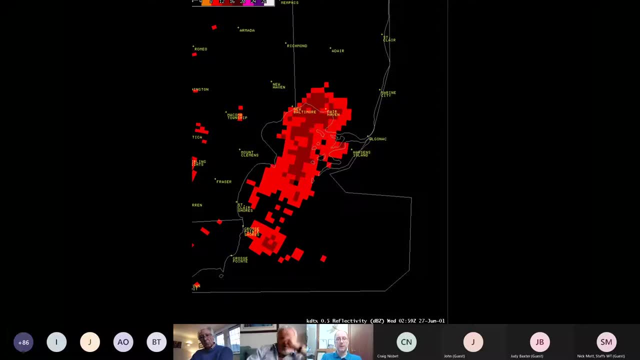 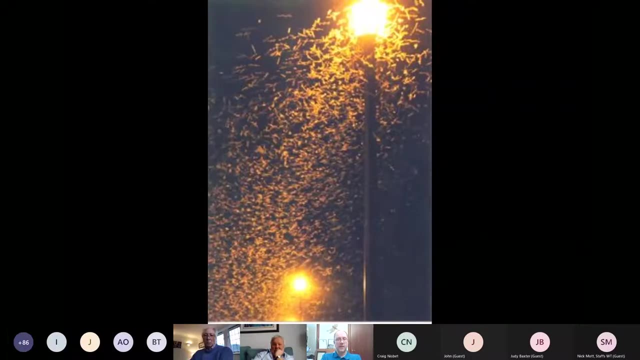 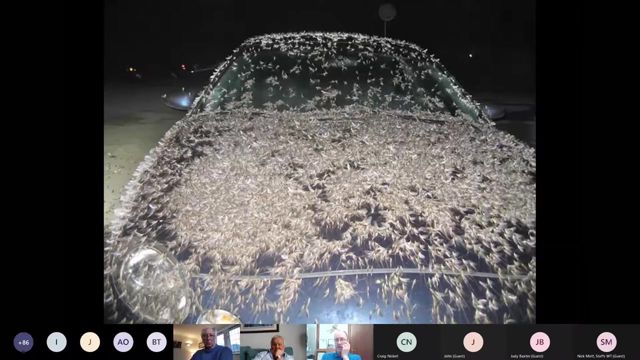 using weather data. That's such a large hatch And that's what it sort of looks like. It is phenomenal. They are attracted to lights. They cover surfaces. This is actually from the Mississippi. This is Hexagenia lumbata And the massive hatches in the lower Mississippi. 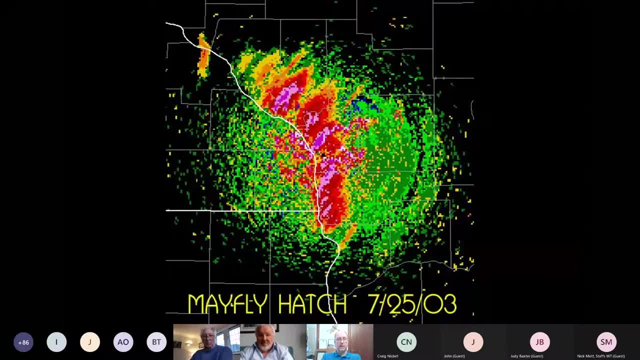 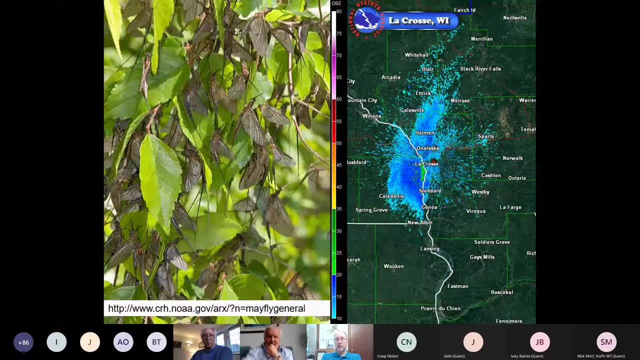 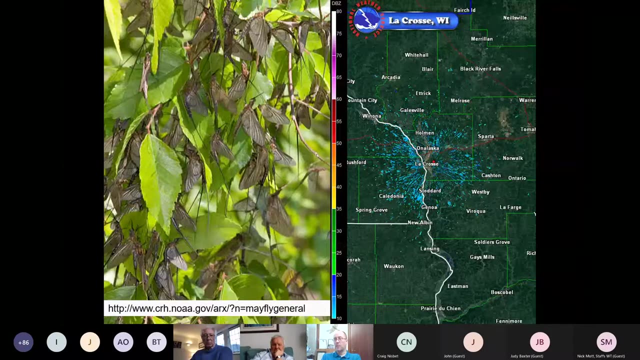 That's another piece of weather data there from 2003,, which is a particularly big hatch on the Mississippi, And they have a service- the US Met Office, if you like- have a service that allows you to track these hatches. And that's just an animation from La Crosse in. 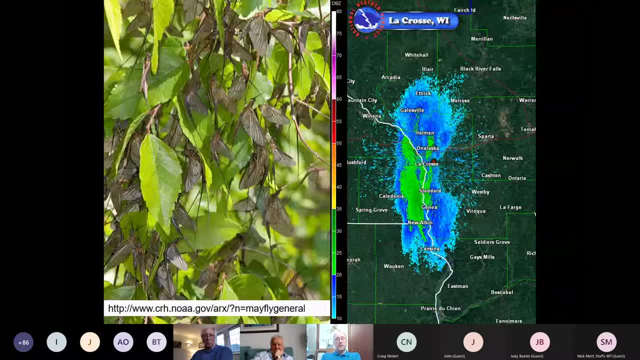 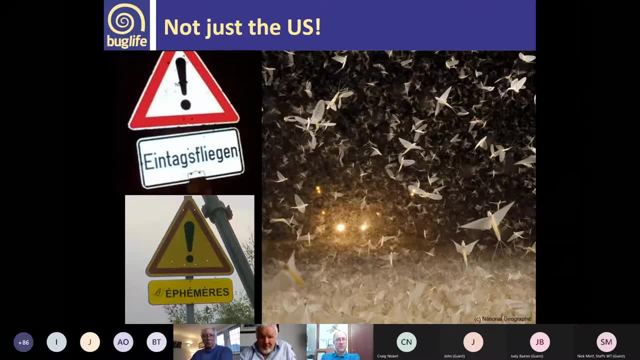 And you can see. you know there's warning signs put up because these things are pretty slippy when they're on the road. You get a drift of mayflies on the road And certainly they're in decline in Europe And we don't get them in the UK, But it's quite an amazing sight to see. We do get large hatches in the UK We get early on in the season. Ruthugina, germanica, can have large hatches on, particularly on the River Tweed, But on some other rivers as well And in the chalk streams. 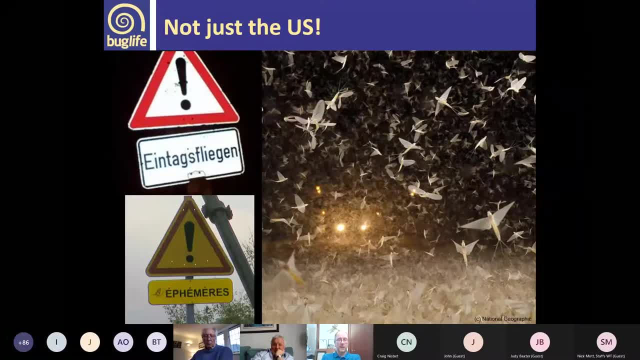 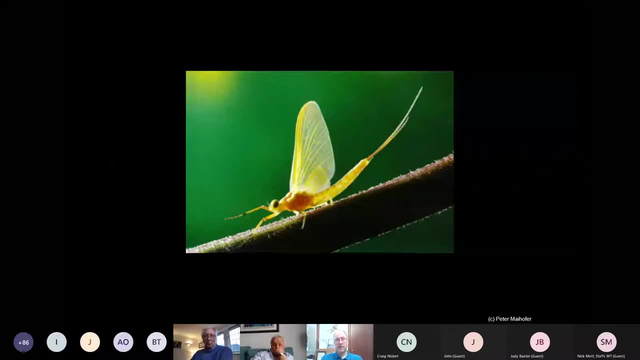 we can have quite large hatches of ephemera danica in some areas Once they've emerged. mayflies are unique as insects in having two adult stages, So most insects emerge from the larvae or the pupa and then that's it: They're an adult. 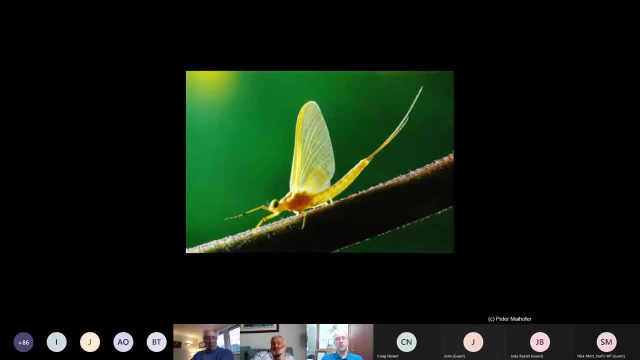 In mayflies. they've got another resting stage, if you like, called the subimago, And this is a. this looks like an adult, but technically it's actually still. it's a last instar larva because it's not sexually mature and it's not. it's not fully, it's not its final stage. 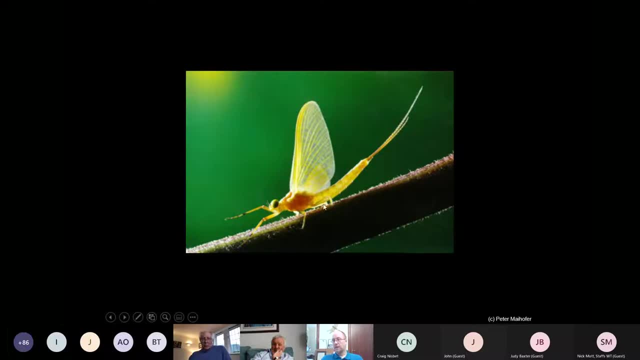 This is a Portimanthus luteus subimago. You can see that the wings are opaque and the body is coloured. The tails are relatively short and the legs are relatively short. This is a male. here We can just about see the developing 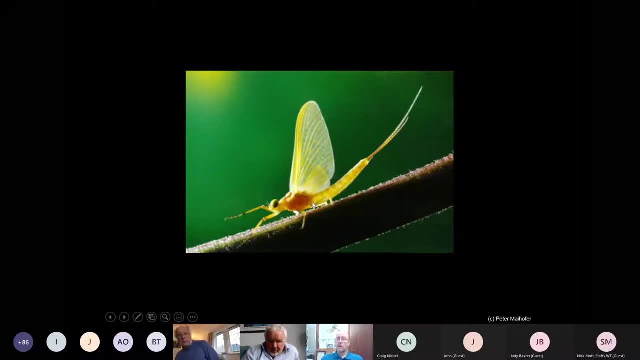 plump genitalia, the forceps here And this. this now needs to go off and it needs to molt again, And so this will go off to the side of the river. it'll find a piece of vegetation or some other substrate for it to sit on and it will molt again. 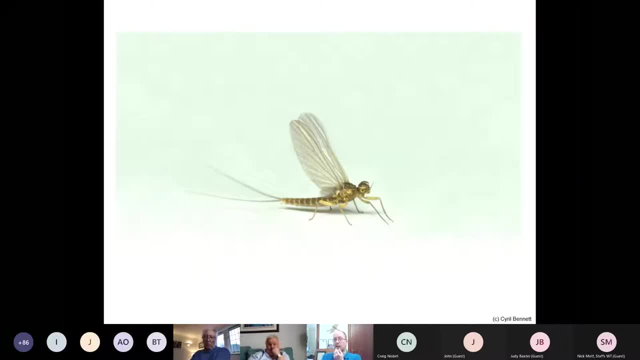 And it does this. and just, there's another little sequence here, this time of a Betis nymphs ohne betis subimago, And it'll do. it will kind of do the same process as it did as a, as a larva, it will um flatten down its wings. 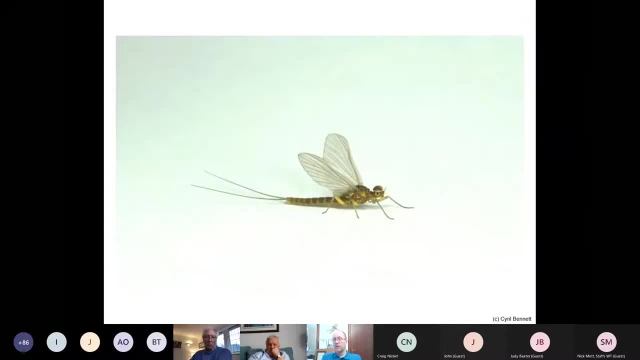 crack open the, the thorax and then crawl out, and this is just a little sequence that shows that. so there's the wings going down. at this point the, the larvae, the, the thorax is splitting and the full adult, the imago, is crawling out from that. um, sub imago skin. 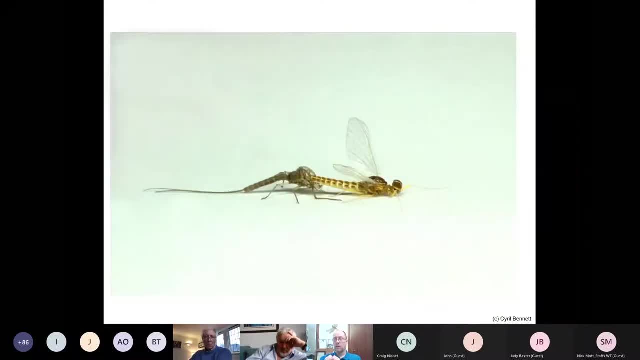 and it really is as quick as that, so they can't hang about. once they've decided they're going to do this, um, when they, when they do this, you know they, uh, this is now, then, fully mature. um, you, you will find these little shucks, these little cast skins left on leaves and things like that, um, but 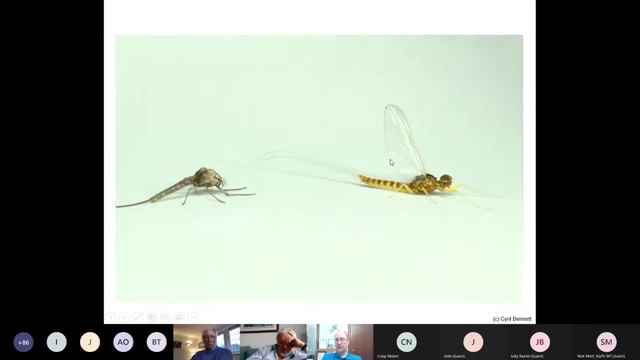 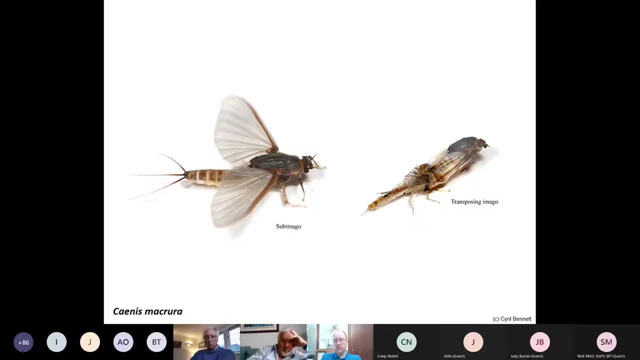 overnight and then will emerge in the in the morning, in the canis. they, they can they, often they just as they are emerging from the river. i i've actually seen them crawling up my chest waders, calling up the leg of the chest waders, and as they're doing it, they're, they're emerging. 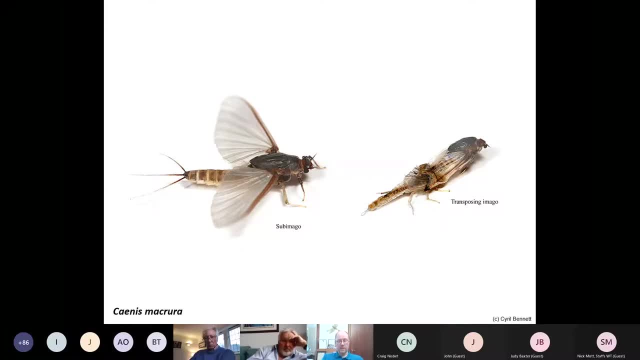 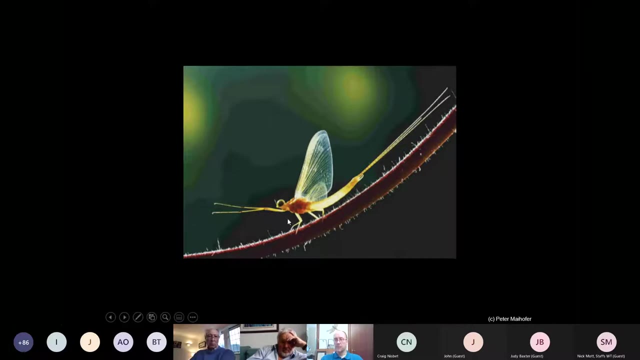 into the imago. so they're. they're coming out the water, um, as a sub imago and then just crawling up and becoming the manual before it gets to up to the top of the waders, um. so this is the same individual we saw earlier on- is the sub imago. this is the imago and you can see the legs are much. 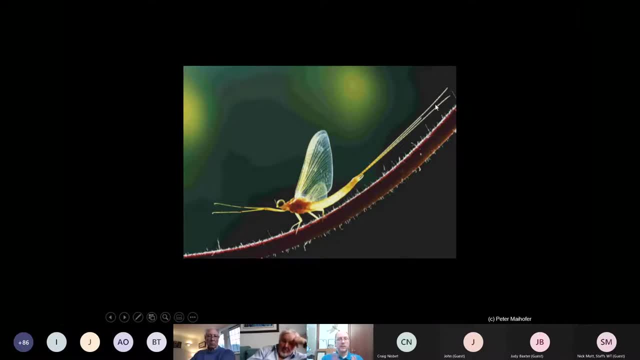 the tails are much longer. the tails are longer to allow it to stabilize itself in flight. um. the legs are longer because this is a male and when, when they go and try and find a female, what will happen is that the male will go off and it will swarm. it will create a sort of a leg or a. 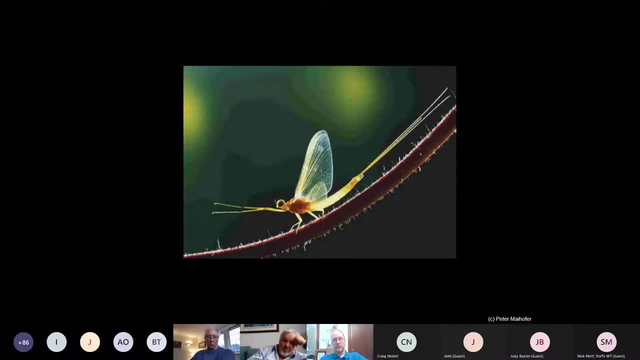 swarm with it and what they do is they. they flap their wings to go up in the swarm and then float down and they do this sort of circular motion. um, all the time they are looking for a female to come to that swarm and you can see that the the eyes on this individual are large and up, pointing up. 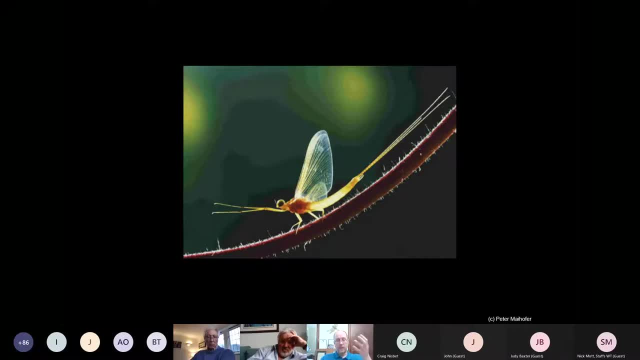 the way, um, and that's because the female will come in above this in the the, in the swarm, and then the male will actually put these long legs right over the top of her wings and immobilize her to stop her from flying, and then they'll couple, then mate and fall out of the swarm. 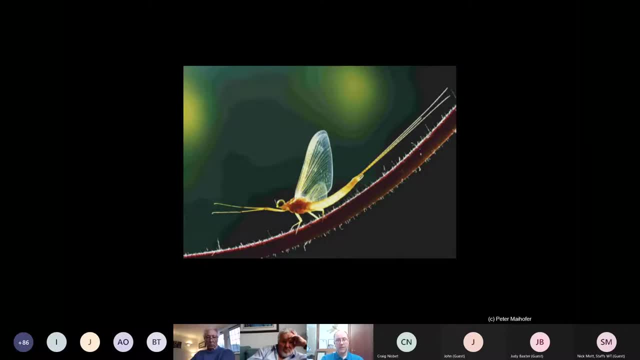 and as they fall out, by the time that they reach the ground, the female has, uh, has been fertilized and the eggs have been fertilized, and the- the male is- is is dying at that point. it won't survive much longer after that, and sometimes they'll fall straight out into into. 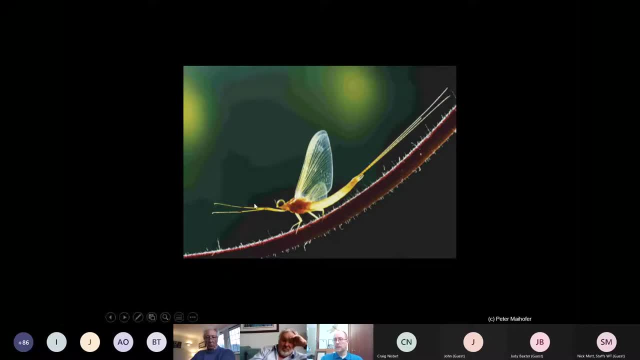 the river. um, the other thing to see on this is that the body is now clear, apart from the wing muscle at this end here to power the wings and the sperm packet that's going to pass on to the female. um, the wings are clear, they're no longer opaque, and the reason they were opaque before is because 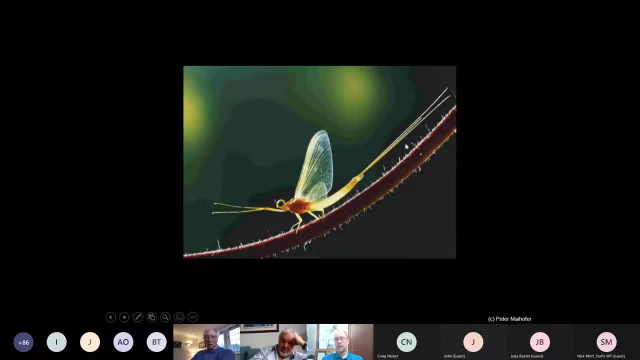 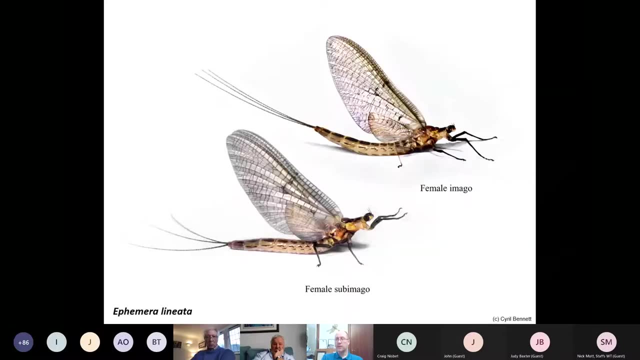 i can see there's a single layer of wings inside them, so it's basically a double, a double layer of wings. um, so those are the main differences between the subimago and the imago, and there's just an example of using. chopped'mago means female presubstantial brineata with the the more muted colors. 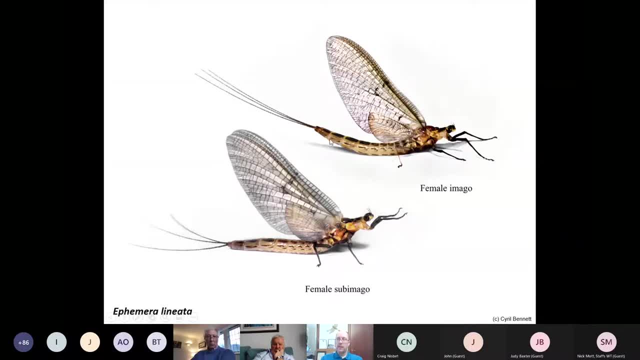 and these are the females. just to just to show you in the female that the, the color remains in the body because the body is full of eggs. um, so it's not a really dynamic element for clear, as in the male. and you see, it doesn't have quite as long legs because it doesn't need those. 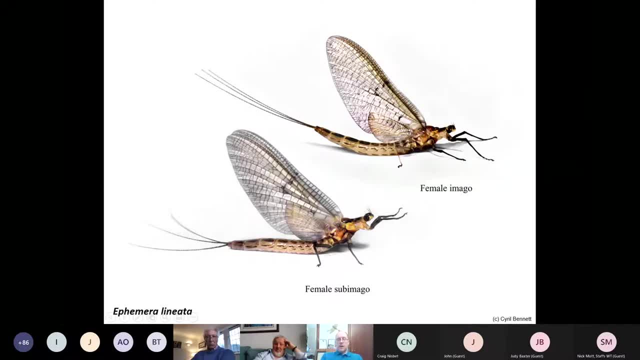 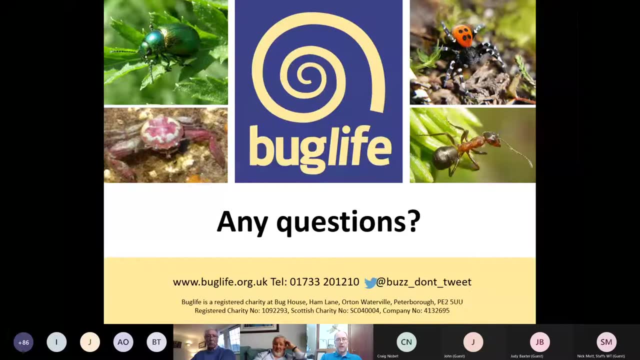 or large eyes. Okay, so that is a really whistle-stop tour through the life cycles and various other bits and pieces about mayflies. I'm going to stop there and see if anybody's got any questions before we move on to some information about identifying mayfly larvae. 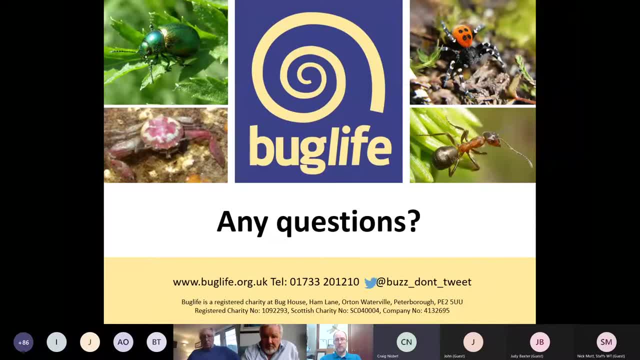 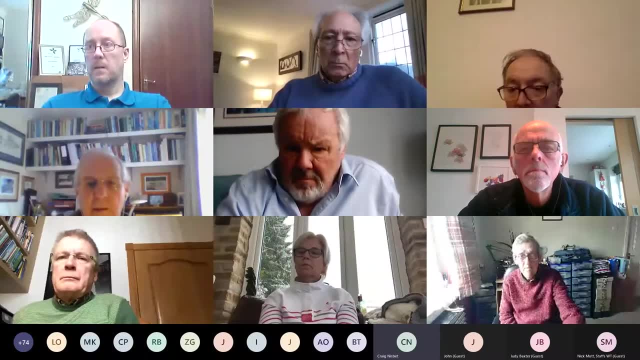 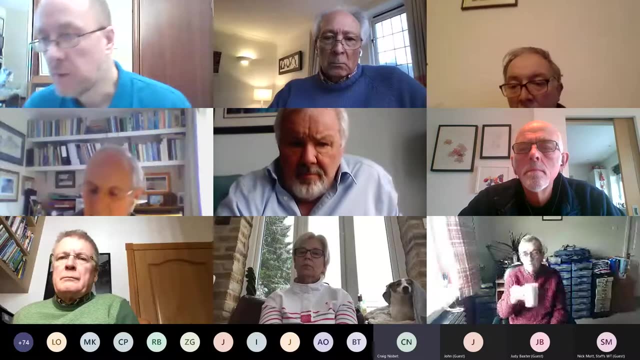 Brilliant. thanks, Greg. We had one question earlier on your talking about the eggs and females from Brian Shaw. I'm not sure if it's a cypher. can you see the conversation I'll hold on? I'll just get it in the meeting chat. Wait, one baited egg per. 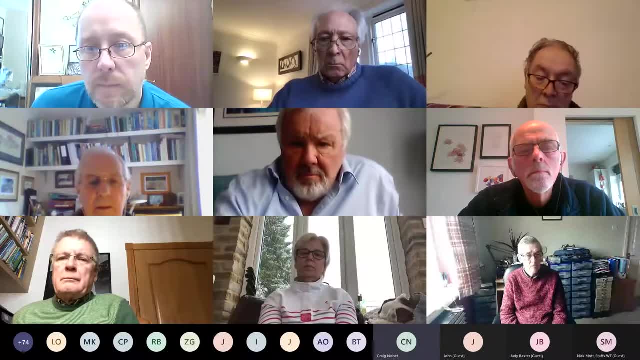 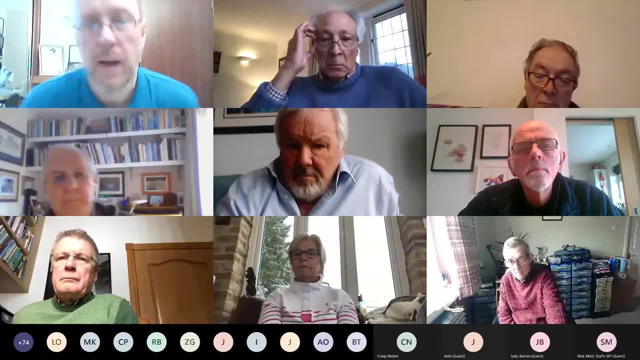 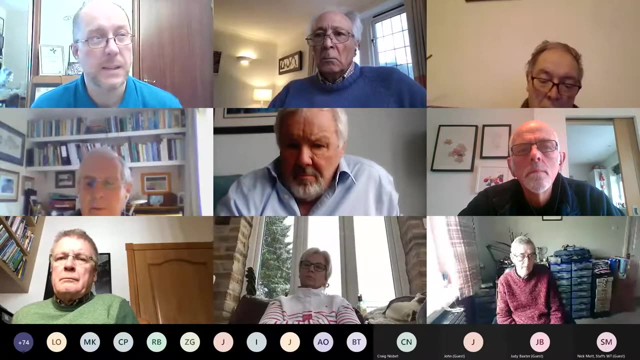 patch of female, One baited patch per female. Yes, mostly Some of the bigger ones. we'll try and we'll do other ones. They tend to lay their eggs and then they get washed off. So, Betis, adults will lay somewhere between three and four thousand eggs. 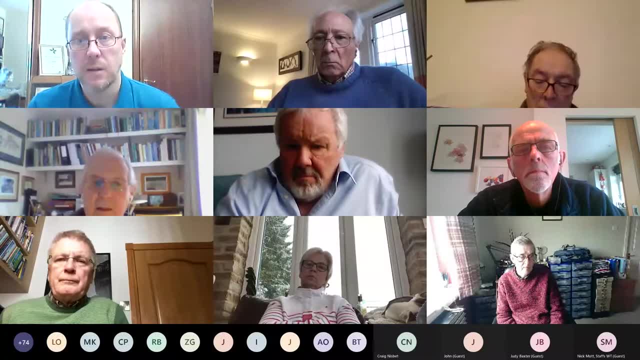 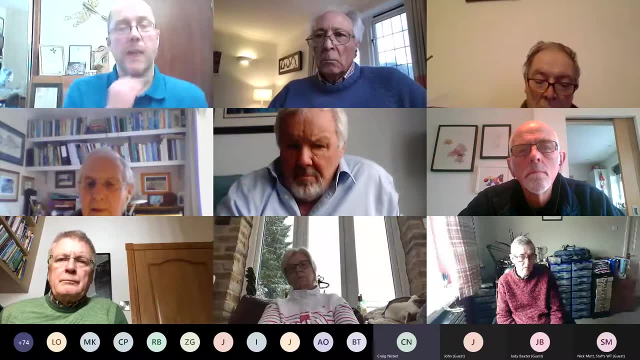 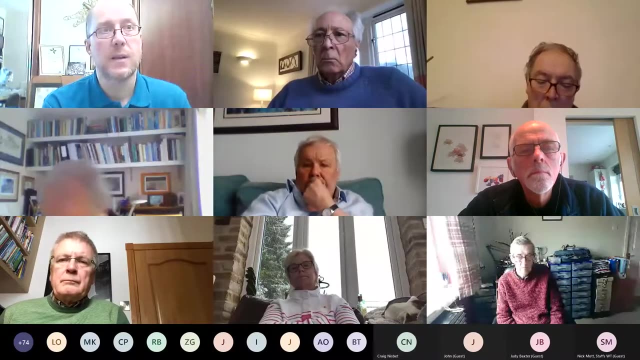 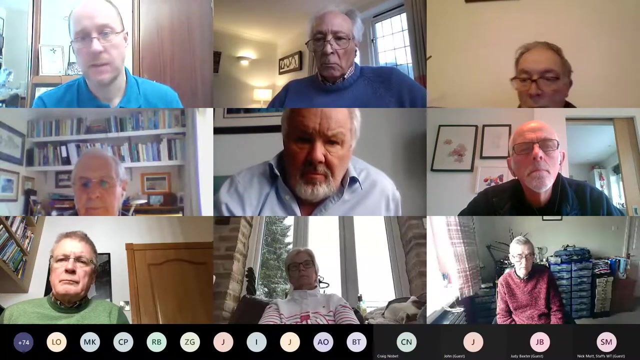 so they will have several patches. I'm just trying to find the chat. Yeah, and you do find. on some of these rocks you'll find. after one set of larvae have hatched out, eggs will be laid on top of that. So there'll. 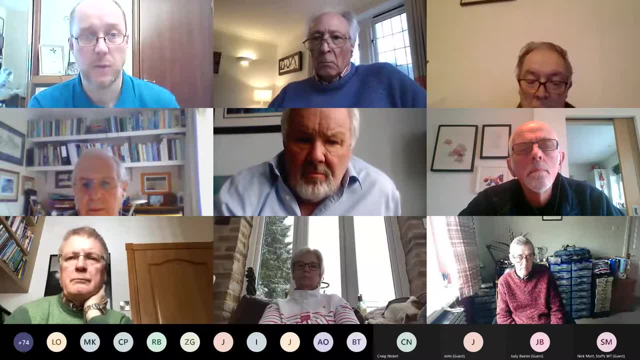 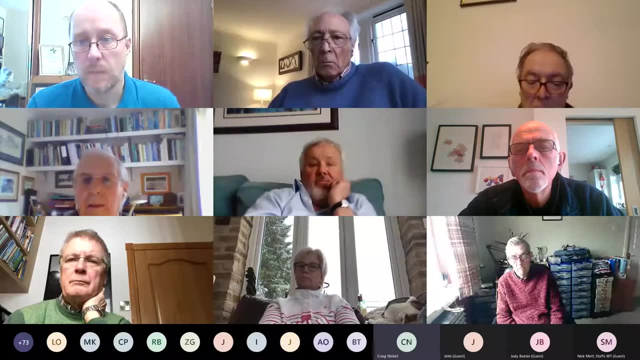 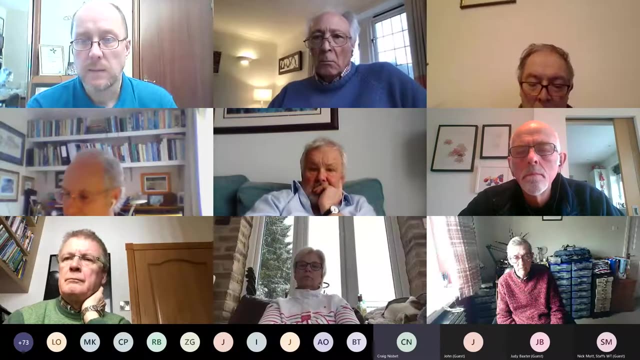 be a continual sort of like laying of eggs, particularly if there's not many exposed rocks in the stream. Okay, a question from Jane Ackerman. Do we know why they go through so many instars compared to other insects? I think it's probably the rapid growth. They are growing. you know they've got a pretty limited time to grow. The species that are going through a lot of instars are having to grow in maybe two or three months time. So they've got to. they've got to basically change their skin quickly to get to the size that they need to emerge. 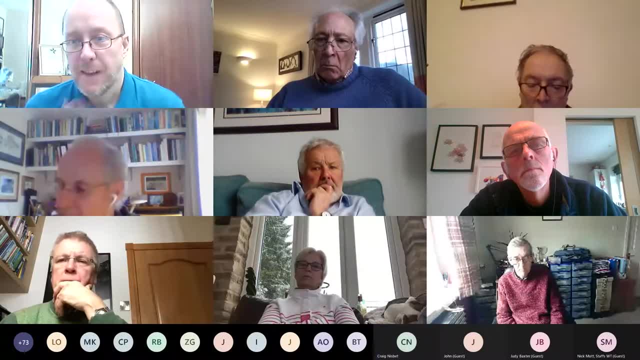 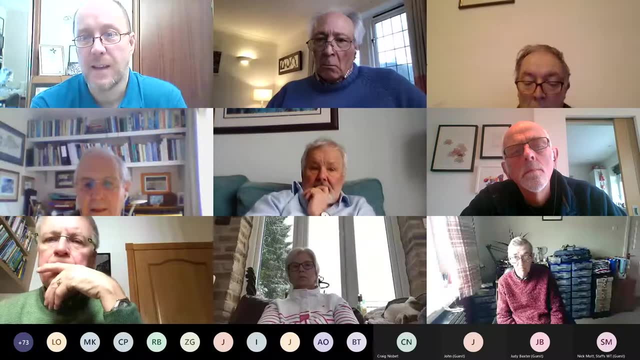 I see the next question: how do the front legs lengthen so quickly? So that is a really good question and I don't know the answer to that. I'm not aware of much research on on the physiological changes in the sub imago and 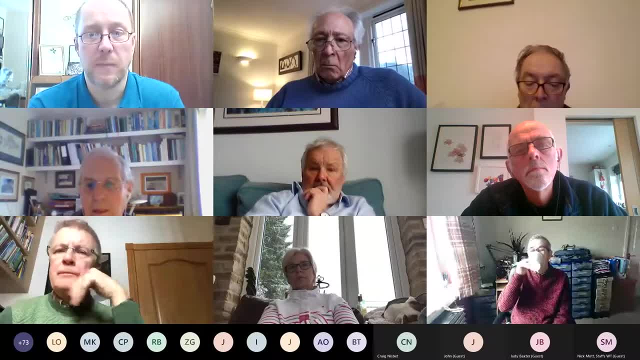 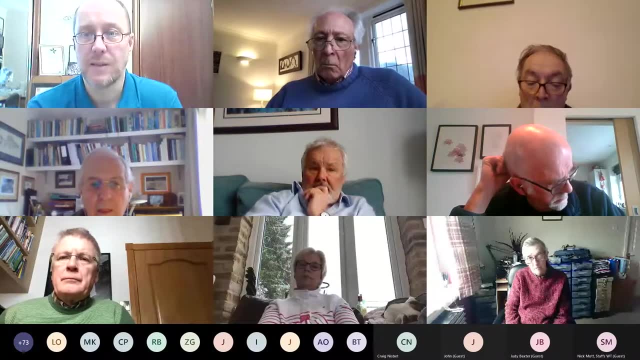 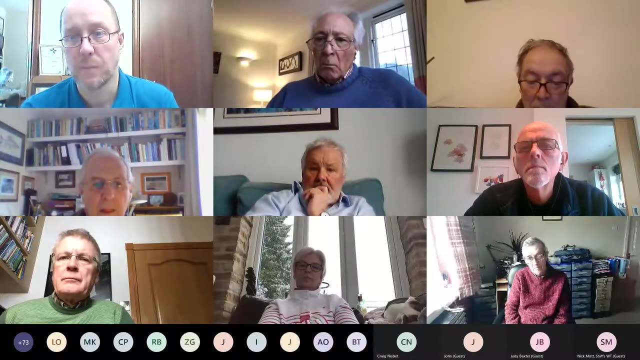 the to the imago stage. but it is interesting because there is a massive change in size and there's not much. it's not as if I don't know, it's not. it's. It's not as if they're going through a pupil stage that allows them to reconstitute their body shape. 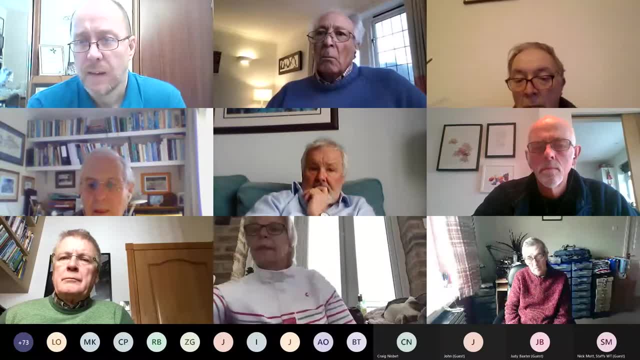 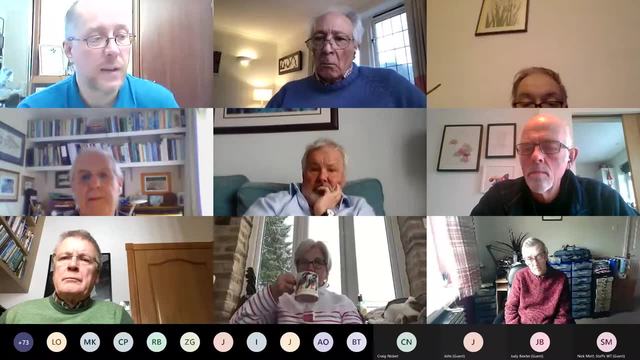 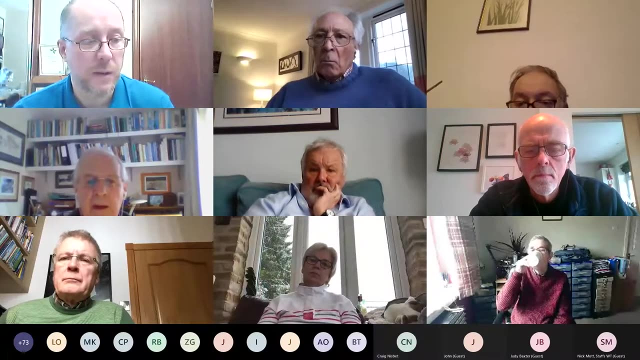 No, I don't know the answer to that. Will some species benefit from increasing temperatures? Yes, indeed, And so there are. there is, there are moves in a lot of aquatic insect groups, So dragonflies in particular are are, because they're quite good dispersers. 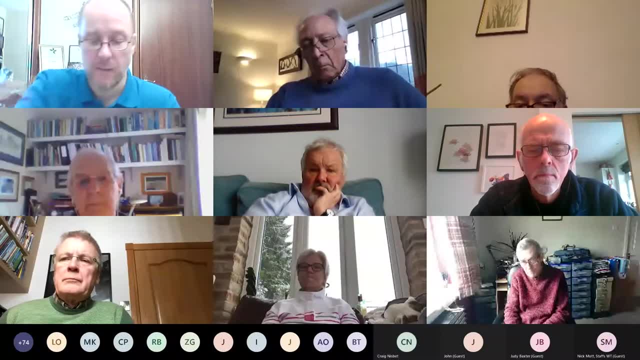 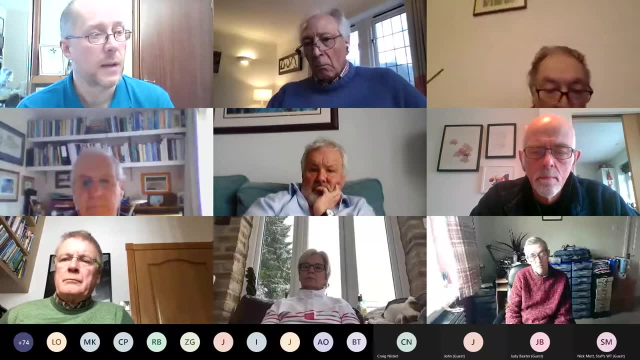 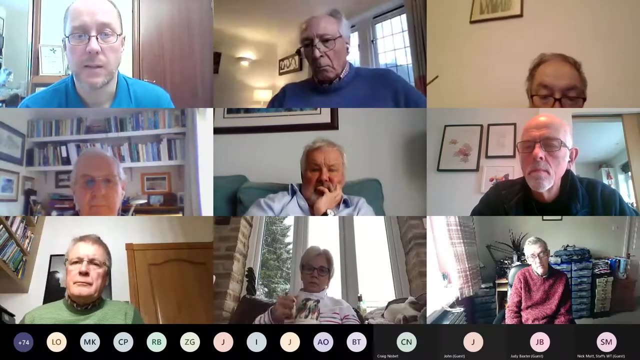 They can move to with on the on that advancing front of warm, warm temperature, And we're seeing that in mayflies as well. So there's a species called Ephemerala notata which is becoming more common in northern areas. I've found it in the River Don, for instance in Aberdeen, and fairly regularly in the River Don. 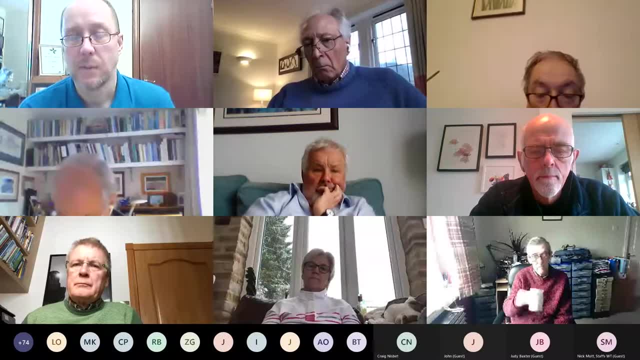 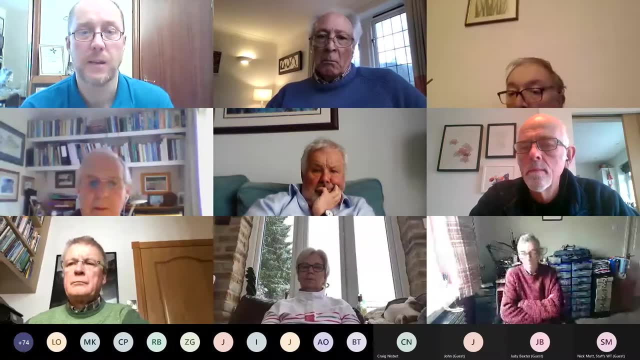 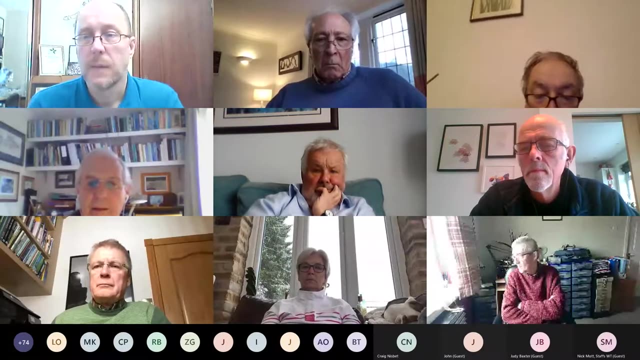 which you know it used to be Occasional but it seems to be. it was first recorded in Scotland, I think in the 70s or 80s, in the River Hendrick, And you know, the fact that it's now further north would suggest that it is moving on the on that climate front. Where are we now? Do the number of instars depend on water temperature and feed, or is it a species specific thing? It's a good question. so It is very much species dependent, but I'm guessing there will be some some variation in the number of instars. 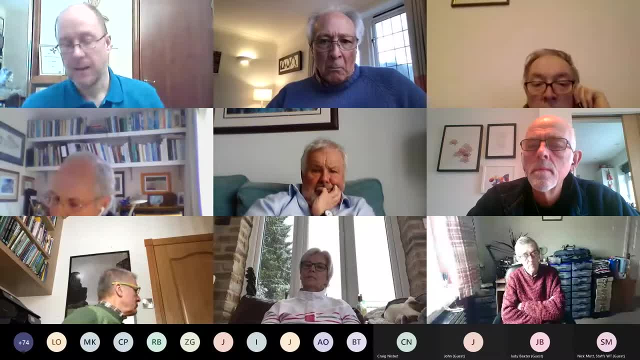 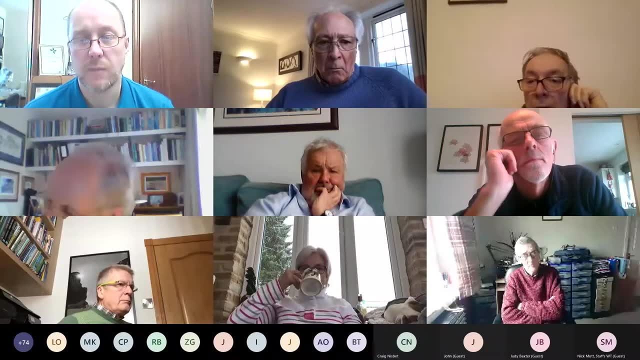 but not not a massive sort of like between 10 and 50,. you know, maybe one or two instars It might. they might emerge earlier, would they? I don't know. Actually, it's a good question Not going to answer that one either. What is the lifespan of females? As you said, the male dies not long after fertilization. the female OK. so. so most of them will go, will fly off from the mating swarm after mating and they will go and find a place to lay eggs. 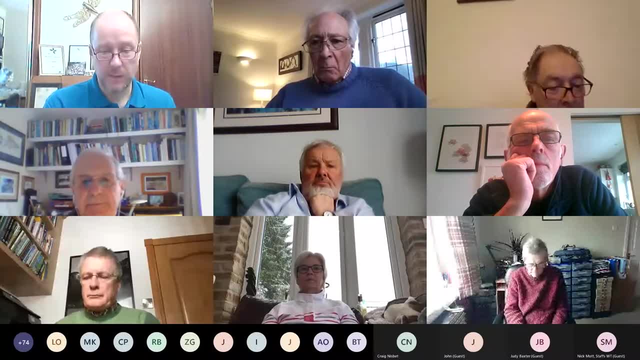 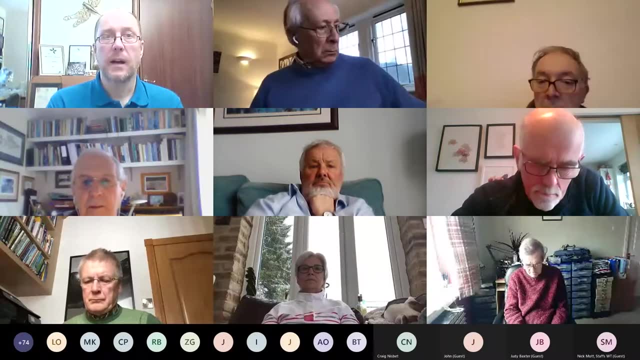 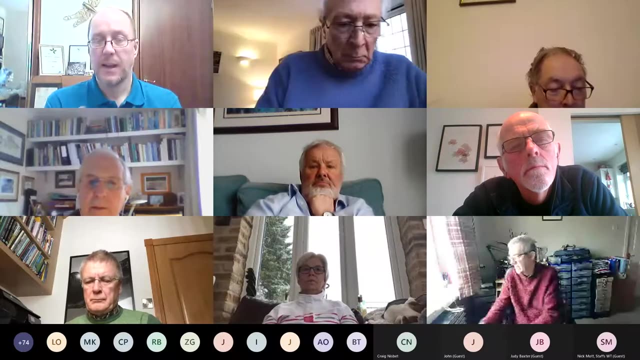 And then that's them that they'll be spent and they'll, they'll, they'll die then. But one particular species, Chloiondipterum, is it. It will actually fly off with with its eggs fertilised and it'll actually gestate them. 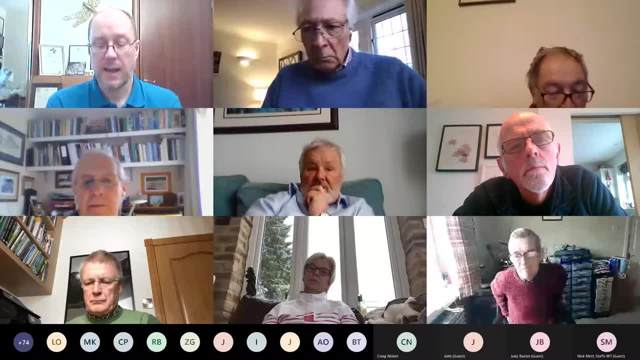 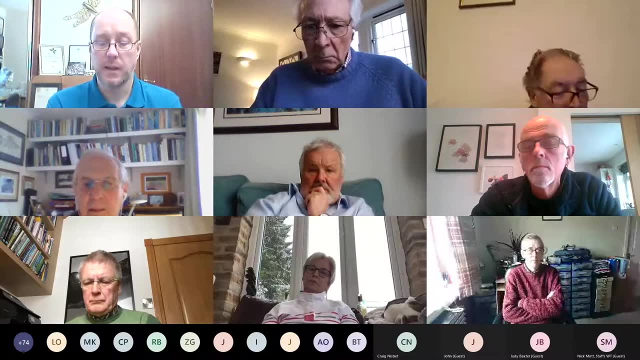 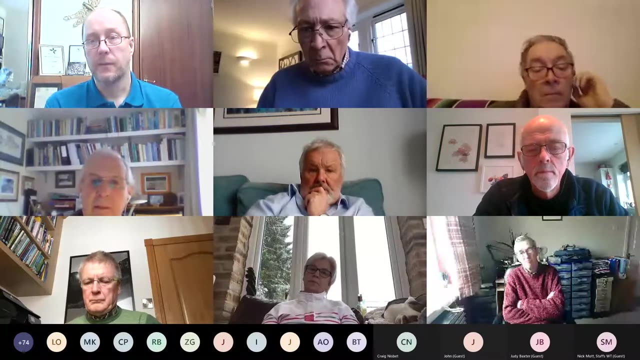 So it it. it keeps those eggs in its body for about a week and then lays its eggs, And when the eggs touch the water they hatch immediately as as as larvae and swim off, So that that one's got a particular particular technique there for for egg laying. 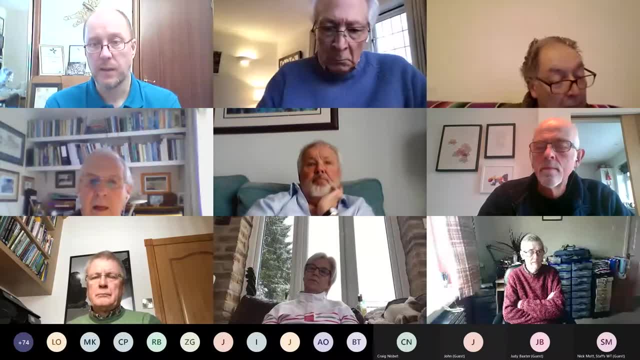 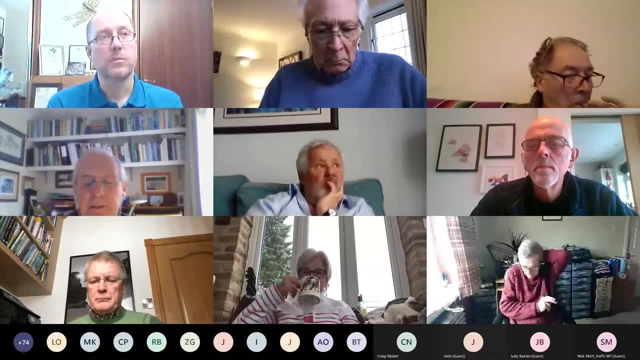 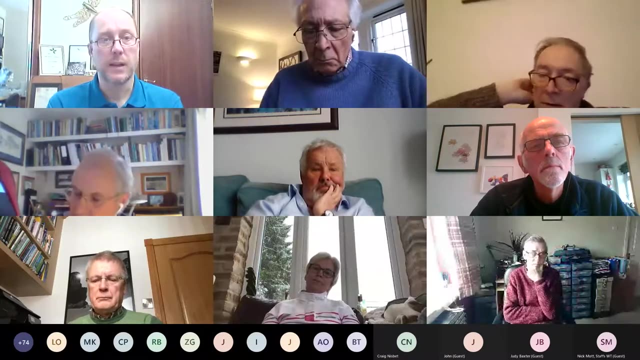 In fact, it doesn't actually lay its eggs, but they're immediately larvied, And that it's actually one of the most successful mayflies in the world. It's colonized, I think, all all continents apart from Antarctica, And that's probably because it can carry these eggs with it. 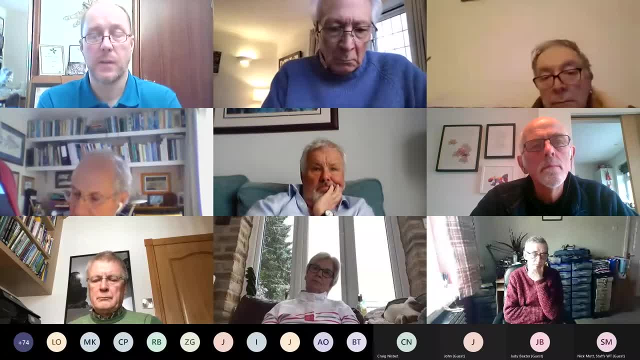 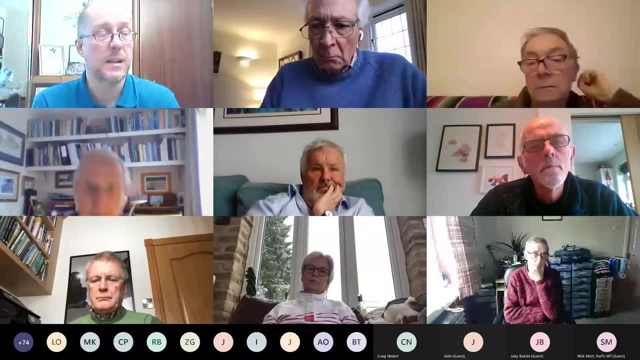 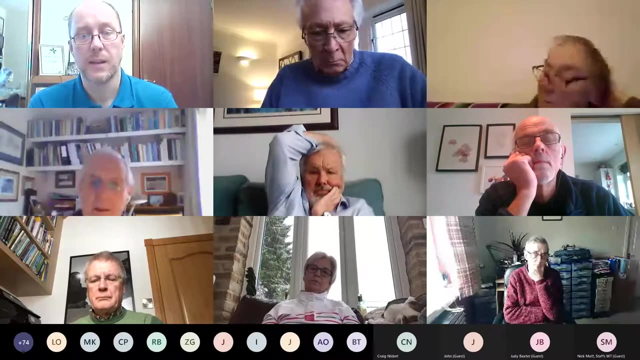 The other thing I didn't see is that some females can develop some. some mayflies can develop without male fertilization, so pathogenetically. So there's about 19, I think 19 species in the UK that can do that out of the 53, which is another way that they can make sure that they continue. 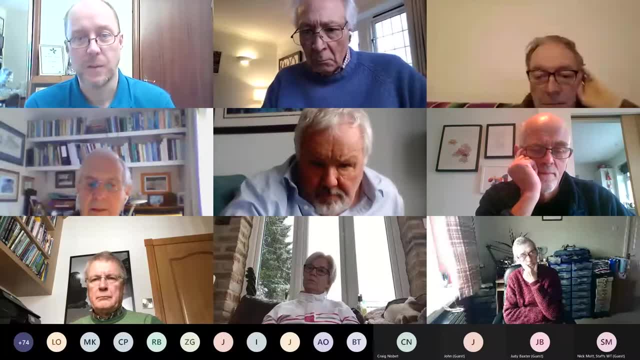 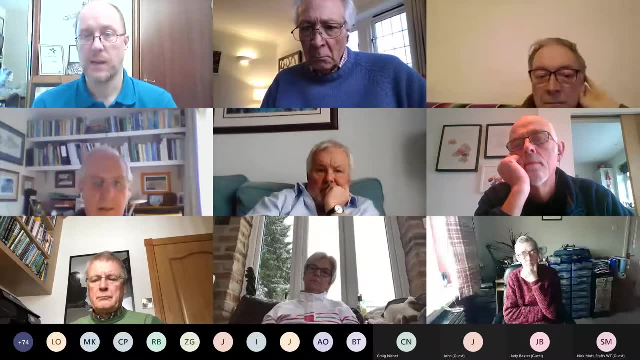 I mean, they've been doing this for 300 million years. You know they're pretty good at this, Kenny. yeah, I think it is a species specific thing, but there will be some variation of that with the map showing species distribution. 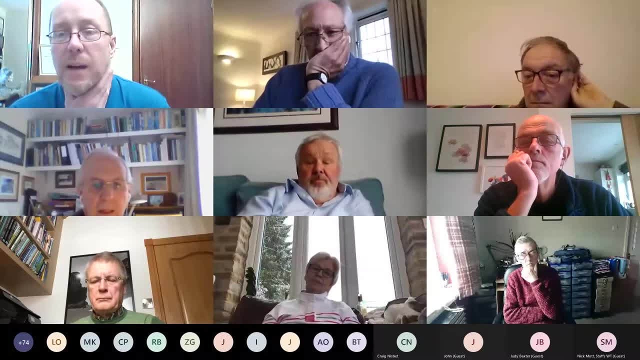 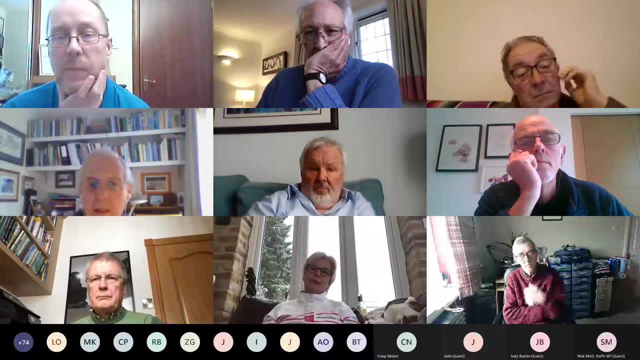 There's no data for Northern Ireland. so they are not there. And if so, why? Or is it a lack of data? And so I run the the mayfly recording scheme, but that only covers Great Britain. It doesn't cover Ireland. 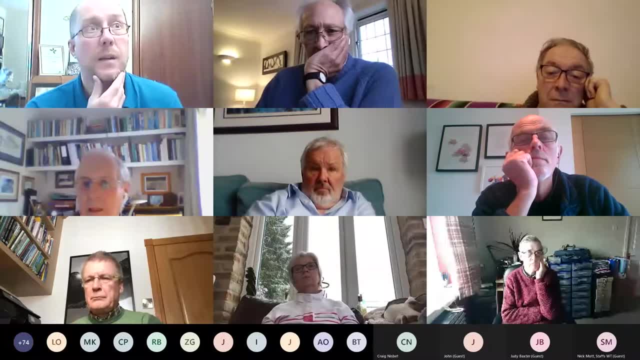 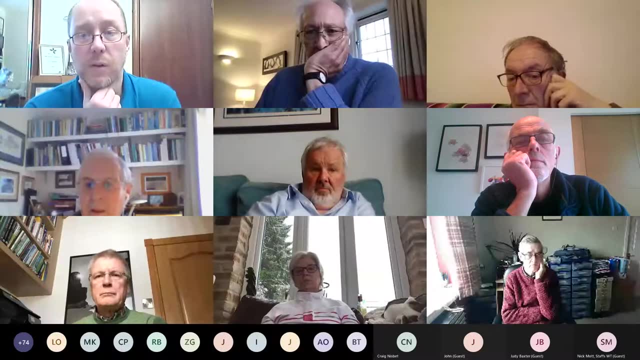 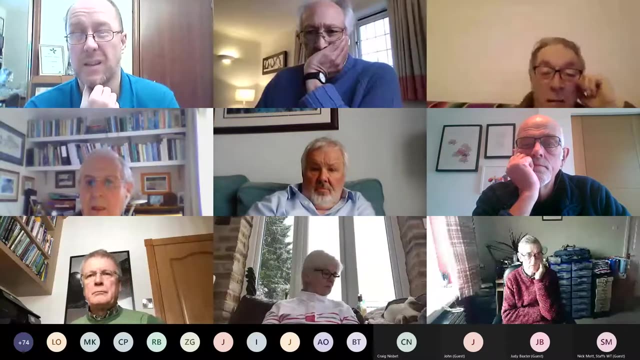 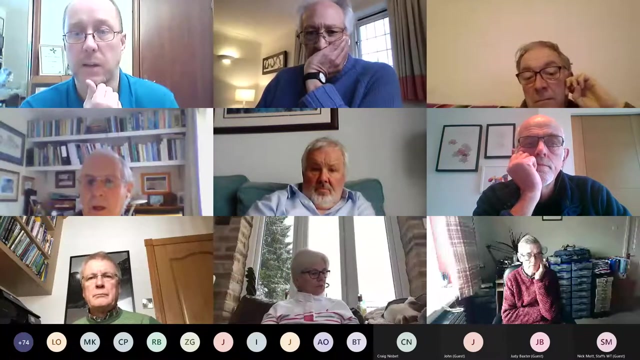 There's. there's the national data, but National Biodiversity Data Center covers Ireland and Cedar in Northern Ireland, So I've not got data. but amelitis is present in Northern Ireland. It's actually endangered there, Classified as endangered Because there's so few populations and it's declining so quickly. 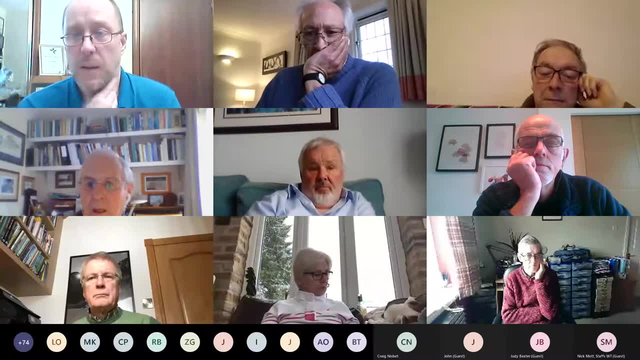 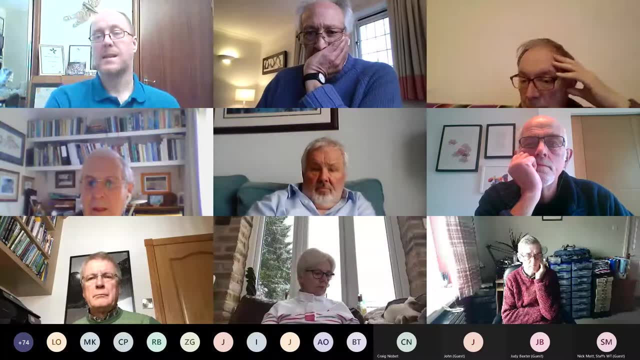 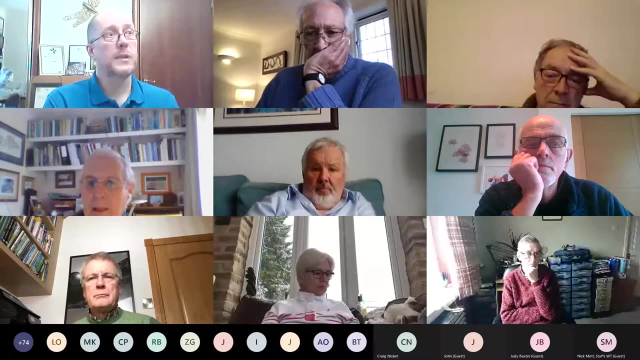 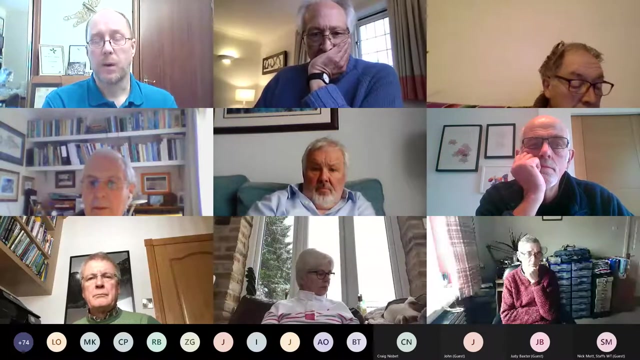 For the same issues. they've not got high enough mountains. How quickly do they adapt to environmental changes like climate change? If you mean by adapt, how quickly are they affected by it? We've seen we're seeing amelitis move upstream fairly quickly, or 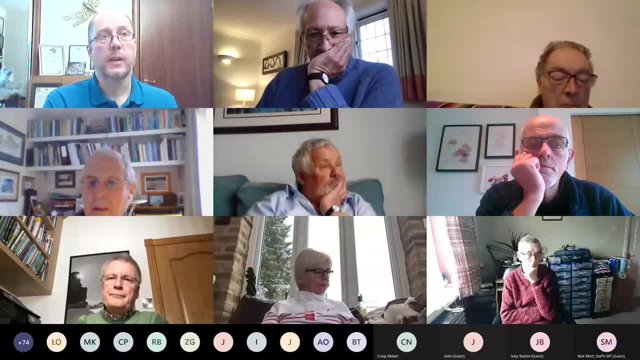 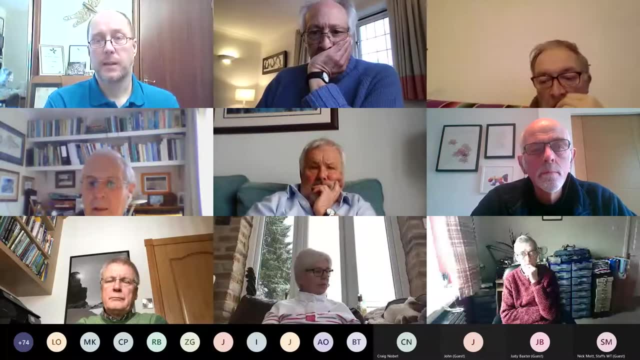 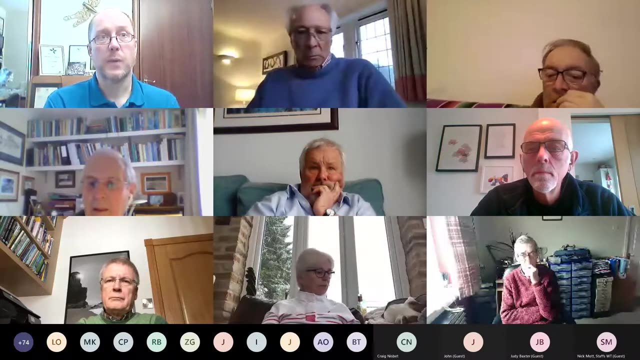 be lost from lower altitudes fairly quickly. So we we did a project where we we surveyed sites where amelitis was present at lower altitudes, and almost all of them. you know, this is maybe 20 years, records from 20 years ago. 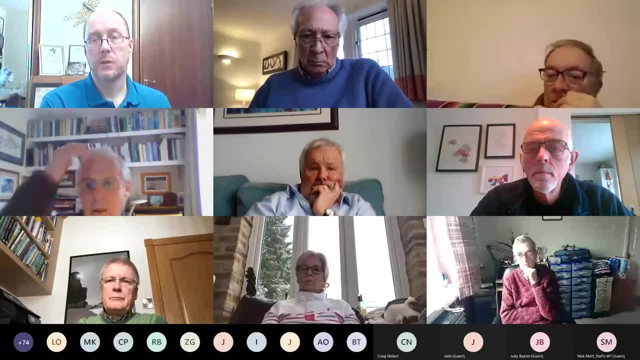 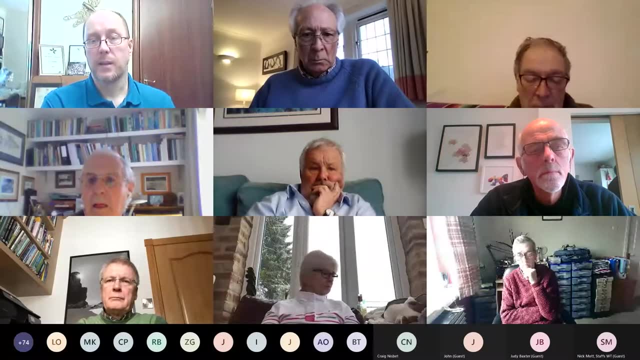 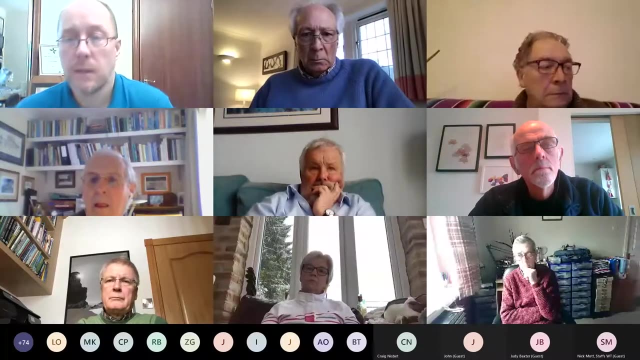 And although almost all of them had lost their amelitis. So, yeah, they do, they do. They are affected by climate change quite quickly And certainly other Environmental changes like pollution can affect them immediately. If you know there's a pollution incident they can be wiped out. 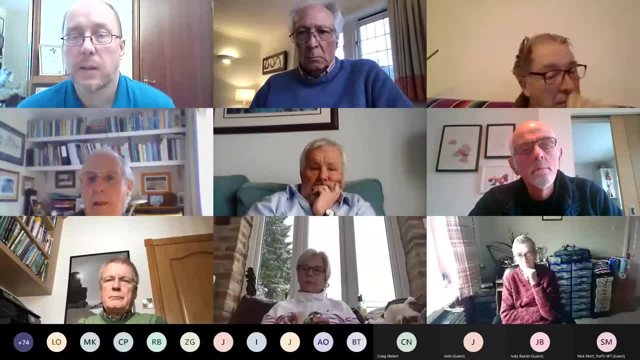 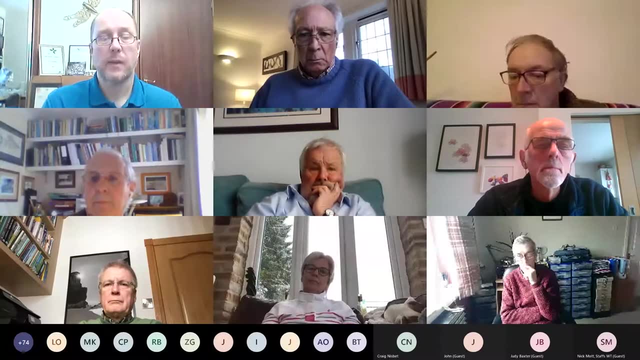 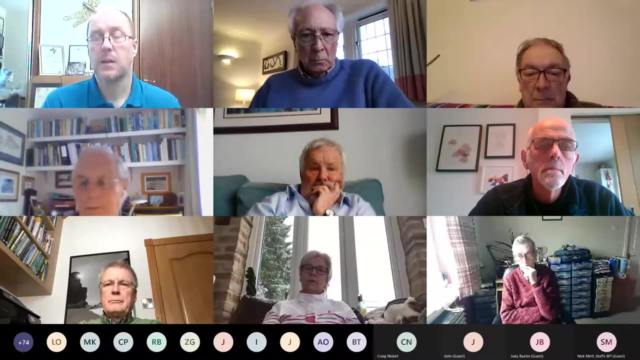 Is the life cycle annual in all mayflies? OK. so in the UK most are have got an annual life cycle, one one year life cycle. Some will have multiple generations in a year, So some of the betas will have up to three generations and the Uh, The larger ones, the ephemera species, typically have a two year life cycle. so they'll, they'll, they'll have two years to develop, and And then in other parts of the world you can have that. I'm racking my brains. I think there's a species that you know is maybe three years, But most are- most are, most are an annual life cycle. There are some species in the world that you know have very quick, quick life cycles as well. What's the evolutionary advantage of having two winged adult phases? 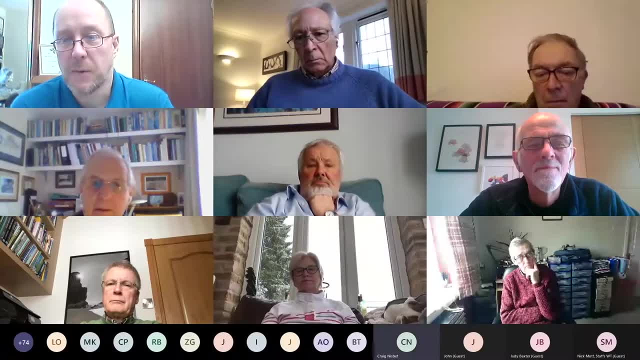 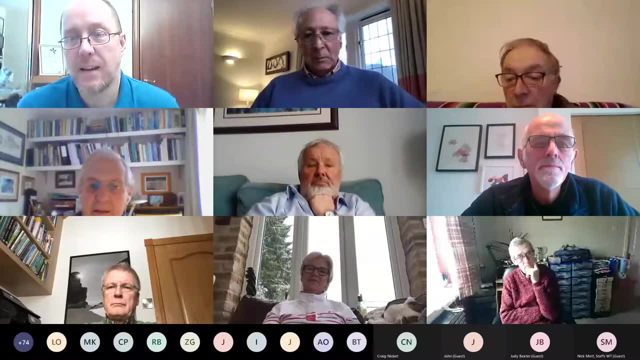 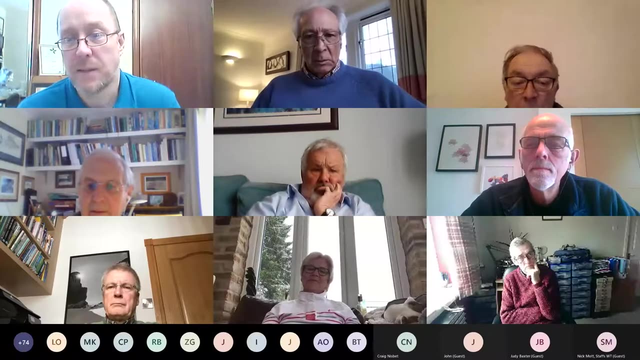 Well, if anybody knows, that would be great. You could let me know. I don't. I there's. there's a lot of debates And there is. it clearly seems to be some sort of hangover. This is, this, is the this. perhaps this is the ancient form. 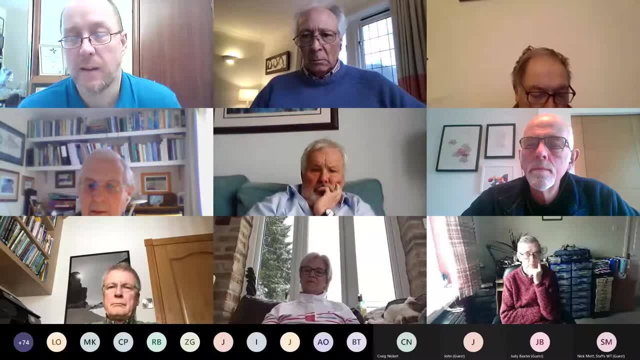 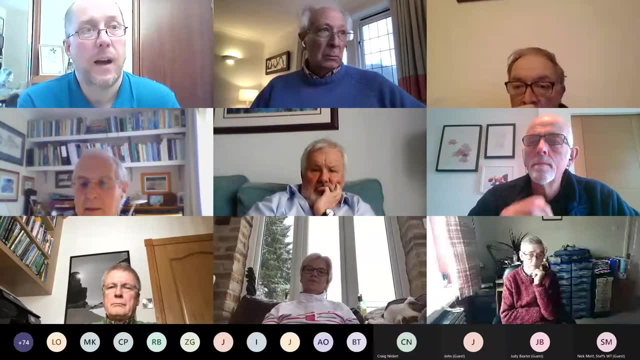 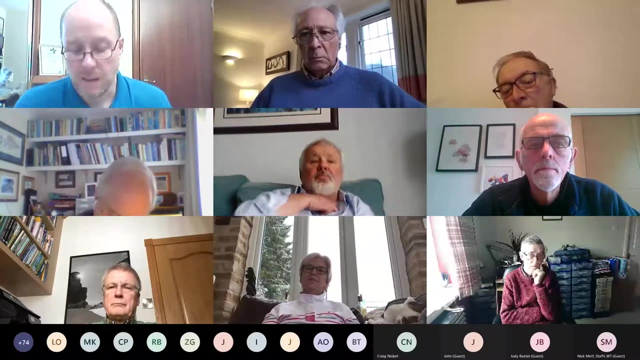 And we know, with them being such a long lineage of of of species, And certainly that does seem to be, as we've mentioned earlier, that there seem to be a lot of development goes on in that extra stage which allows them to. it is perhaps because they can't go from the stage of having 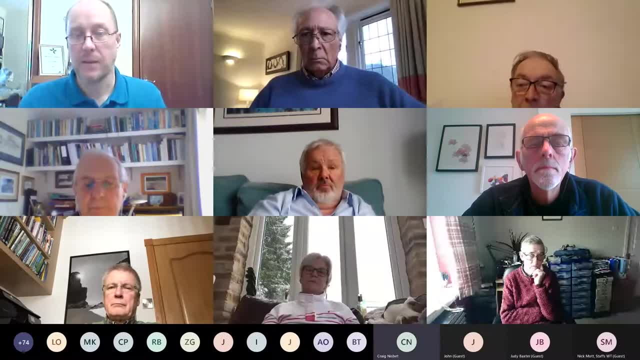 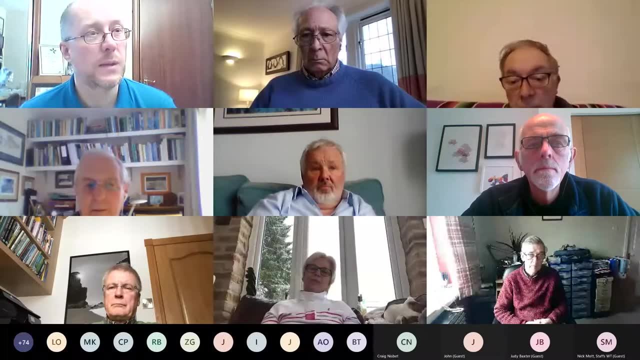 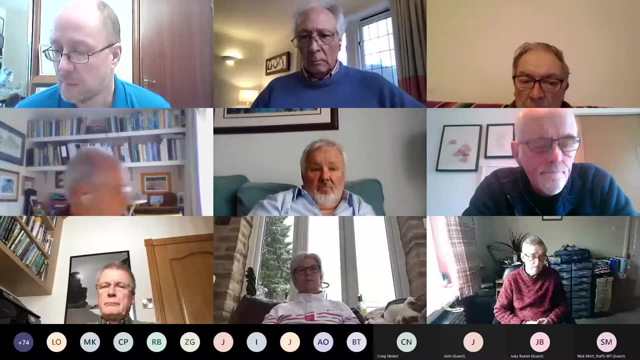 all those features present in the nymph and then come out as a fully formed adult, And some. I think there is one, one or two species that are almost forgotten that stage in the. I'm trying to think there is a species that's forgotten that stage. 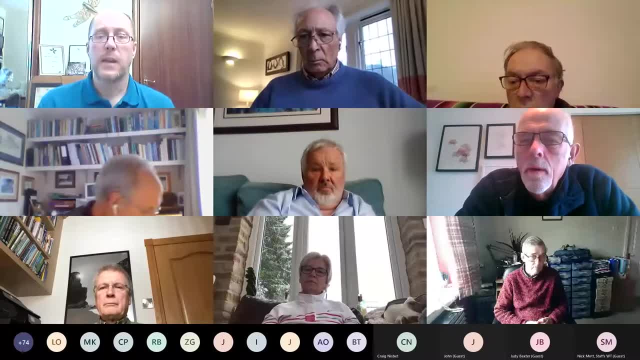 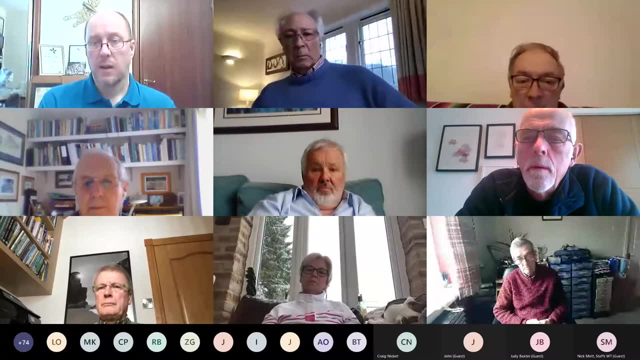 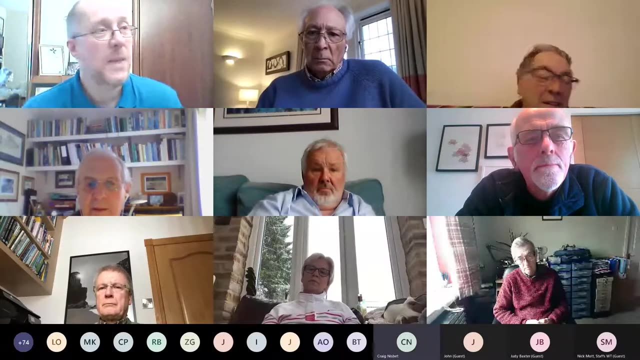 and doesn't and just comes out and just gets on with it and the But it is probably to do with morphological change. What is the definition of a mayfly? Oh right, I should have said this at the start, so I may. 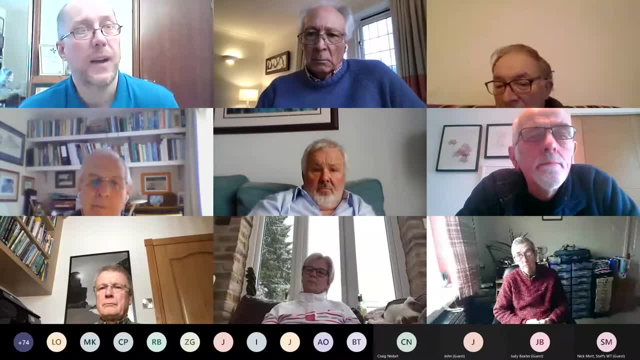 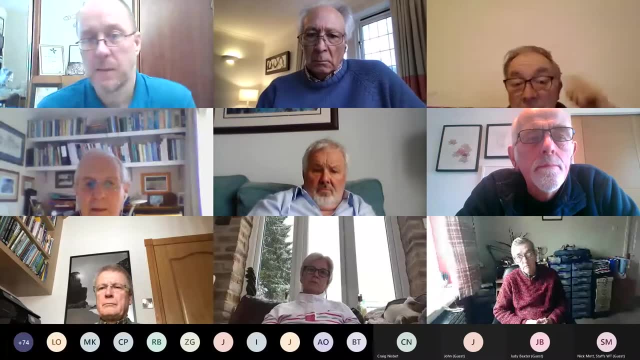 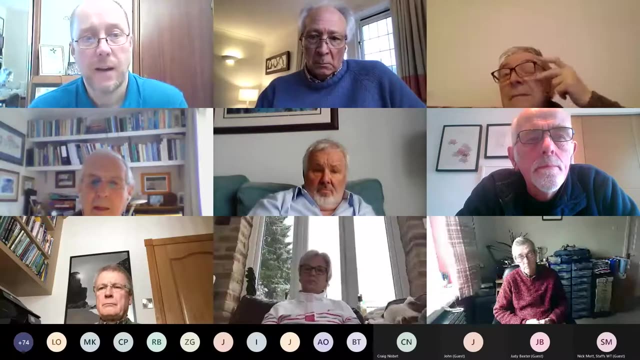 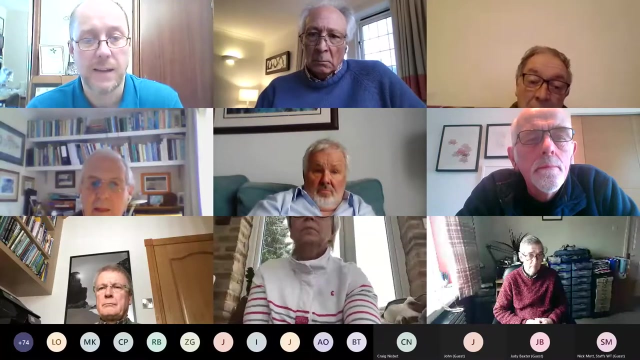 Mayfly Is different, are different things to different people. so the word mayfly is used as we saw. Eaton used it to describe all ephemeroptera and In the south of England mayfly is the three ephemeridae species, ephemera species, so ephemeridanica, lineata and vulgata. 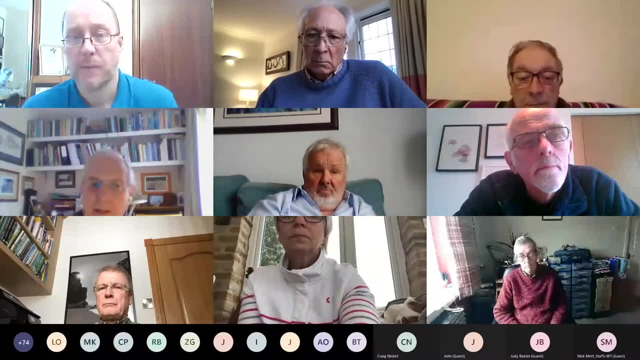 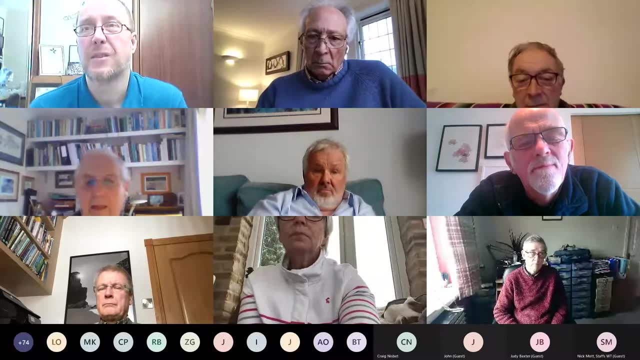 In again. in a lot of areas they'll call the rest of them upwing flies, which I think is a bit clumsy and pretty, pretty not very nice, you know, not not doesn't fit them really. They used to be called dayflies because 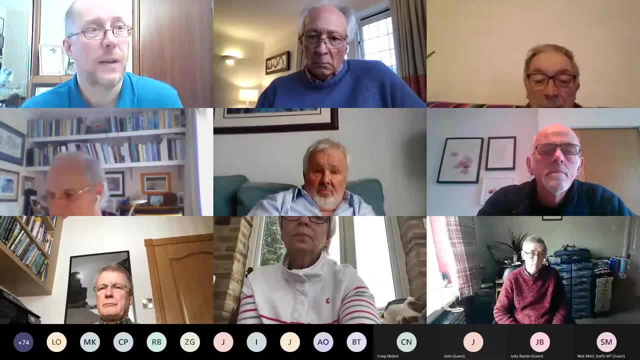 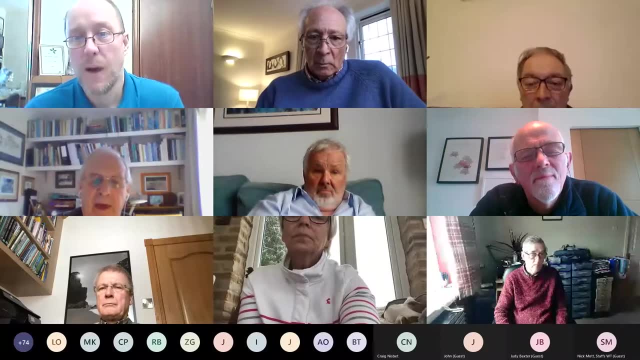 of the short life cycle or the short adult life cycle. And if you- if you- to talk about a mayfly up in Caithness, they would be talking about a stonefly. so that's kind of why we we tend to use the, the Latin or the. 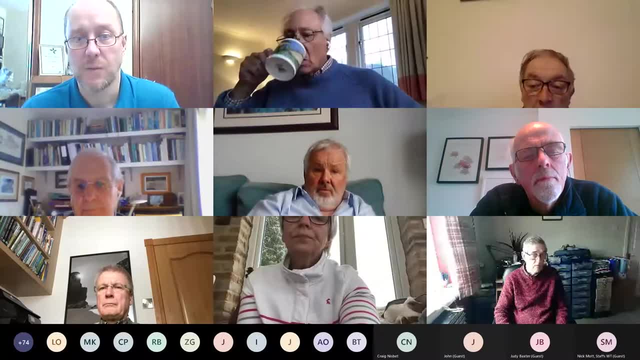 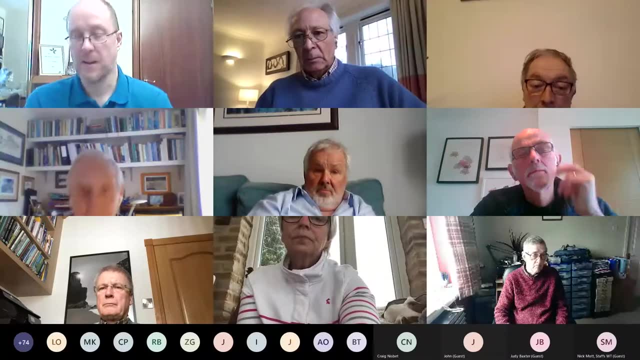 the scientific name ephemeroptera, when we're trying to make sure we what we're talking about. it's a good question and it's one that causes lots of arguments in a pub, if we ever get to go to a pub again And are the size of local population cyclic. And if so, what periods? And Possibly sometimes some species do go in a sort of like boom and bust. There's a lot. there's a lot in that question. It can depend a lot on environmental conditions, It can depend on on in rivers. It can depend on water quality and it can depend on on on temperature. We have got a The North Atlantic Oscillation has been shown to affect populations of of various freshwater invertebrates And and certainly I've seen presentations on on fish that shows a seven year cycle. 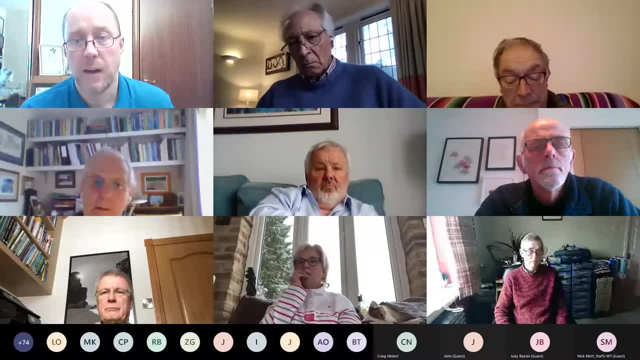 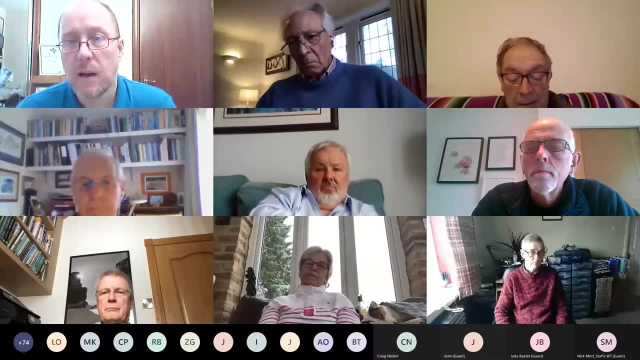 in population size and or in catches at least. And so, yeah, there is probably something that I wouldn't. I wouldn't like to see what the period is on that And I'm not sure what. No, I'm not sure what. I'm not sure what. 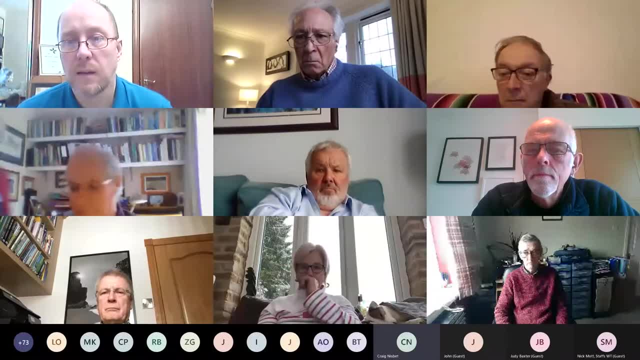 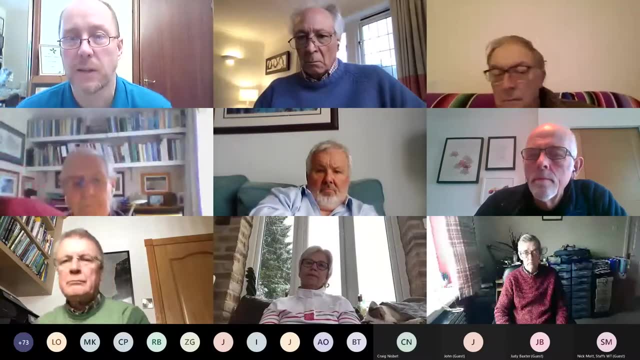 Adrian is referring to and Southern is at present. Maybe she can elaborate. I think. I think it's. I think you answered the question. There's no amelitis in Northern Ireland, It's in the Republic. so Southern Ireland, Yeah, very good. 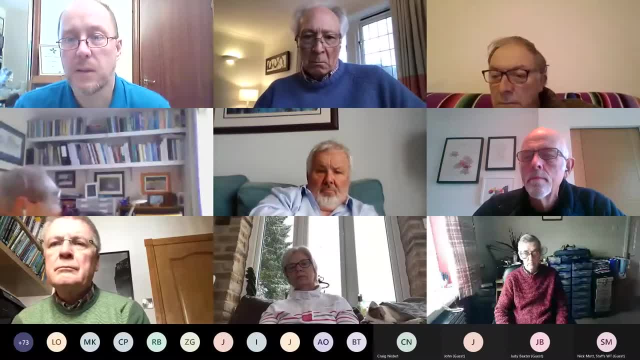 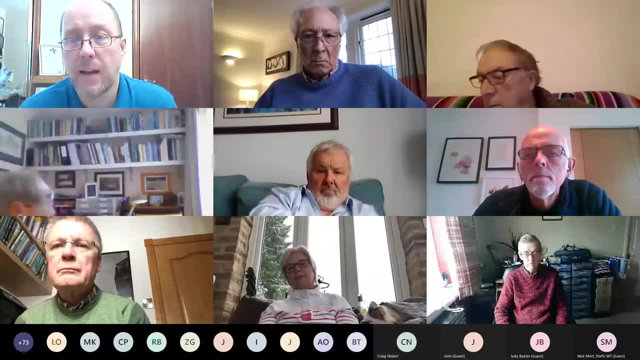 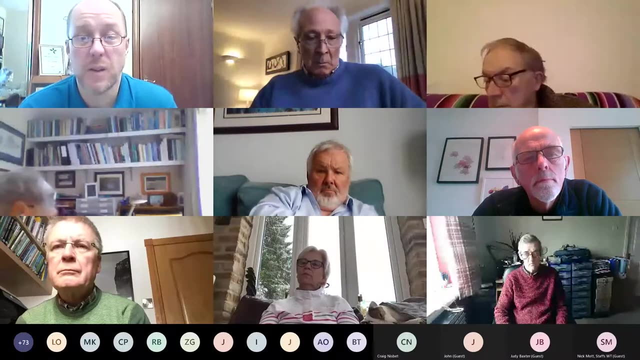 And I remember Danica- can the development to the Imago stage be actively delayed or postponed? No Well, I think Ken Whelan in Ireland has has a paper which showed that they emerge anyway, and they emerged in a really bad Summer storm. One year and that the and their reproductive success was really poor and that you can still- you can probably still- see the impact of that poor emergence in the population structure just now, because they're a two year. You can see that the difference between them if they were a one year life cycle. 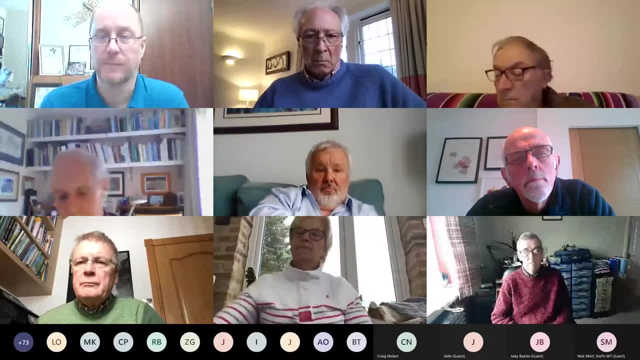 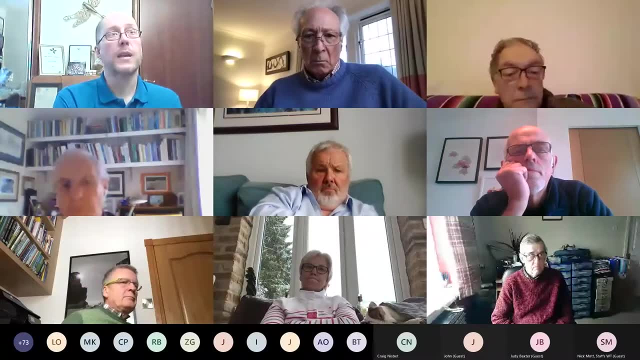 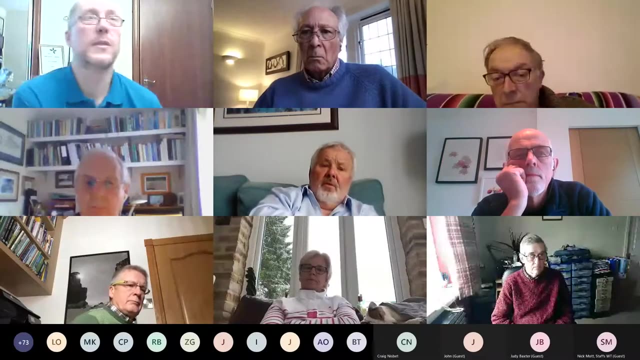 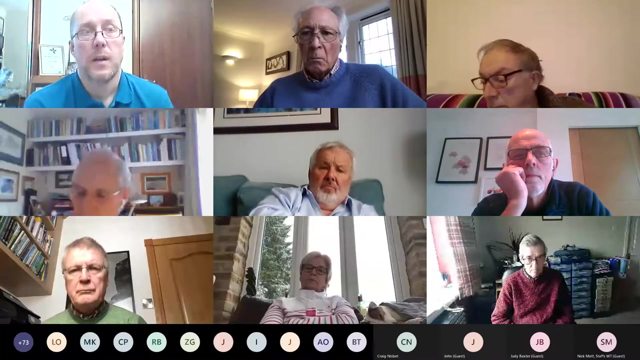 they would. you know, if they emerge at the wrong time, that's it gone. What factor triggers nymphs to hatch? and So the preceding weather. So temperature is one thing, So the two different approaches, So the early season hatches emerges will. 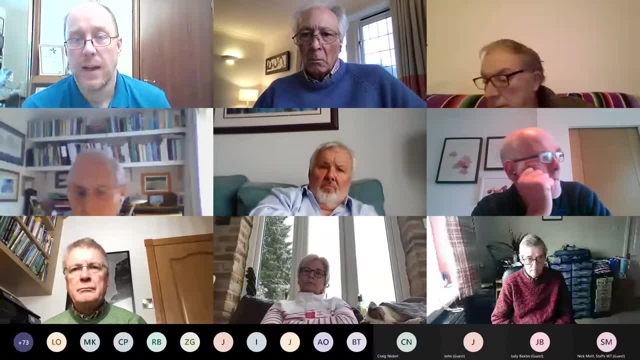 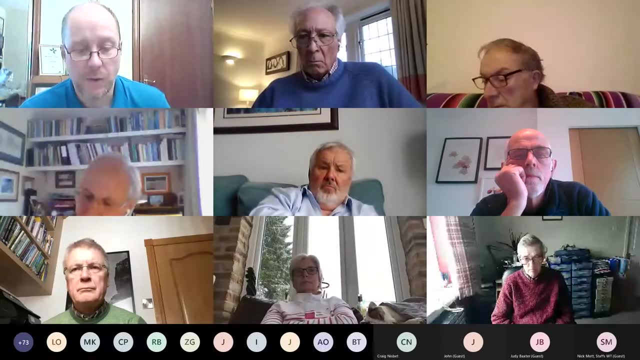 It's pretty much on the length, And so you'll find the hatching at the Same time all year round, because they're not really bothered about temperature if it's early season. So Ruthergina, Germanica, on different rivers, has a day when you can pretty much 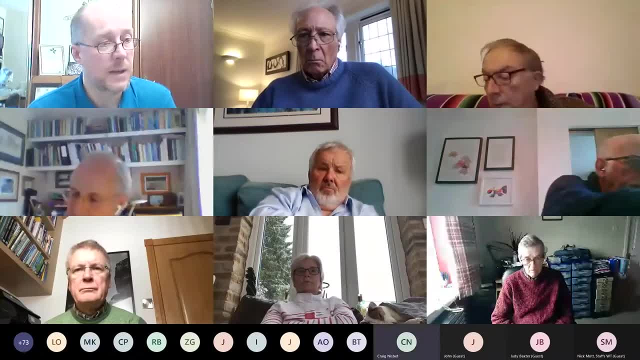 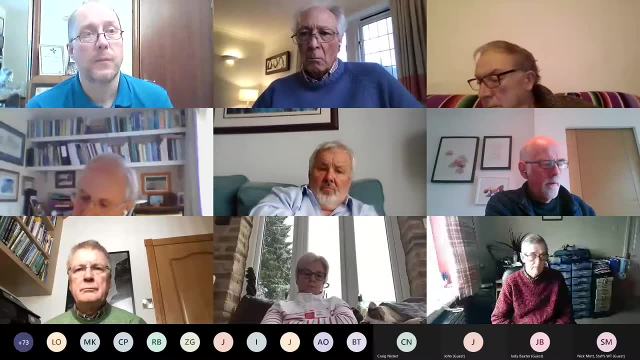 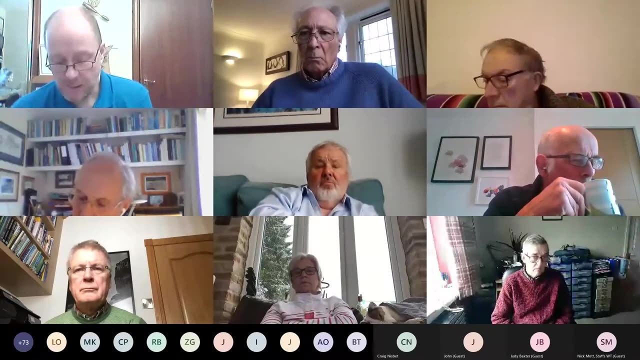 expect the hatch to start. I think the the river Tweed is about April the 15th, The from memory. But the other type of trigger is that's on temperature and and on the actual day. it can be do, it can be to do with. 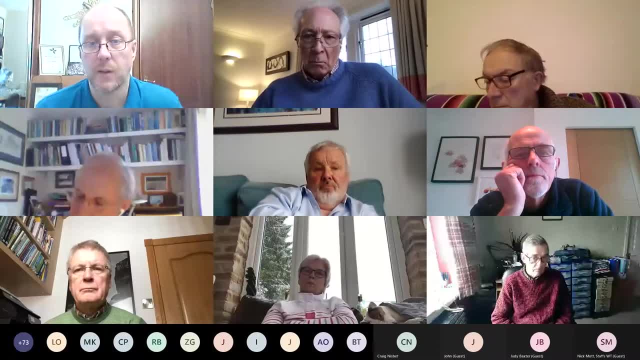 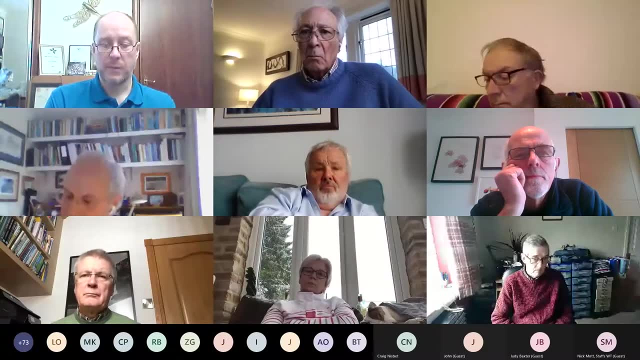 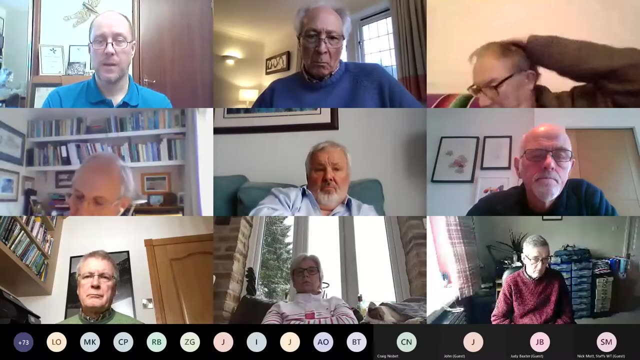 Brightness, and so they're looking for good weather and, depending on what the temperature has been in the day before and what the temperature is on the day, that can determine what time of day they actually emerge, whether, if it's been a very warm day before and a warm evening, you might find them hatching earlier in the morning. 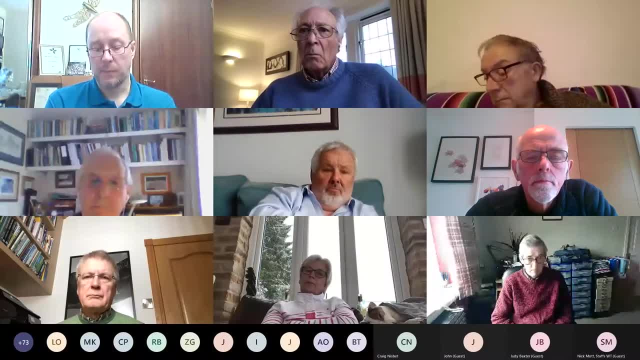 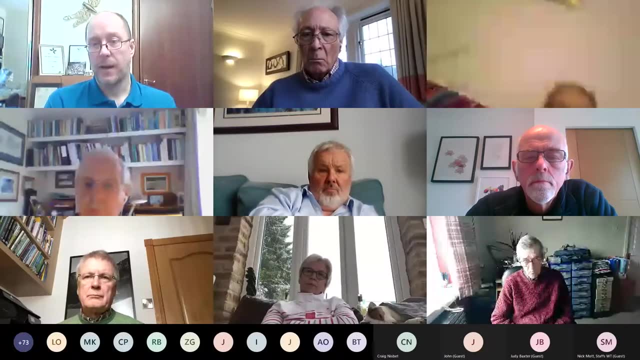 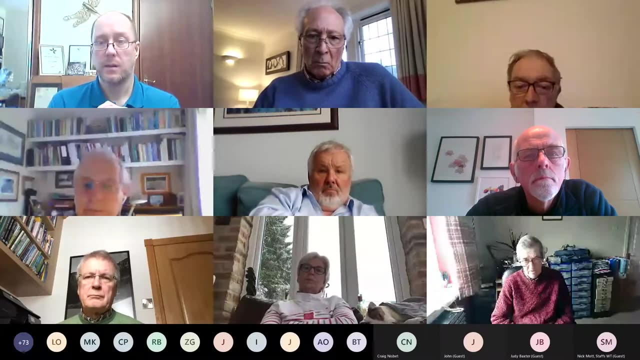 in the morning, whereas if it's been a cooler evening they might Hatch later in the day. So there's a the subtle sort of differences in the triggers, but the main ones are either day length or temperature. I think that's it. 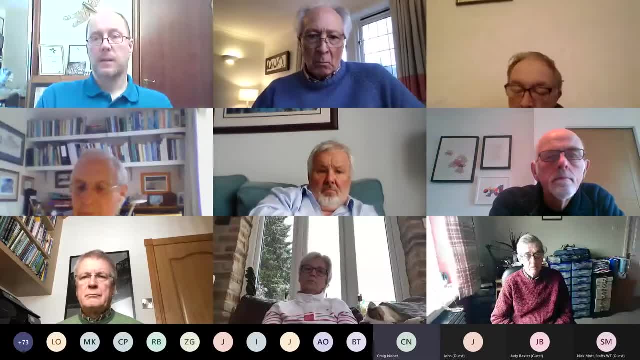 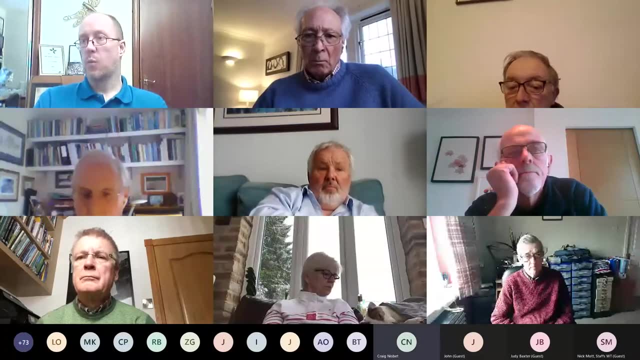 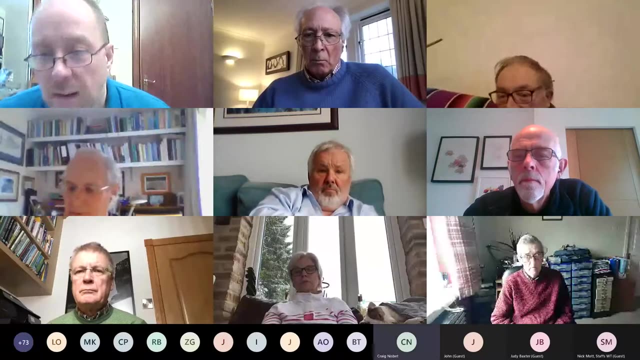 Yeah, I think that's it. He was just making a point about the amelitis. Yeah, in Ireland. Yeah, OK, well, what I'll do now Is I'll move on to the identification. Oh, last minute question. 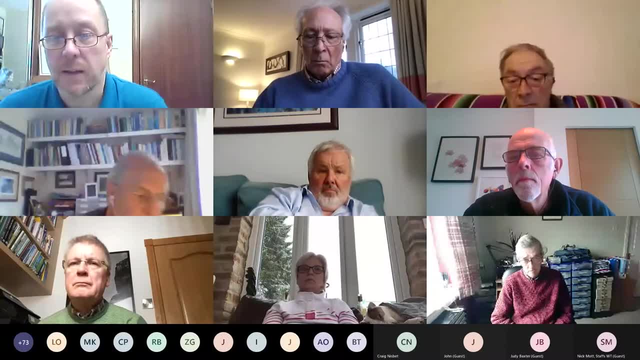 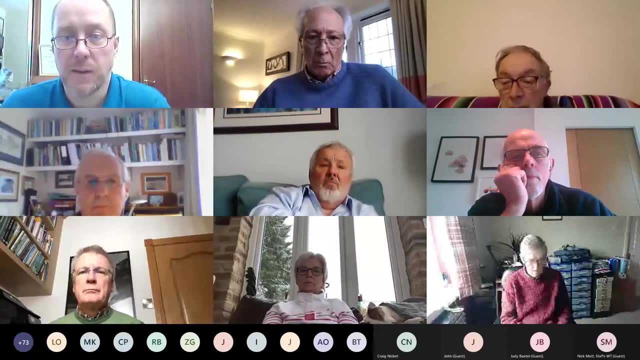 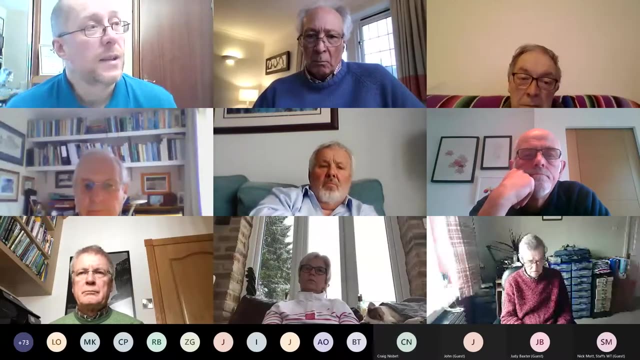 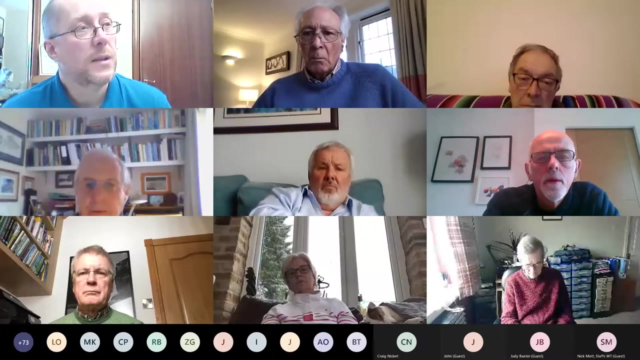 Can increase shade from repairing plant and then affect hatching and possibly, but at least they're still there to be able to hatch. I suppose I think there are some. there are some species. It's interesting that there are species that the heptagenosulphuria anecdotally 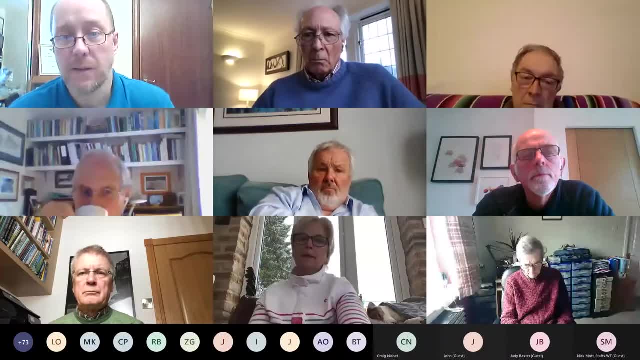 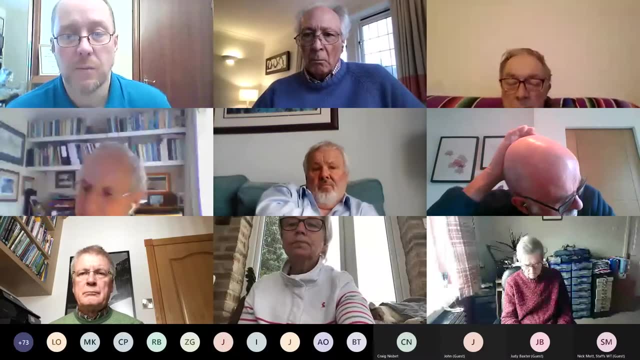 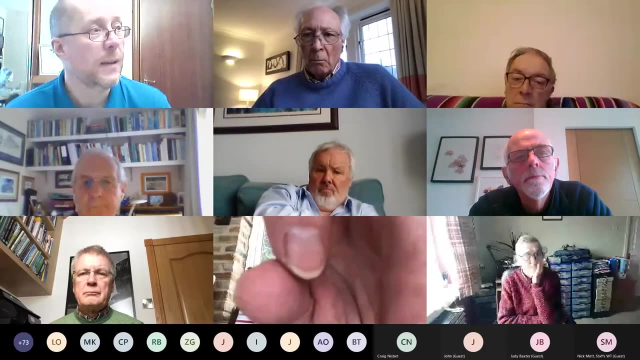 they don't like hatching where there's any shade, and they'll hatch into direct sunlight, and then they'll fly straight up to the top of the trees, So potentially, there's an impact there. I think the key with riparian planting, though, is that we shouldn't be making 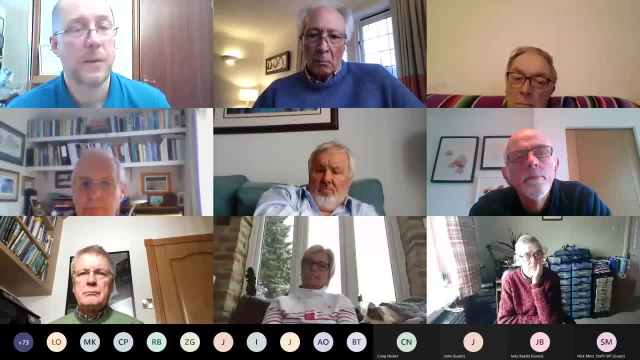 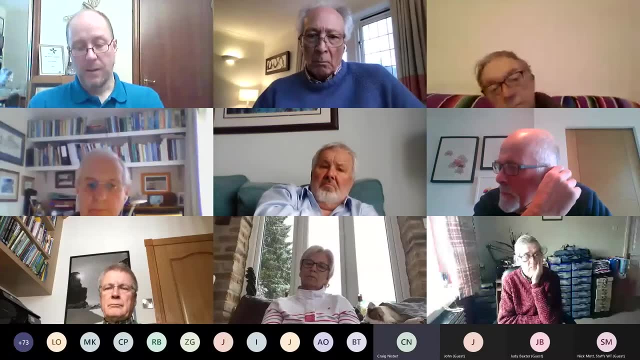 dark corridors. you know it is all about dappled light, It's about little patches here and there and that you know it's not about covering the whole of the the banks in trees, because some species do need some sunlight in there.